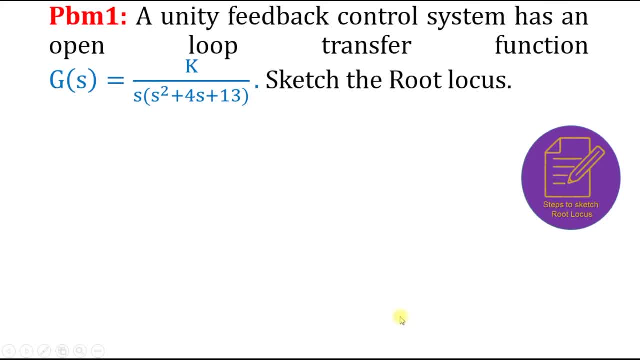 I welcome you all. In this video we are going to solve one problem related with root locus concept. You can see the problem statement here, Problem 1.. A unity feedback control system has an open loop transfer function. g of s equal to k divided by s into s squared plus 4s plus 13.. 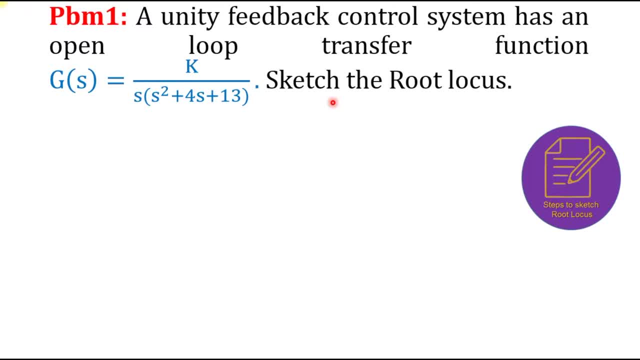 Step 1. Sketch the root locus. Before going to solve the problem, we should know what are the steps to be followed to sketch the root locus. The first step is locating the poles and zeros. Step 2 is finding the root locus on the real axis. 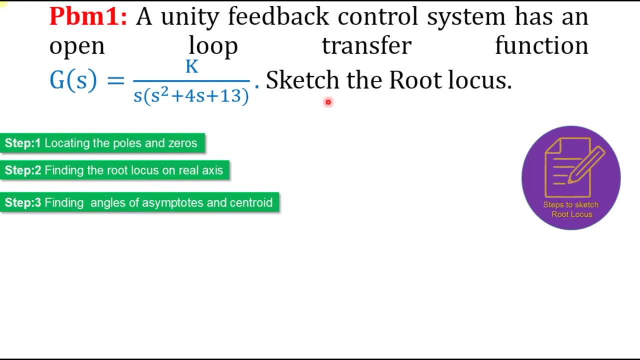 Step 3 is finding the angles of asymptotes and centroid. Step 4 is finding the breakaway point or break-in point. Step 5 is finding the break-in point or break-in point. Step 6 is finding the crossing point on imaginary axis. 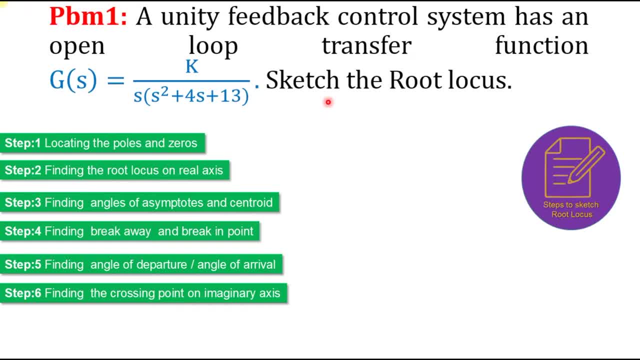 These are all the steps we need to follow to sketch the root locus of the given system. We know that root locus is a graphical method In order to find out the closed loop poles. in order to meet out the stability, we need the exact closed loop poles. 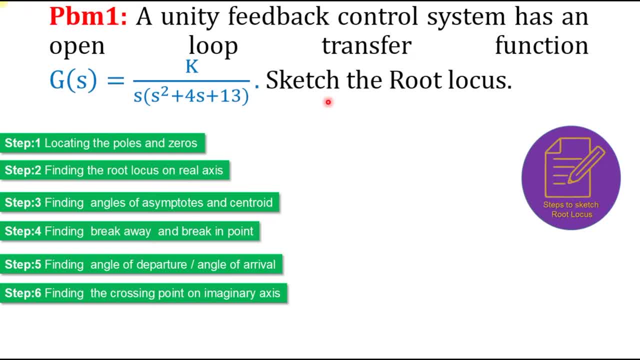 When we want to fix the closed loop poles to meet out the stability, you can use this technique. This is a graphical technique where we are going to use the open loop poles. From the open loop poles and zeros information, we are going to find out the location of the closed loop poles. 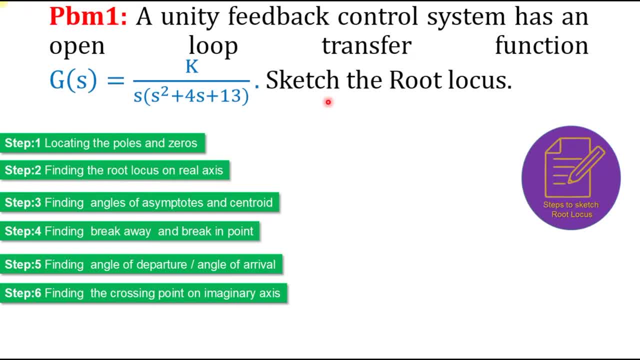 So by various values of open loop gains and some other parameters like damping ratio, we can able to trace the open loop poles So we can get the right location for the closed locus, the locations of closed loop poles. Our objective is to meet out the stability The system should. 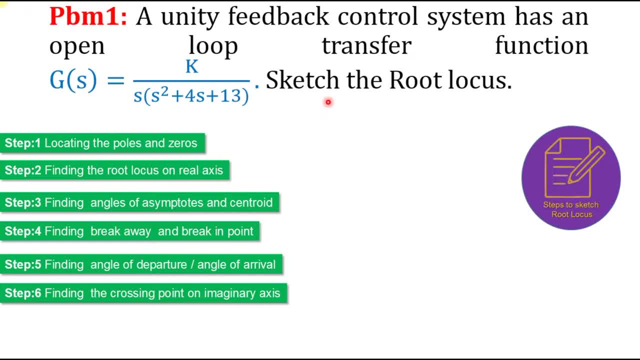 meet out the stability for the various values of gain and various values of damping ratio, We can able to calculate the closed loop poles, locations and, with the information of open loop poles and zeros, Let me solve this problem. So our step 1 is finding the open loop. sorry, 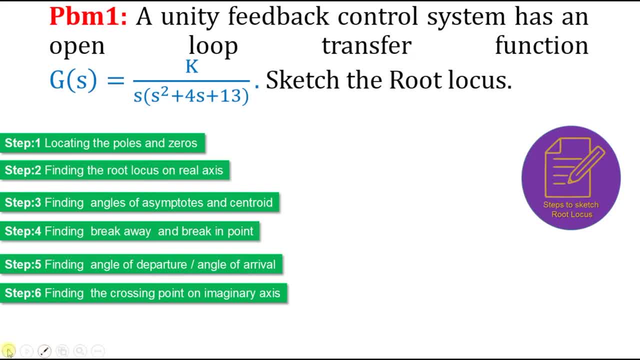 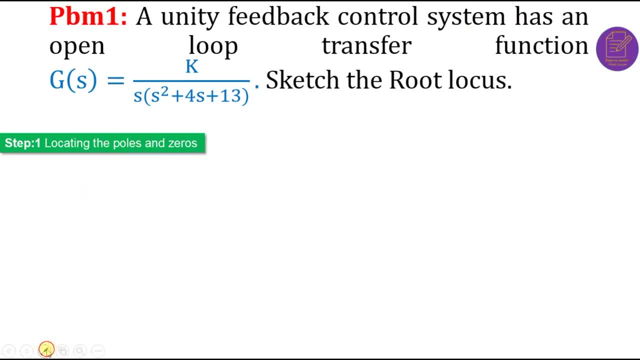 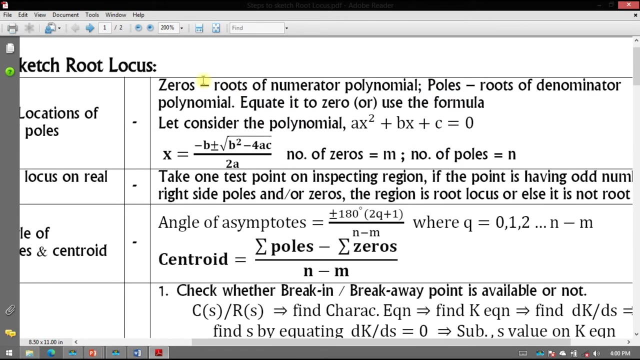 locating the open loop poles and zeros. Step 1, locating the poles and zeros. We can refer this rule book in order to do some analysis about this step specifically. So step 1 is finding the root location of zeros and poles. Zeros: we know that the roots of numerator 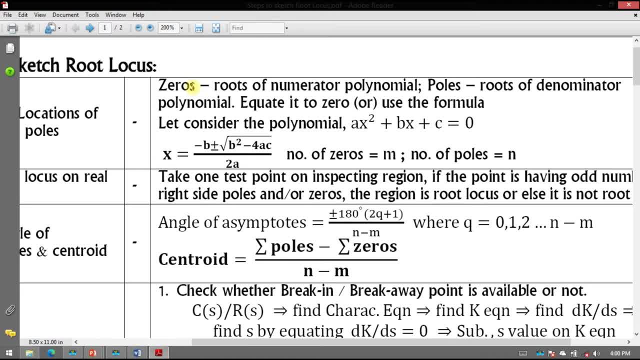 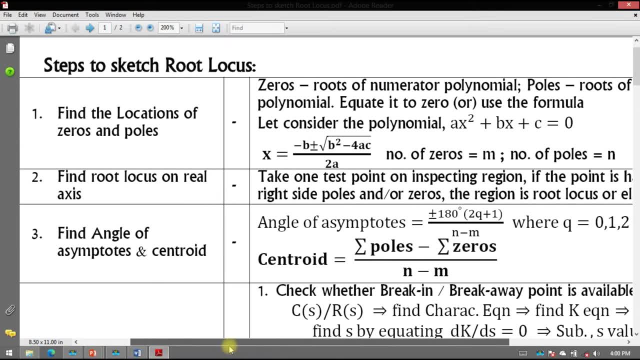 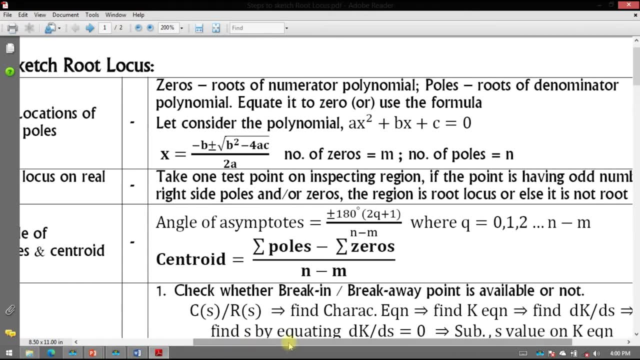 polynomial Poles are the nothing but roots, Roots of the denominator polynomial. So if you want to find out the roots of these polynomials- I mean numerator and denominator polynomial- we can get the values of zeros and poles of the given system. So we need to find out the root means, Let's say your. 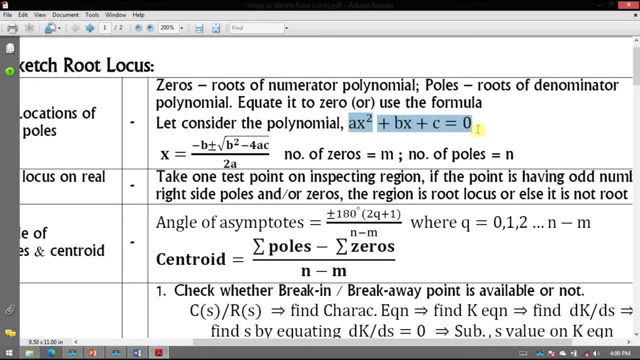 equation is: you are having the equation like this: A x square plus b x plus c equal to zero. Let us assume this is the second order equation You can use. this formula X is equal to minus b, plus or minus root of b square minus 4 e c divided by 2. a Where number of 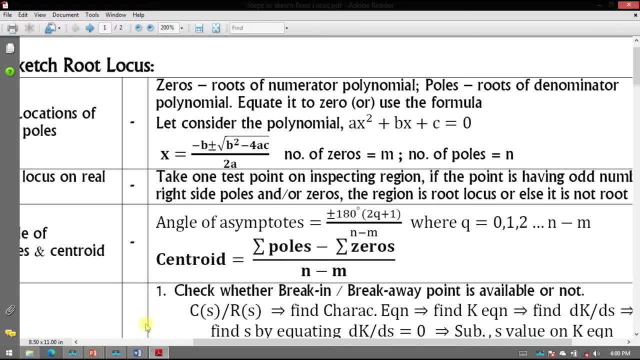 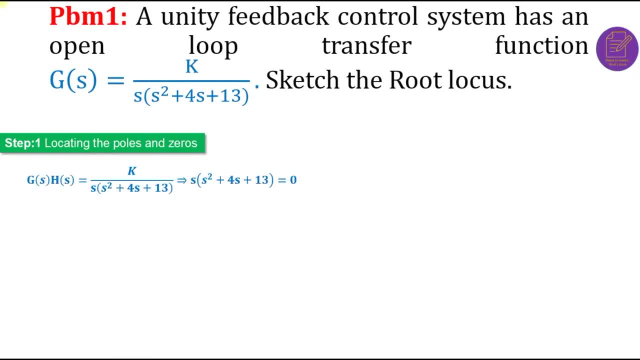 zeros are called as m, number of poles are called as n. Let me solve the step 1.. So we know that we are going to solve the root locus problem only with the information of open loop poles and zeros. So in this system itself you can see there is no zeros are available. 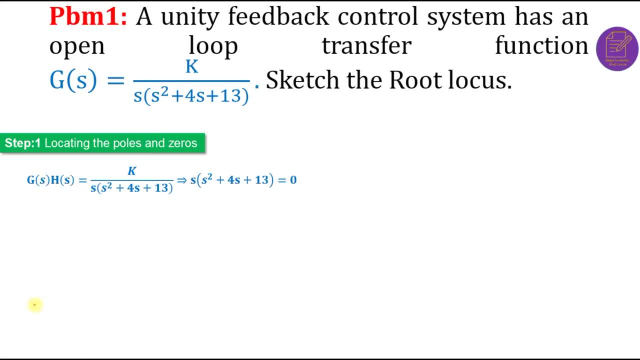 See, this is k, k, this is nothing but the gain value. So we can consider this whole equation as k into 1, by s, into s square, plus 4s plus 13.. There is only one zero. Sorry, there is. only poles are available in this system. So s I mean numerator itself, we 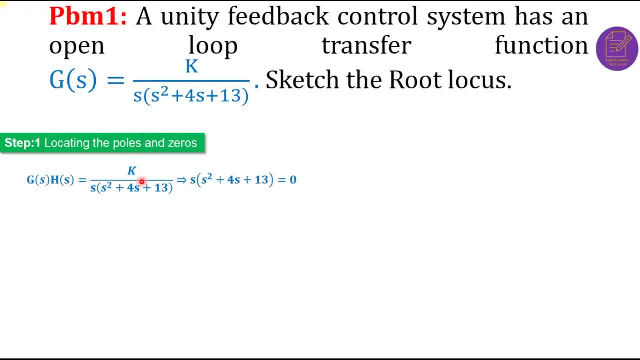 are not having any s term, So that only we are telling like that. So the denominator term s into s square plus 4s plus 13, equal to 0. So we can consider this whole equation as 0.. So one solution is s equal to 0.. So this s we can able to say that one solution. 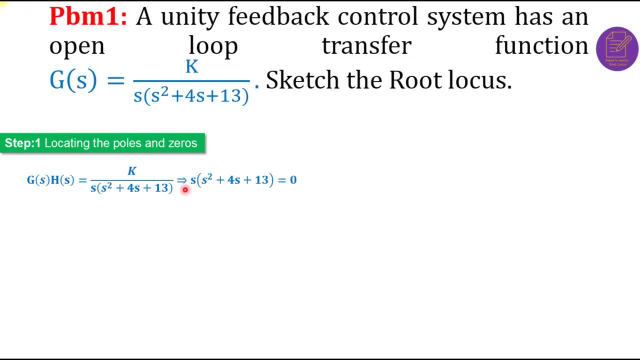 of s is equal to one value of s is equal to 0 and another two s solutions we need. This is in third order system, right? So one value of s is 0. Another two values we require. Okay, So we can use the formula whatever we refer from this, that PDF file, So minus. 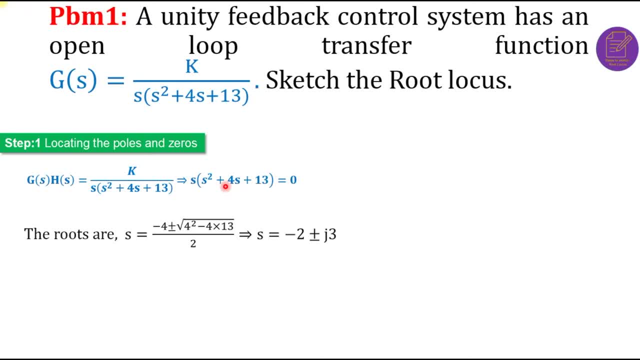 b plus or minus, root of b square minus 4. a, c divided by 2 into a. So here the value of a is 1.. Okay, You can able to understand, Okay, Okay, From this equation I can say that a equal to 1.. Okay, Sorry, So I can say that a equal to 1, b equal. 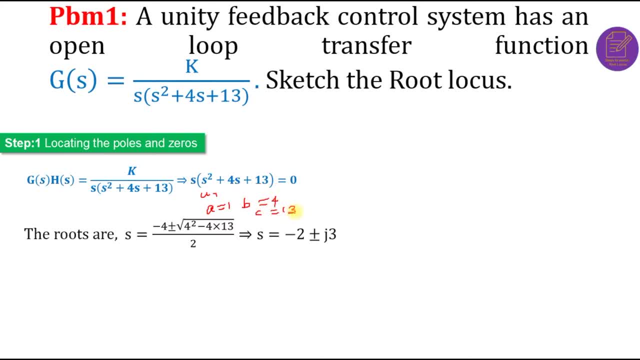 to 4 and c equal to 13.. Okay, Let's substitute the value of a, b, c in this. in that formula We can get the s value, which is equal to minus 2, plus or minus j, 3.. Okay, This is the. 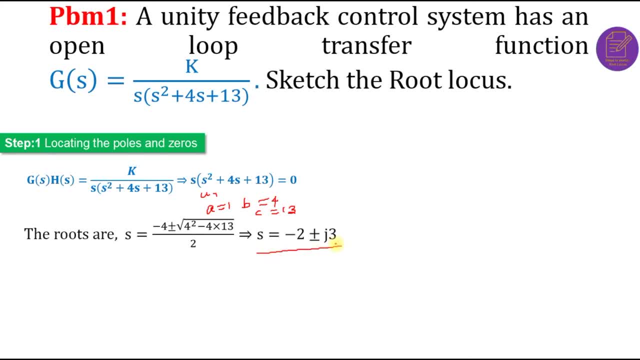 s value we are getting from this formula. Okay, And then we can say that these are all the poles of the open loop system: 0, minus 2 plus j 3 and minus 2 minus j 3.. Okay, So we can say that p naught sorry. p 1 equal to 0, p 2 equal to minus 2 plus j 3, p 3 equal. 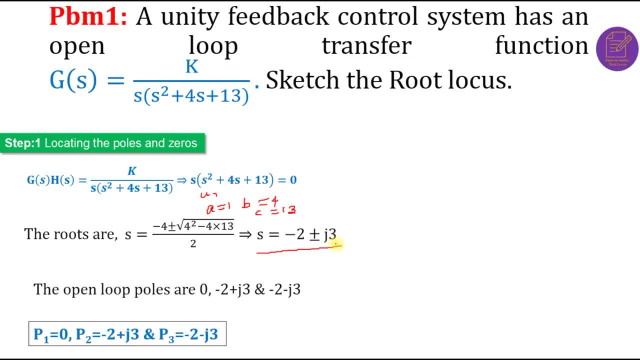 to minus 2 minus j, 3.. Okay, We can locate the pole like this. Okay, Consider this is a s plane. In, in, in, in your x axis. this is a s plane. Okay, So we can locate the pole. 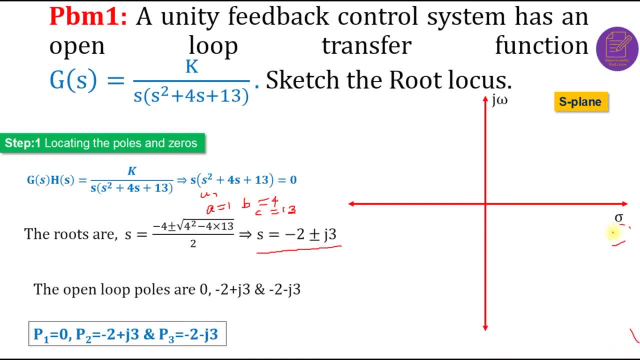 like this: This is a. this is a real real, this is, this is simply real axis. Okay, And this is a. y axis, j, omega axis. Okay, Take the lesser point. Yeah, Let me locate the pole. Okay, We are having three poles, Am I right? Poles are always represented with. 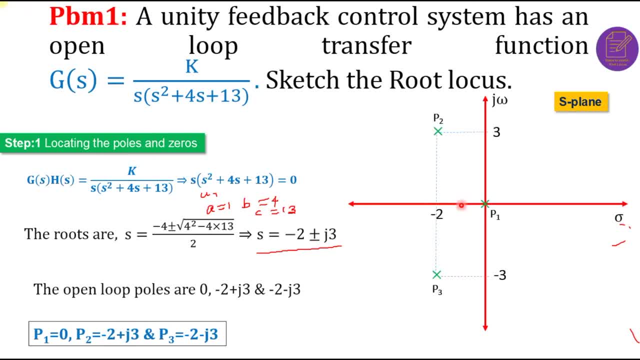 the help of the cross point. We know that. So this is the locating the poles. Okay, This is a rough diagram. Okay, I find in. finally, we will, we will take a graph sheet and we will, we will plot the roots, root location. 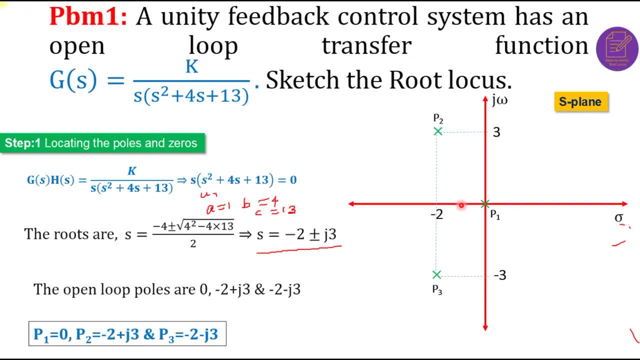 Okay, This is a rough diagram. Okay. So, in order to understand the concepts, each and every step, some some concepts is there. So, if you want to understand the concepts, you need to make it as a rough diagram, Okay, And only we can able to draw the final diagram. 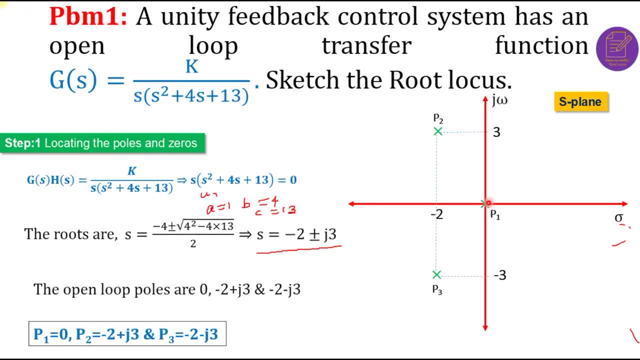 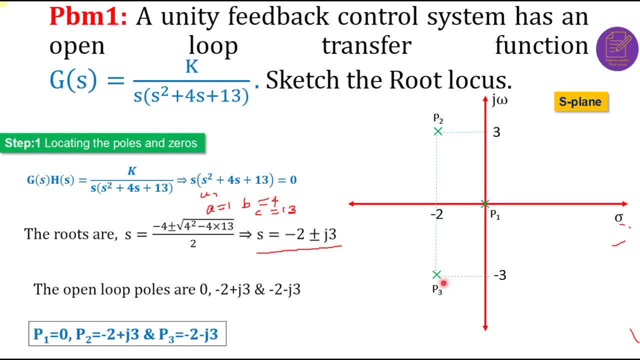 nothing but minus 2, minus j 3.. This is p 3, pole 3 value. Okay, So these three poles are shown, shown as a cross point here. So this is step 1.. Okay, Locating the poles and 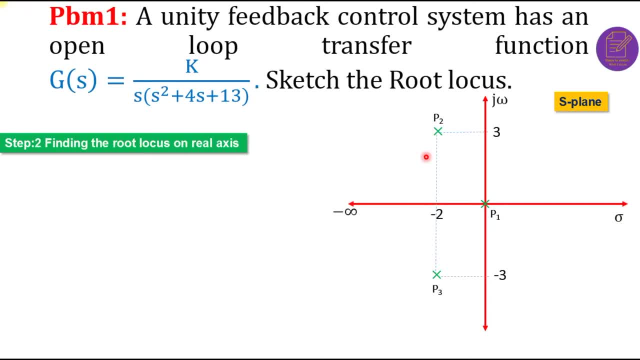 zeroes. Okay, Step 2, finding the root locus on real axis. Okay, So we need to find out the root locus on real axis. See, This is the segment. Okay, So this is the inspecting region. We can also say that this is the inspecting. 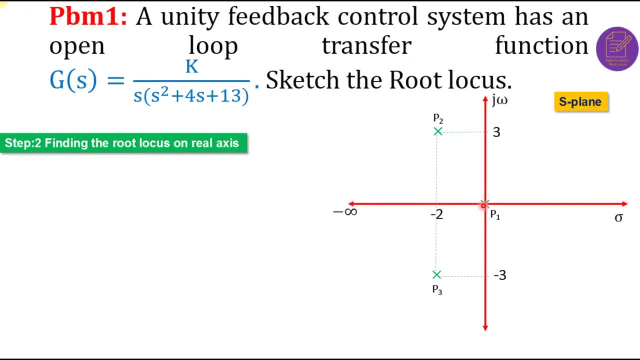 region. okay. so whether in this negative real axis any root locus is available or not, this is the question. okay, so in this step we need to focus on this area only: negative real axis, okay. negative real axis. real axis of s plane. okay, so let me, let me go and refer this material. so step two is: 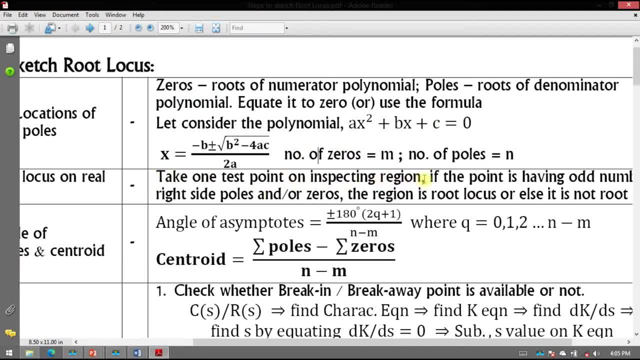 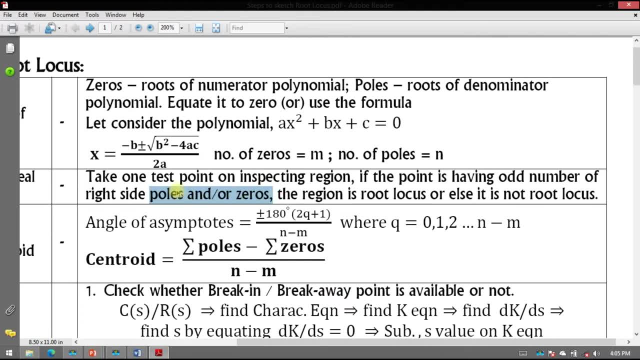 take one test point on inspecting region. if the test point is having odd number of right side poles and are zeros, okay, and the region is root locus, or else it is not root locus, okay. this is somewhat. this is somewhat having some concepts, concept, okay. so what we have to do is we need to 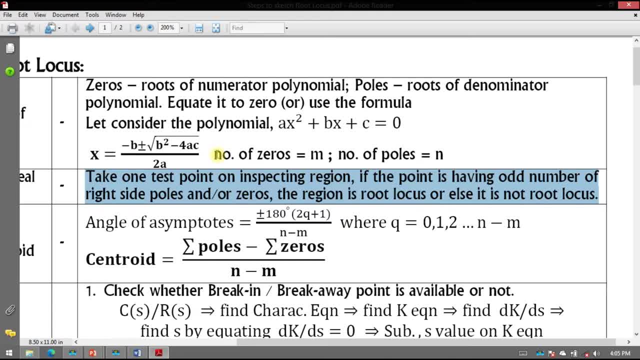 take one test point on real axis, on this negative real axis. this is what we are called as inspecting region here. okay, so if the point is having odd number of okay, the number should be in odd. okay, odd number of right side to the point on. okay, right side means, and we are telling about right side of the testing point, okay, 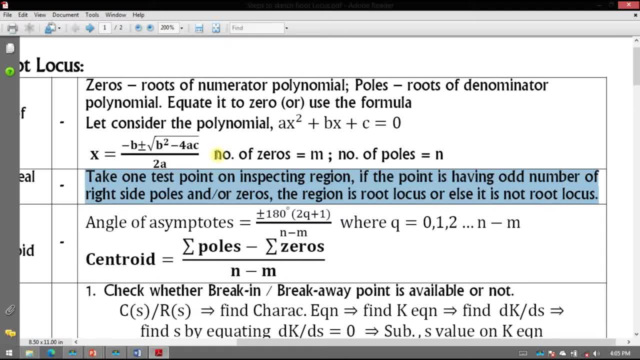 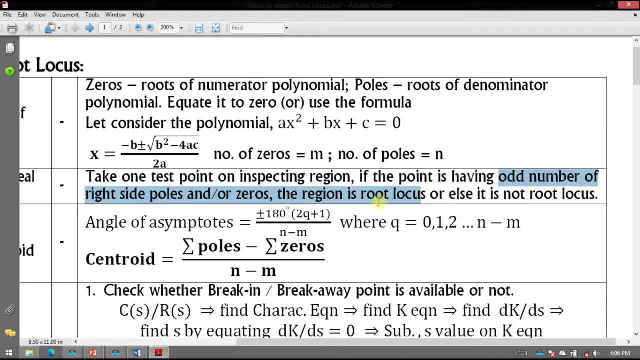 either this odd number of right side- this is constant, okay, either it may be a pole. either this odd number of right side- this is constant, okay. either it may be a pole. either this odd number of right side- this is constant, okay. either it may be a pole, either it may be zero, either it may. 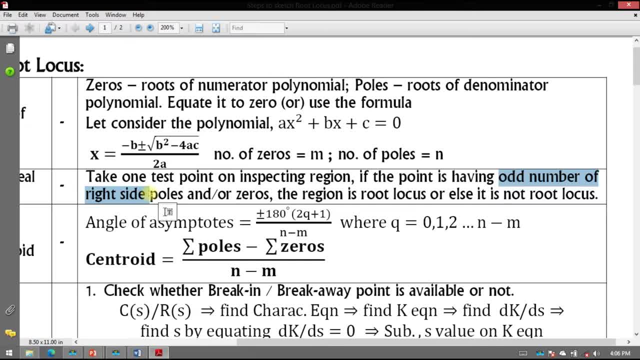 either it may be a pole, either it may be zero, either it may, either it may be a pole, either it may be a poles and it may be a poles, and zeros be a poles, and it may be a poles and zeros be a poles, and it may be a poles and zeros. okay, whatever we need, right side, the total. 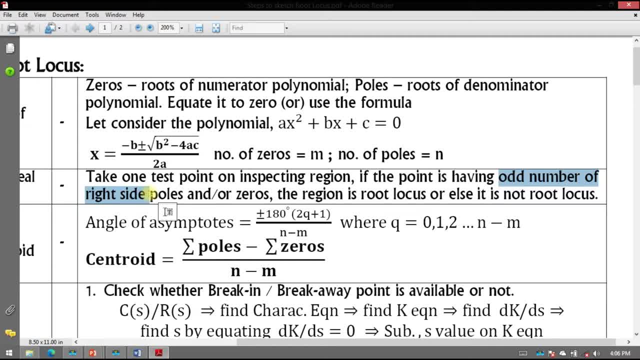 okay, whatever we need right side, the total. okay, whatever we need right side, the total, available poles. and our zero should be in available poles and our zero should be in available poles and our zero should be in odd number. then you are inspecting region, odd number, then you are inspecting region. 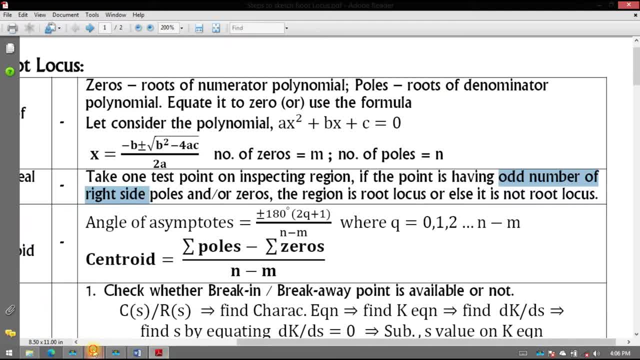 odd number, then you are inspecting region. is what the root locus or otherwise it is? is what the root locus or otherwise it is? is what the root locus or otherwise? it is not a root locus in our problem. this is not a root locus in our problem. this is. 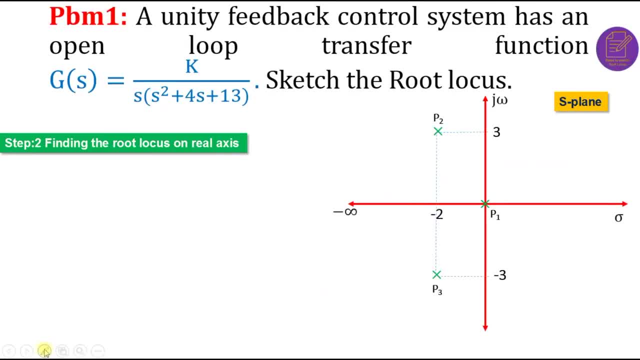 not a root locus in our problem. this is very simple, that this is the inspecting, very simple, that this is the inspecting very simple, that this is the inspecting region. am i right so we can say that we region? am i right so we can say that we? 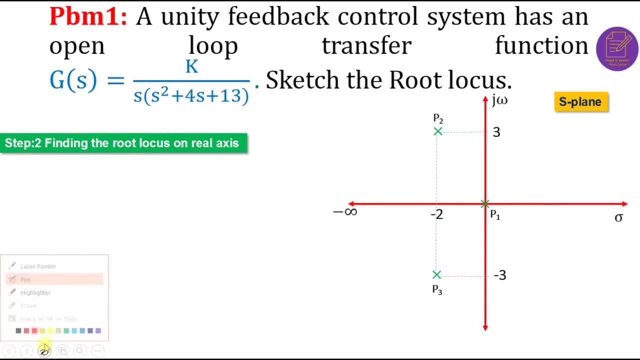 region, am i right? so we can say that we can? we can take a test point over here. can we can take a test point over here? can we can take a test point over here? okay, yeah, I'm taking, yeah, I'm taking one. okay, yeah, I'm taking, yeah, I'm taking one. 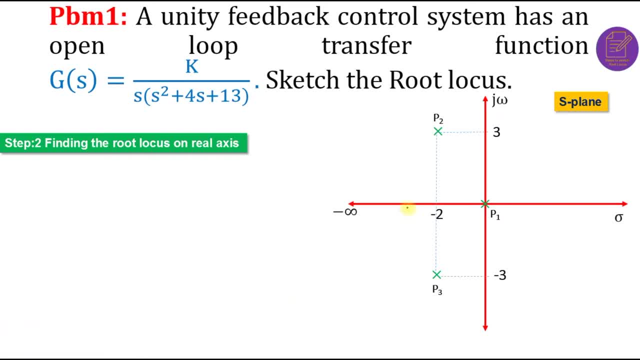 okay, yeah, I'm taking. yeah, I'm taking one testing point over here. okay, I'm taking testing point over here. okay, I'm taking testing point over here. okay, I'm taking one testing point over here. this is the one testing point over here. this is the one testing point over here. this is the test point. okay, so to the test point. 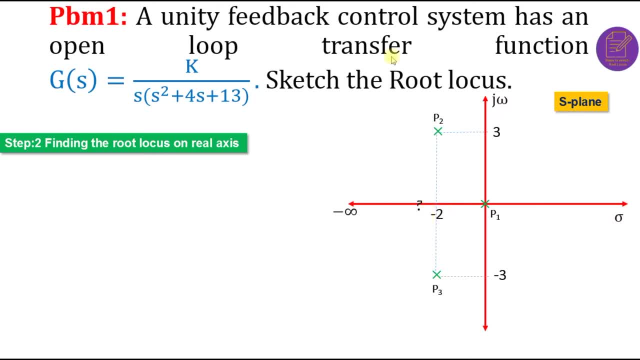 test point. okay, so to the test point. test point: okay, so to the test point. okay to the. to this test test point. what okay to the to this test test point. what okay to the to this test test point. what is the total number of right side right? 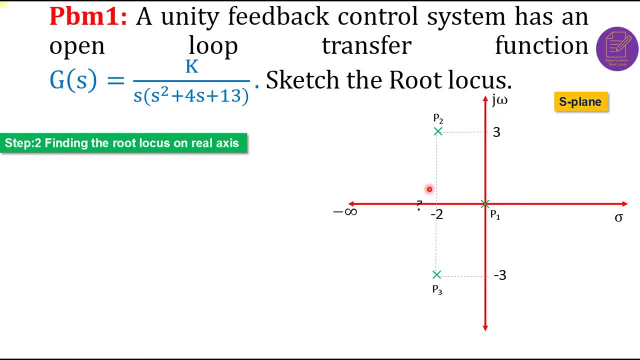 is the total number of right side right is the total number of right side right side poles and our zeros. okay to this test side poles and our zeros. okay to this test side poles and our zeros. okay to this test point point: there is only one right side poles. 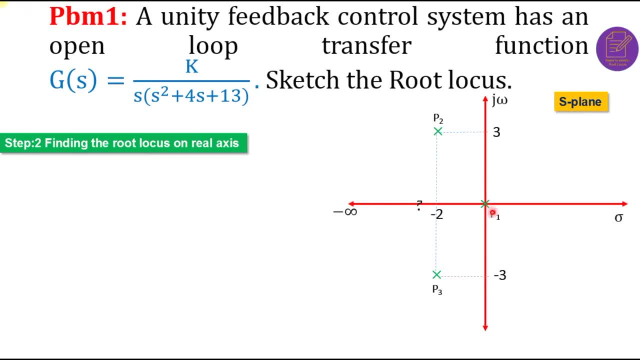 there is only one right side poles. there is only one right side poles. okay, right side to this. test, point it this. okay, right side to this test, point it this: okay, right side to this test, point it this side. am I right? so to the test point side. am I right? so to the test point. 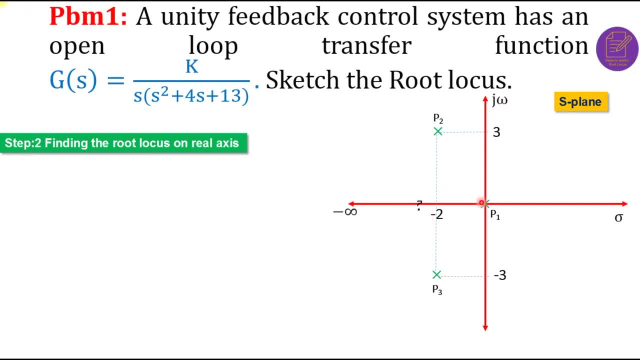 side, am I right? so to the test point: the right side poles and our zeros here in the right side poles and our zeros here in the right side poles and our zeros here in our problem we are having only poles. our problem we are having only poles. our problem we are having only poles. so right side poles are only one. okay, so 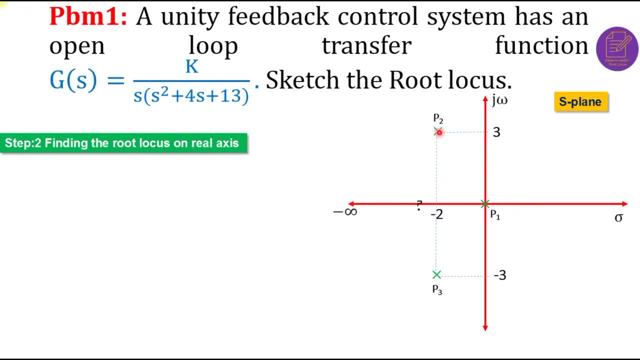 so right side poles are only one, okay, so, so right side poles are only one, okay. so in this real axis, we need to focus. in this real axis, we need to focus in this real axis. we need to focus. don't focus on the poles present at. don't focus on the poles present at. 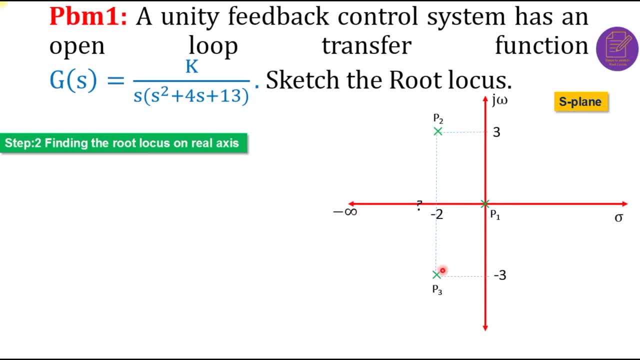 don't focus on the poles present at this second and fourth quadrant third course. this second and fourth quadrant third course. this second and fourth quadrant third course. second and third quarter: okay, we second and third quarter. okay. we second and third quarter: okay, we need to focus on only the poles and zeros. 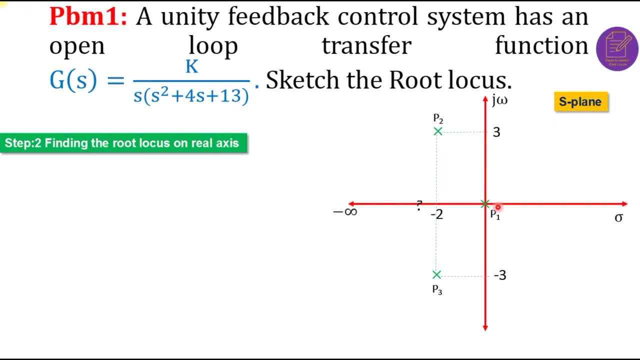 need to focus on only the poles and zeros, need to focus on only the poles and zeros. which is available in these negative, which is available in these negative, which is available in these negative real axes. that is why I told you earlier real axes. that is why I told you earlier: 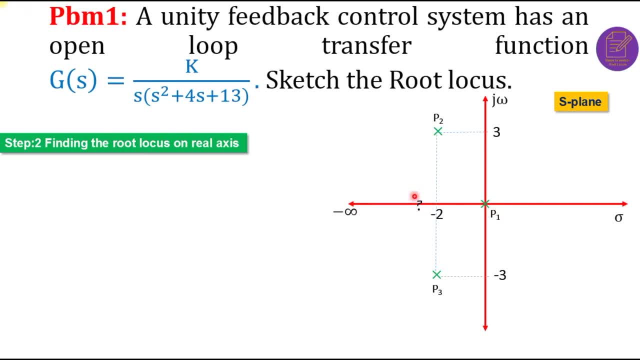 real axes. that is why I told you earlier: okay, so for this test point to this test. okay, so for this test point to this test. okay, so for this test point to this test point, there is only one odd number of point. there is only one odd number of. 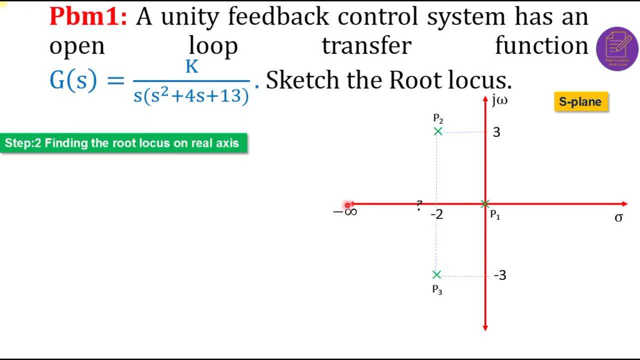 point. there is only one odd number of poles are available. so this entire region poles are available. so this entire region poles are available. so this entire region is considered as root locus as per the is considered as root locus as per the is considered as root locus as per the rules. we are telling: okay, so there is. 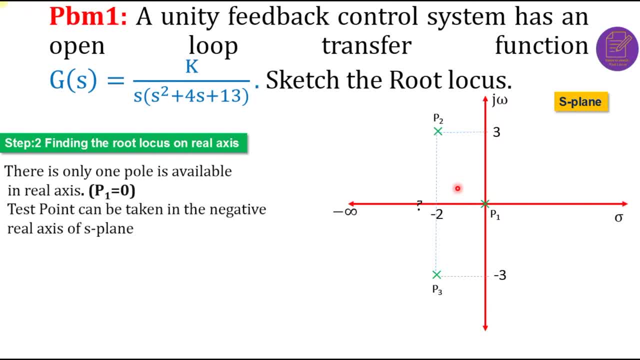 rules. we are telling okay, so there is rules. we are telling okay, so there is. only one pole is available in real axis. only one pole is available in real axis. only one pole is available in real axis. p1 equal to 0 test point can be taken in. 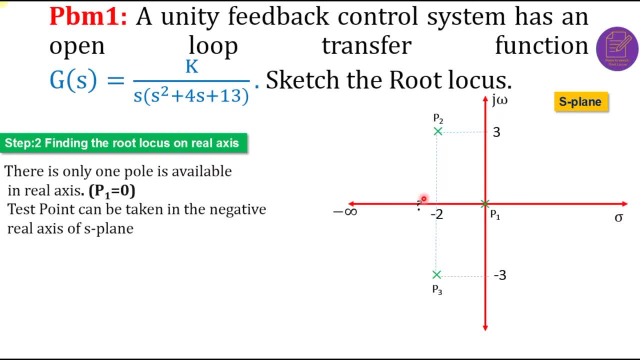 p1 equal to 0 test point can be taken in. p1 equal to 0 test point can be taken in. the negative real axis of s plane. yeah, the negative real axis of s plane. yeah, the negative real axis of s plane. yeah, this is taken here, over here and to the 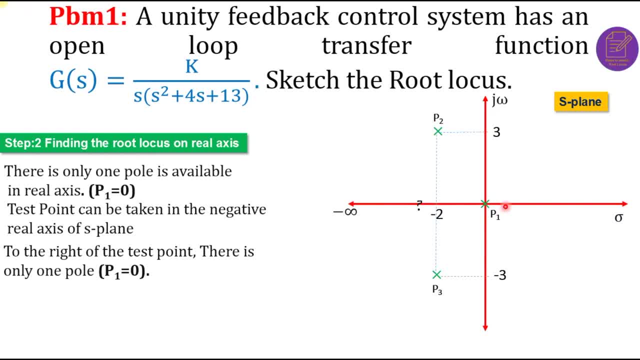 this is taken here over here. and to the: this is taken here over here. and to the right of the test point: there is one right of the test point. there is one right of the test point. there is one. only one pole is available, we already. only one pole is available, we already. 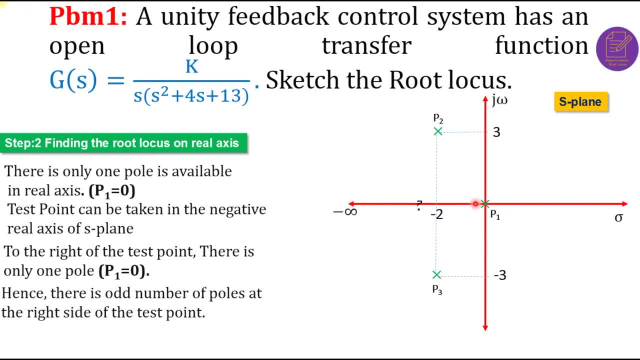 only one pole is available. we already discussed, right hence there is. there is discussed, right hence there is. there is discussed, right hence there is. there is a odd number of poles at the right side, a odd number of poles at the right side, a odd number of poles at the right side of the test point. yes, of course. so the 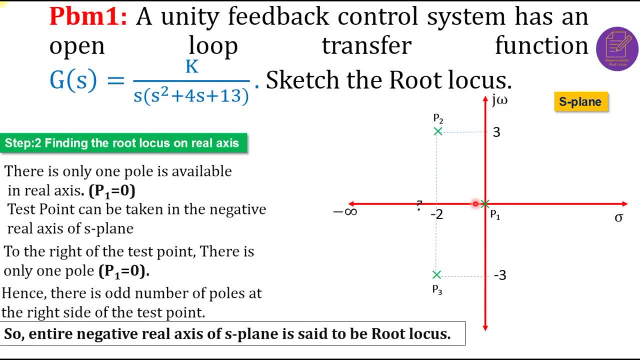 of the test point? yes, of course. so the of the test point? yes, of course. so the entire negative real axis of. I mean the entire negative real axis of. I mean the entire negative real axis of. I mean the inspecting region is said to be root. inspecting region is said to be root. 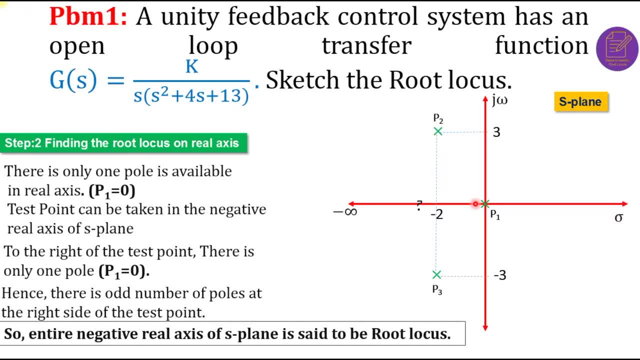 inspecting region is said to be root locus. okay. so if you want to, if you want locus, okay. so if you want to, if you want locus, okay. so if you want to. if you want to highlight, okay, the step 2 in your to highlight, okay, the step 2 in your. 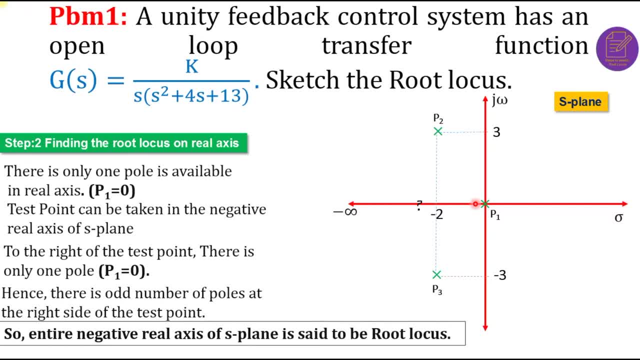 to highlight, okay, the step 2 in your rough diagram, so that we know we predicted rough diagram, so that we know we predicted rough diagram, so that we know we predicted that the entire negative real axis is that the entire negative real axis is that the entire negative real axis is root locus. okay, just highlight the line. 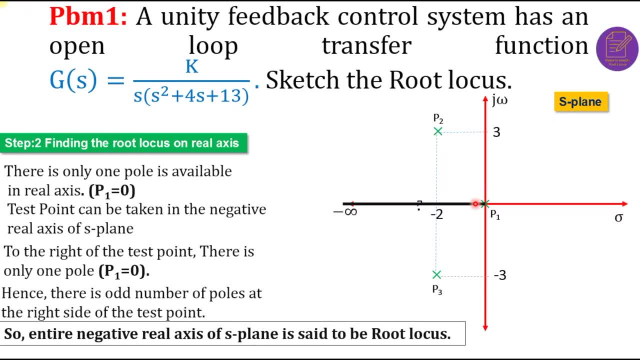 root locus. okay, just highlight the line: root locus. okay, just highlight the line. okay, with more thicker line. so this is okay with more thicker line. so this is okay with more thicker line. so this is the symbolic representation of root, the symbolic representation of root, the symbolic representation of root locus here. okay, so if you want to, 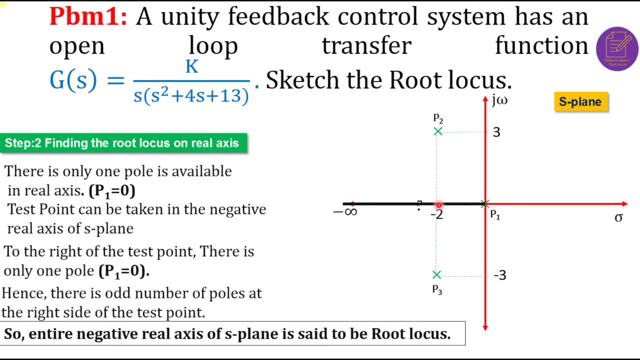 locus here: okay. so if you want to locus here, okay. so if you want to differentiate the axis with the root, differentiate the axis with the root, differentiate the axis with the root. locus- you need to make it as thick line. locus- you need to make it as thick line. 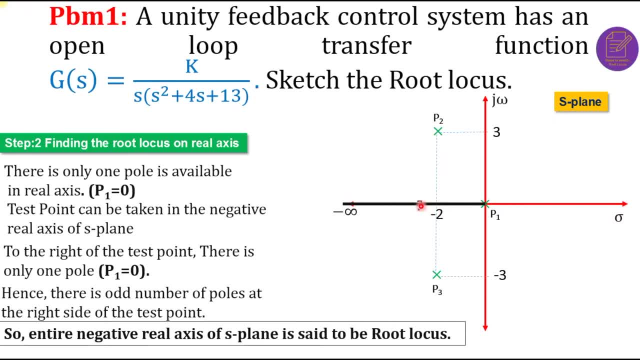 locus. you need to make it as thick line, okay, so this is the symbolic. okay, so this is the symbolic, okay. so this is the symbolic representation of the real axis root, representation of the real axis root, representation of the real axis root locus. okay, if we go into the third step, 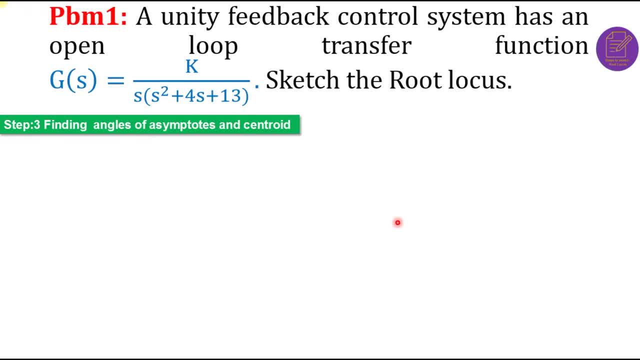 locus. okay, if we go into the third step. locus. okay, if we go into the third step: finding angles of asymptotes and finding angles of asymptotes and finding angles of asymptotes and centroids. okay, so let me refer to the centroids. okay, so let me refer to the. 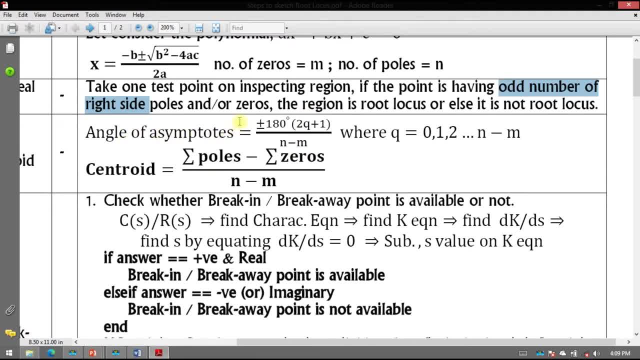 centroids. okay, so let me refer to the rule book here. angles of asymptotes is rule book here. angles of asymptotes is rule book here. angles of asymptotes is equal to plus or minus 180 degree. into equal to plus or minus 180 degree. into equal to plus or minus 180 degree. into 2q plus 1 divided by n minus M, where Q. 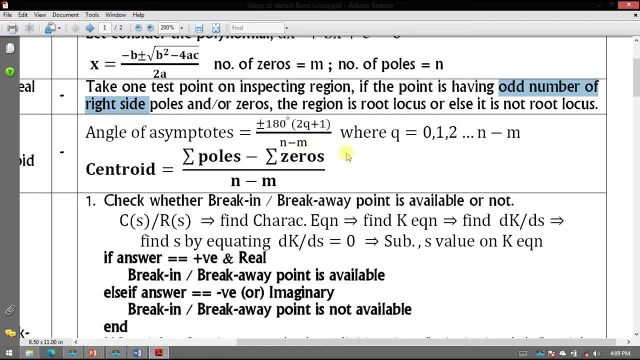 2q plus 1 divided by n minus M. where Q, 2q plus 1 divided by n minus M, where Q is equal to 0, 1, 2 up to n minus M, we is equal to 0, 1, 2 up to n minus M we. 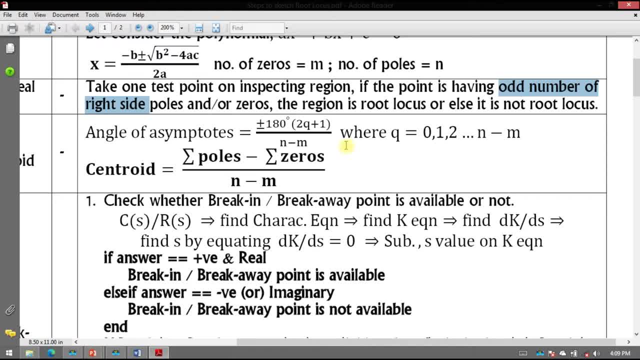 is equal to 0, 1, 2, up to n minus M. we know that n is number of poles M is. know that n is number of poles M is. know that n is number of poles. M is number of zeros. centroid means sum of number of zeros. centroid means sum of. 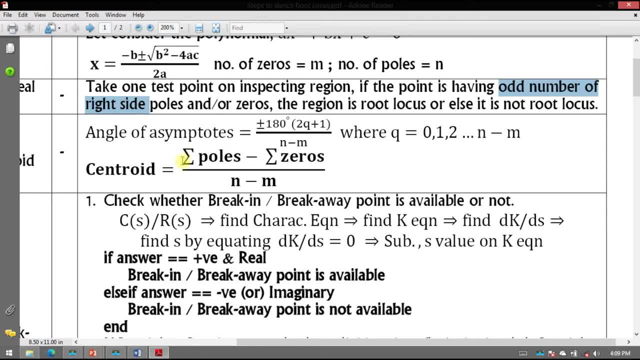 number of zeros. centroid means sum of poles minus sum of zeros divided by n poles, minus sum of zeros divided by n poles minus sum of zeros divided by n minus M. this is a simple formulas. we are minus M. this is a simple formulas. we are minus M. this is a simple formulas we are having. okay, so there are three poles. 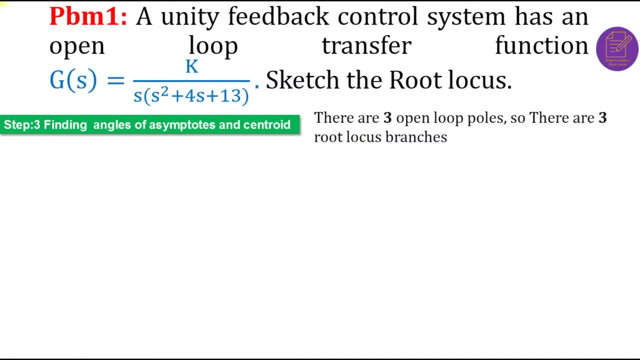 having okay, so there are three poles. having okay, so there are three poles. okay, there are three open poles. we are okay, there are three open poles. we are okay, there are three open poles. we are having now system, we are having three. having now system, we are having three. 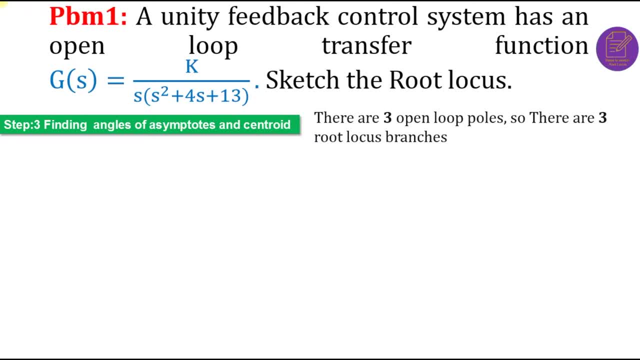 having now system, we are having three poles. there are three root locus branches poles. there are three root locus branches poles. there are three root locus branches. is there okay? so this is a very simple, is there okay? so this is a very simple, is there okay? so this is a very simple and important thumb rule over here. so 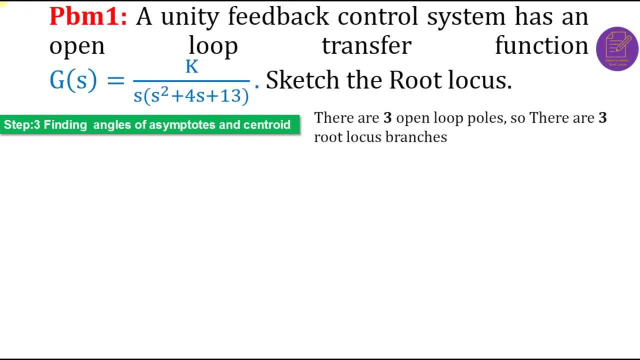 and important thumb rule over here. so and important thumb rule over here. so there are three open poles. the number of there are three open poles, the number of there are three open poles. the number of poles, the number of root locus branches- poles, the number of root locus branches. 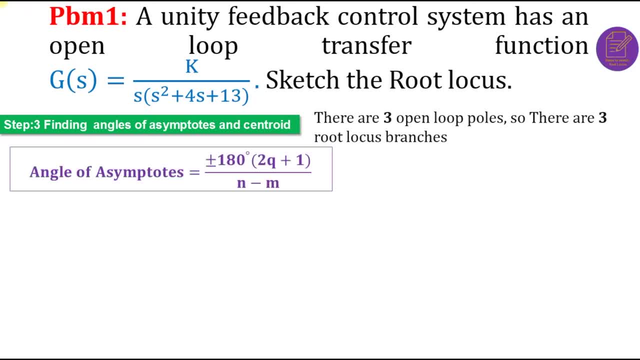 poles. the number of root locus branches is equal to the number of open loop, is equal to the number of open loop is equal to the number of open loop poles. okay, so angles of asymptotes. we poles. okay, so angles of asymptotes. we poles. okay, so angles of asymptotes. we already referred this formula, right, just. 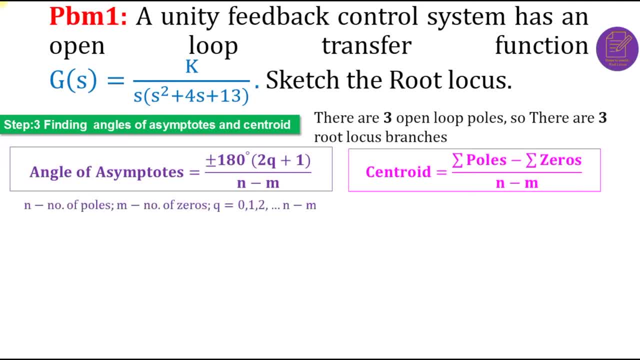 already referred this formula right. just already referred this formula right, just simply. we also know about the centroid, simply. we also know about the centroid simply. we also know about the centroid value. so n is a number of poles, M is value. so n is a number of poles, M is 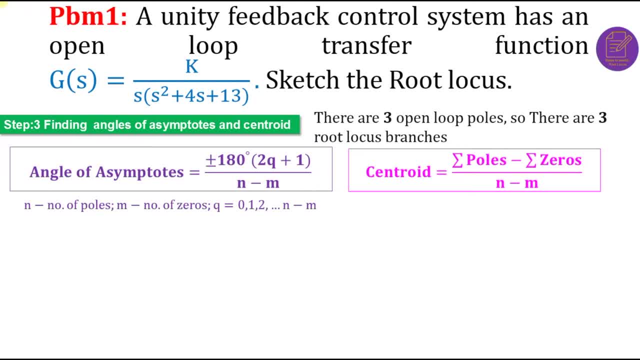 value. so n is a number of poles, M is zeros and Q is equal to 0, 1, 2 up to n zeros and Q is equal to 0, 1, 2 up to n zeros and Q is equal to 0, 1, 2 up to n minus 1. so let's substitute the value of 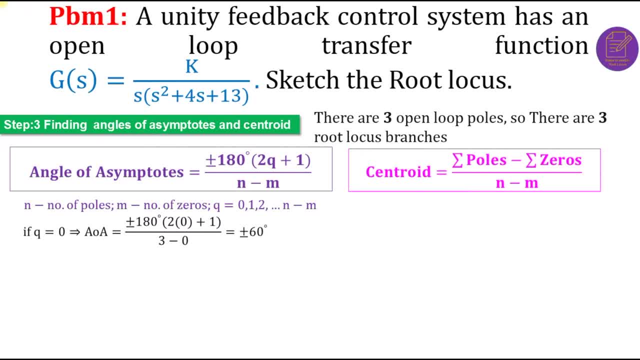 minus 1. so let's substitute the value of minus 1. so let's substitute the value of Q is 0 here. so we are having the OA Q is 0 here. so we are having the OA Q is 0 here. so we are having the OA angles of asymptotes as 16 degree. I mean. 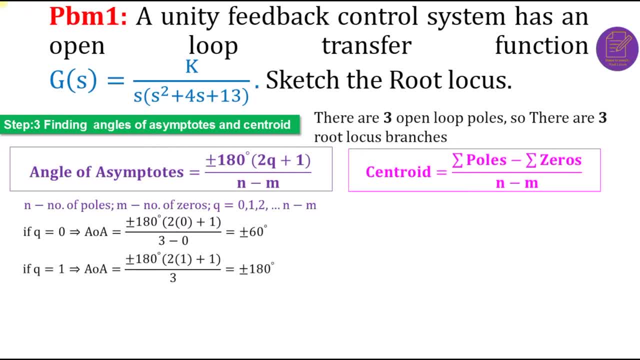 angles of asymptotes as 16 degree. I mean angles of asymptotes as 16 degree, I mean plus or minus 60 degree, and then for the plus or minus 60 degree, and then for the plus or minus 60 degree, and then for the value of Q equal to 1, the plus or minus. 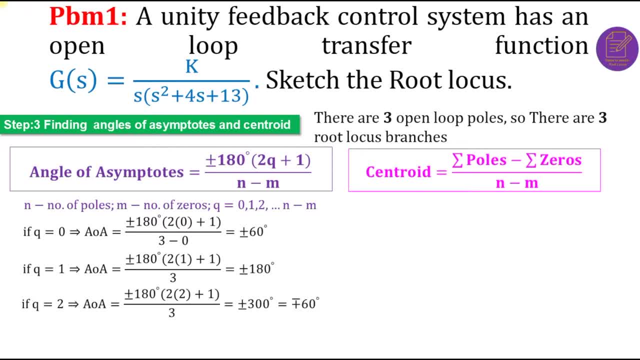 value of Q equal to 1, the plus or minus value of Q equal to 1, the plus or minus 180 degrees there. and for the value of Q, 180 degrees there. and for the value of Q, 180 degrees there. and for the value of Q equal to 2, there is the repetition of the. 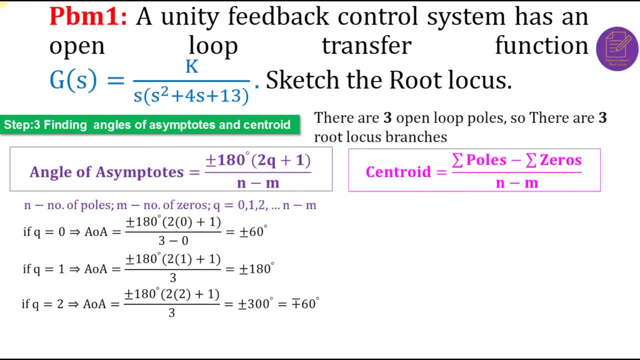 equal to 2. there is the repetition of the equal to 2. there is the repetition of the first angle. is we are getting I mean first angle? is we are getting I mean first angle? is we are getting I mean plus or minus the 300 degree or? 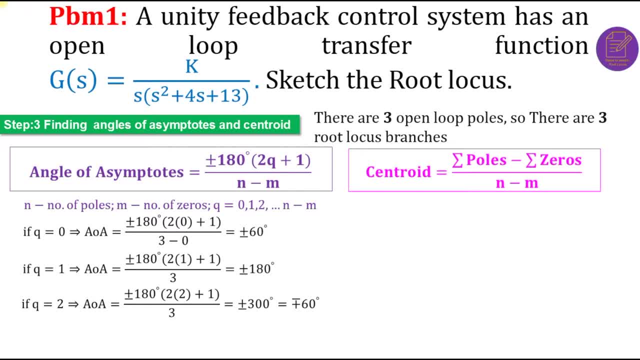 plus or minus the 300 degree, or plus or minus the 300 degree, or otherwise. minus or plus 60 degree, okay, otherwise. minus. or plus 60 degree, okay, otherwise. minus or plus 60 degree, okay, either both of them is same, okay, so now. either both of them is same, okay, so now. 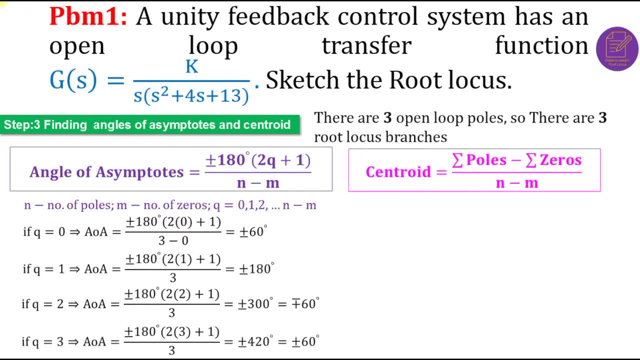 either. both of them is same, okay. so now, if you are, if you are increasing the, if you are, if you are increasing the, if you are, if you are increasing the value of Q, as 3 means we are getting value of Q, as 3 means we are getting. 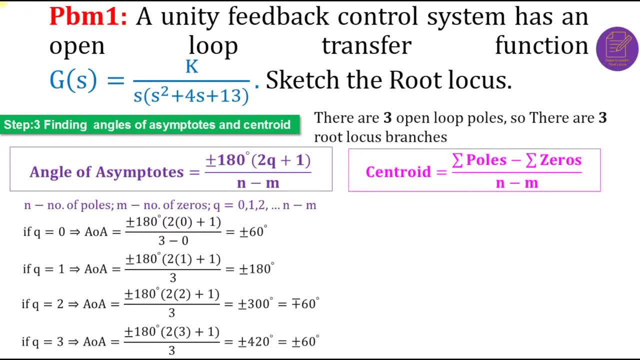 value of Q as 3 means we are getting again. we are getting plus or minus 60. so again we are getting plus or minus 60. so again we are getting plus or minus 60. so the- the value is continuously repeated. the, the- the value is continuously repeated. 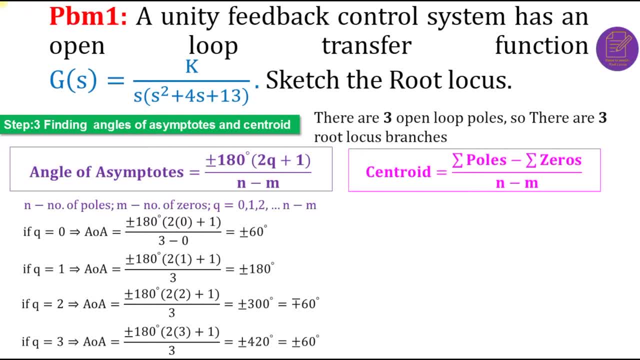 the, the, the value is continuously repeated: okay, 60, 180, 60, 180 likewise. this is the okay: 60 180, 60, 180. likewise. this is the okay: 60 180, 60, 180 likewise. this is the angle of asymptotes, value and centroid. 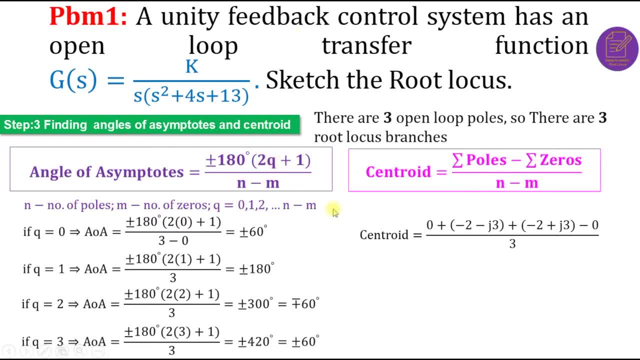 angle of asymptotes, value and centroid. angle of asymptotes, value and centroid. we're talking about the centroid value. we're talking about the centroid value. we're talking about the centroid value. we know that the roots of this I mean. we know that the roots of this, I mean. 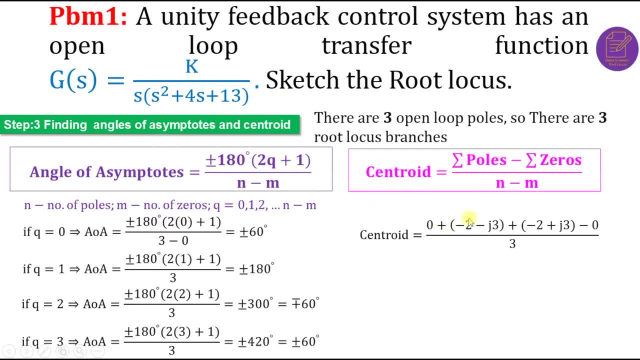 we know that the roots of this, I mean, and the open-loop poles. we know that is. and the open-loop poles, we know that is. and the open-loop poles. we know that is equal to 0 minus 2 plus 2 J 3. sorry, yeah. 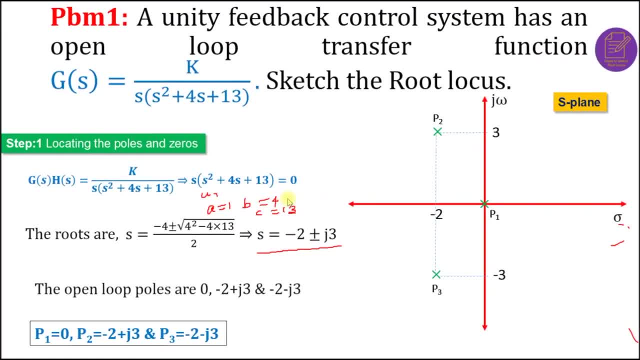 equal to 0 minus 2 plus 2 J 3- sorry, yeah. equal to 0 minus 2 plus 2 J 3- sorry, yeah. this is, these are all the poles we are. this is these are all the poles we are. this is these are all the poles we are. having right, these are all the poles: 0. 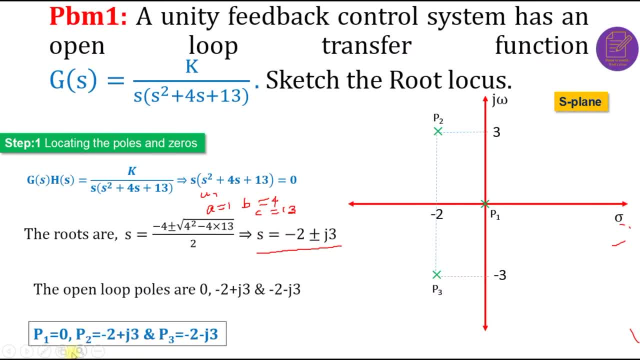 having right. these are all the poles. 0 having right. these are all the poles: 0 minus 2 plus J 3 and minus 2 minus J 3, minus 2 plus J 3 and minus 2 plus J 3, minus 2 plus J 3 and minus 2 plus J 3. this is all the poles we are having okay. 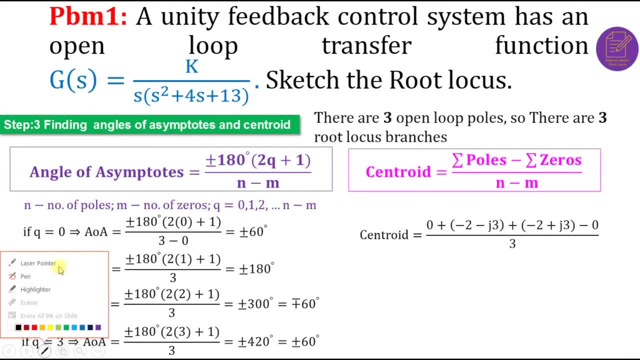 this is all the poles we are having. okay, this is all the poles we are having, okay. so we are just summing all the poles. so we are just summing all the poles. so we are just summing all the poles, open-loop poles, and there is no zeros. 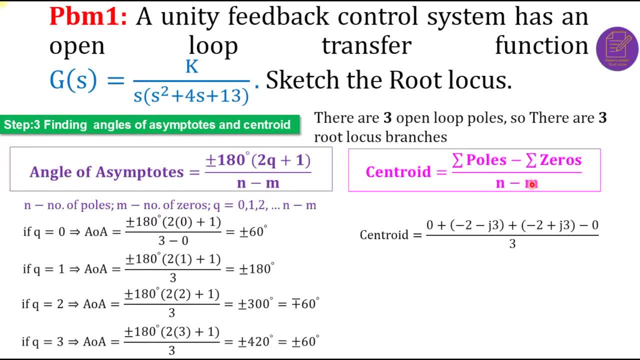 open-loop poles and there is no zeros. open-loop poles and there is no zeros over there. divided by 3 n minus M, that over there, divided by 3 n minus M, that over there, divided by 3 n minus M, that is 3 minus 0, is 3. okay, the centroid. 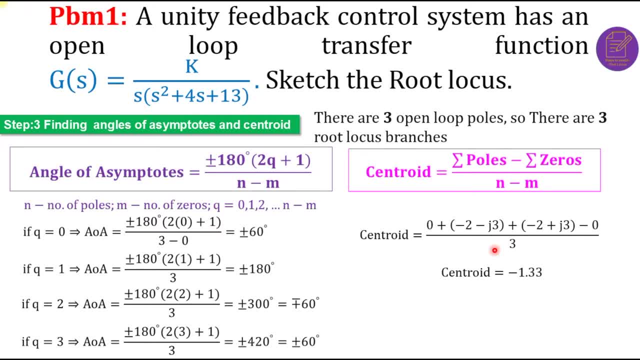 is 3 minus 0 is 3- okay. the centroid is 3 minus 0 is 3- okay. the centroid value is minus 1.33- we are getting okay. value is minus 1.33: we are getting okay. value is minus 1.33- we are getting okay. so this is the angles of asymptotes and 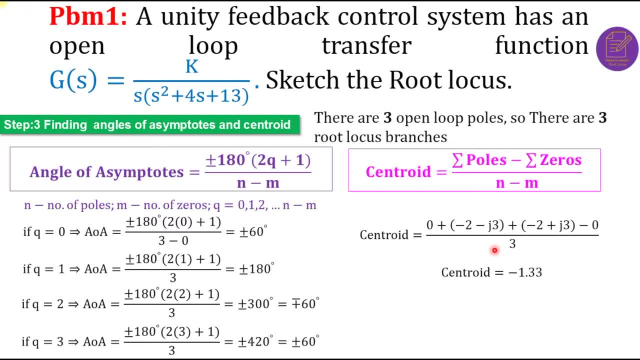 so this is the angles of asymptotes, and so this is the angles of asymptotes and centroids. okay, see, root locus is nothing, centroids. okay, see, root locus is nothing, centroids. okay, see, root locus is nothing, but the? it is a graphical method, I told. but the? it is a graphical method, I told. 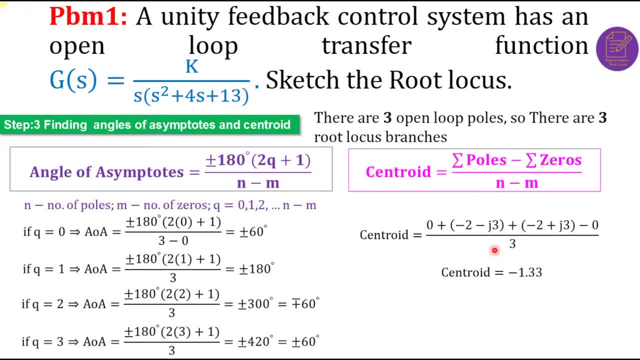 but the it is a graphical method. I told earlier: okay, this is a graphical earlier. okay, this is a graphical earlier. okay, this is a graphical representation of the possible locations. representation of the possible locations, representation of the possible locations, of the closed-loop poles in order to of the closed-loop poles in order to. 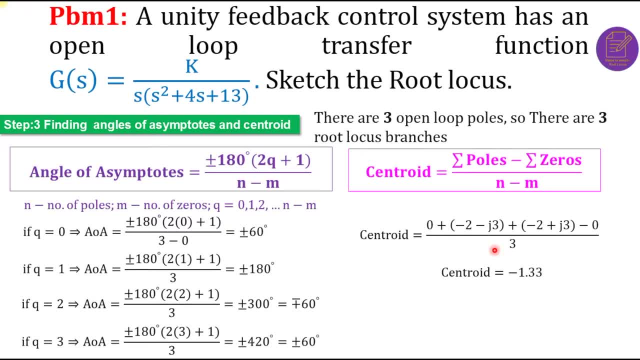 of the closed-loop poles in order to meet up the stability. okay, so see, the meet up the stability. okay, so see the meet up the stability. okay, so see, the one thing is that we already find the one thing is that we already find, the one thing is that we already find the real axis root locus. okay, so the. 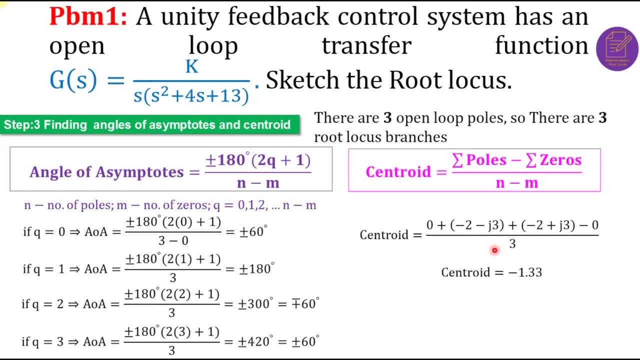 real axis root locus. okay. so the real axis root locus. okay. so the closed-loop poles may available in closed-loop poles may available in closed-loop poles may available in negative. negative I mean available in negative. negative I mean available in negative. negative I mean available in entire negative real axis like this: okay. 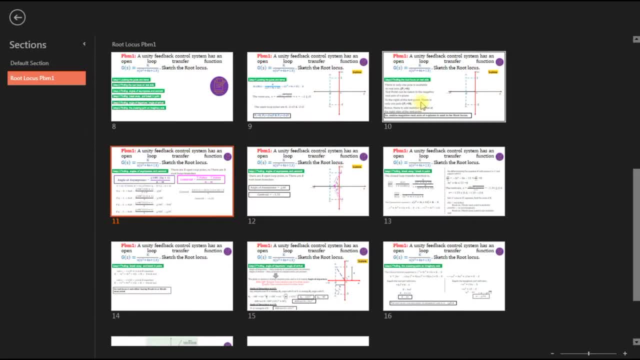 entire negative real axis like this. okay, entire negative real axis like this. okay, see, I will show you the second step. see, I will show you the second step. see, I will show you the second step here. see, we already told you right the in here. see, we already told you right the in. 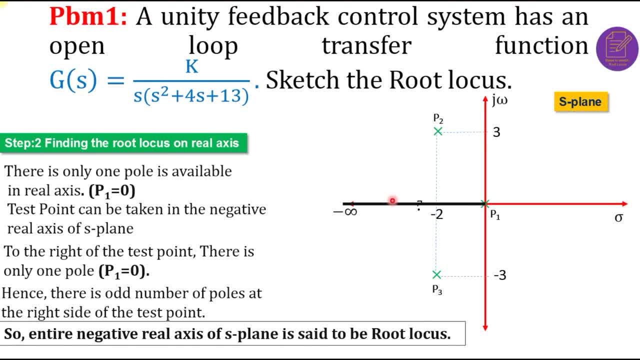 here. see, we already told you right: the in order to maintain the stability, the order to maintain the stability, the order to maintain the stability, the closed-loop poles may available in these closed-loop poles may available in these closed-loop poles may available in these entire negative real axis, whatever in. 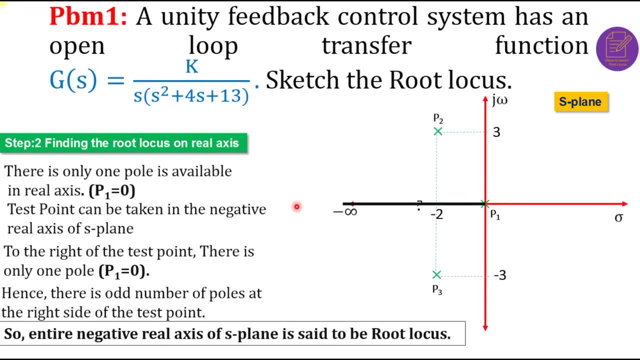 entire negative real axis whatever. in entire negative real axis, whatever. in which places of negative real axis, the which places of negative real axis, the which places of negative real axis, the closed-loop poles may available. okay, so, closed-loop poles may available. okay, so, closed-loop poles may available. okay, so, based upon the different values of K, we 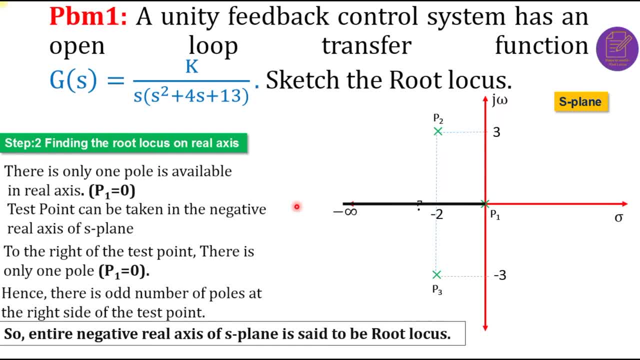 based upon the different values of K. we, based upon the different values of K, we can get the different numbers of, can get the different numbers of, can get the different numbers of negative real axis poles. I mean closed negative real axis poles. I mean closed negative real axis poles. I mean closed loop holes. this is a symbolic 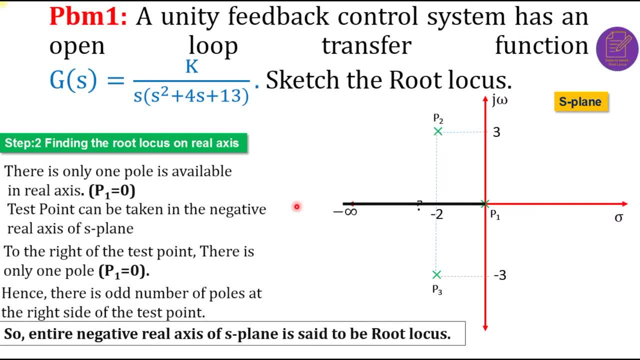 loop holes. this is a symbolic loop holes. this is a symbolic representation. okay, so this is the representation. okay, so this is the representation. okay, so this is the possible locations, similarly the the root possible locations, similarly the the possible locations, similarly the the root locus may have the some branches in. 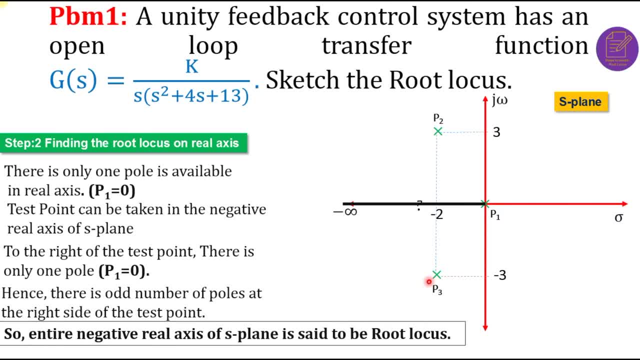 locus may have the some branches in locus may have the some branches in this quadrant, also second quadrant, our this quadrant, also second quadrant. our this quadrant, also second quadrant, our third quadrant. they may also vary, they third quadrant, they may also vary, they third quadrant. they may also vary, they may also having some branches in this. 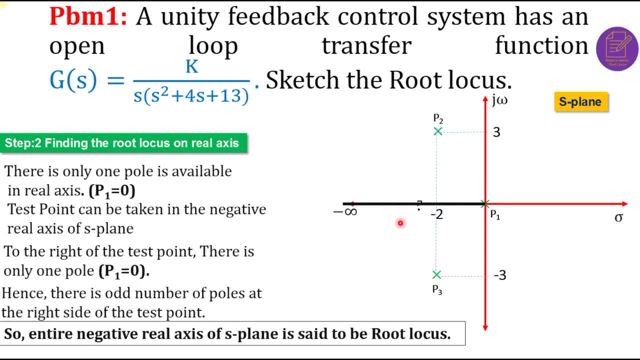 may also having some branches in this, may also having some branches in this second and third quadrant. okay, so, in second and third quadrant. okay, so, in second and third quadrant. okay. so, in order to find out the second and third order to find out the second and third. 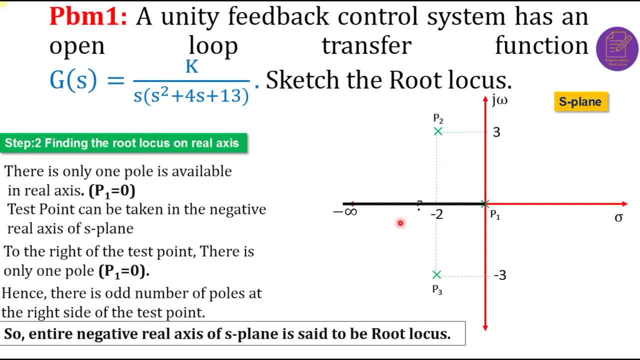 order to find out the second and third quadrant. I mean the directions of that quadrant. I mean the directions of that quadrant, I mean the directions of that particular branches. okay, we need that, we particular branches. okay, we need that, we particular branches. okay, we need that, we need a guidance. okay, if you want to you. 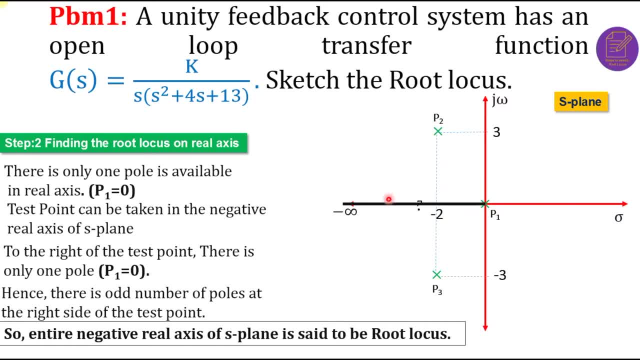 need a guidance. okay, if you want to. you need a guidance. okay, if you want to. you see you just drawn this negative real. see you just drawn this negative real. see you just drawn this negative real axis because we are having one pathway axis, because we are having one pathway. 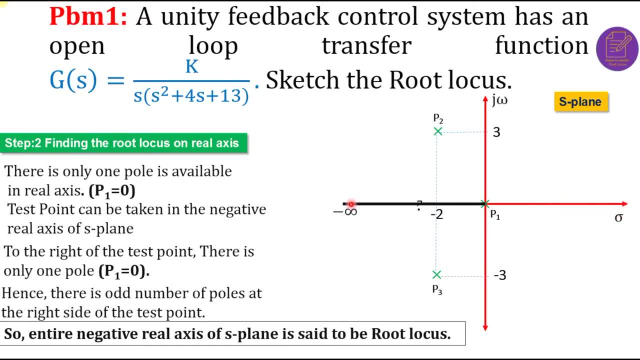 axis, because we are having one pathway in that, okay, this negative real axis is in that okay, this negative real axis is in that, okay, this negative real axis is already having one path and we are not already having one path. and we are not already having one path and we are not in the need of any guidance other than. 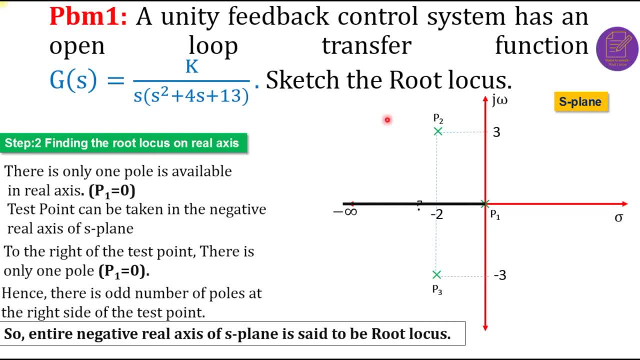 in the need of any guidance other than in the need of any guidance other than that. but roughly we are going to have that, but roughly we are going to have that, but roughly we are going to have one branch here and also one more. one branch here and also one more. 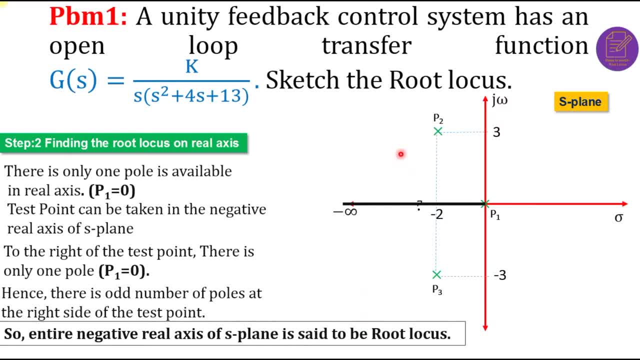 one branch here and also one more symmetrical branch will be available here. symmetrical branch will be available here. symmetrical branch will be available here. okay, either okay, either okay, either any in which direction it may available, any in which direction it may available. any in which direction it may available. for whatever may be, we need the guidance. 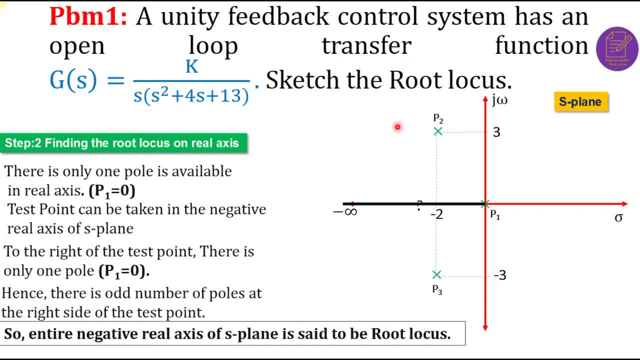 for whatever may be, we need the guidance. for whatever may be, we need the guidance. okay, so, okay, in this direction, towards, okay, so, okay, in this direction, towards, okay, so, okay, in this direction, towards this direction, to paddle with this, this direction, to paddle with this, this direction, to paddle with this direction, to paddle with this axis. 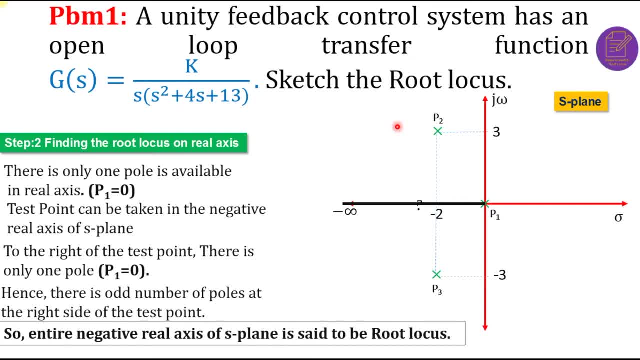 direction to paddle with this axis. direction to paddle with this axis- the branch will go likewise. we need the- the branch will go likewise. we need the- the branch will go likewise. we need the guidance in order to draw the branches. guidance in order to draw the branches. guidance in order to draw the branches which is not available in negative real 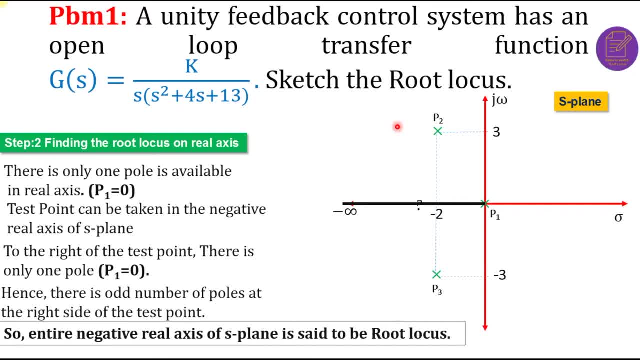 which is not available in negative real, which is not available in negative real axis. other than that, i mean second axis. other than that, i mean second axis. other than that, i mean second quadrant and third quadrant root locus quadrant and third quadrant root locus quadrant and third quadrant root locus branches. if you want to draw the second. 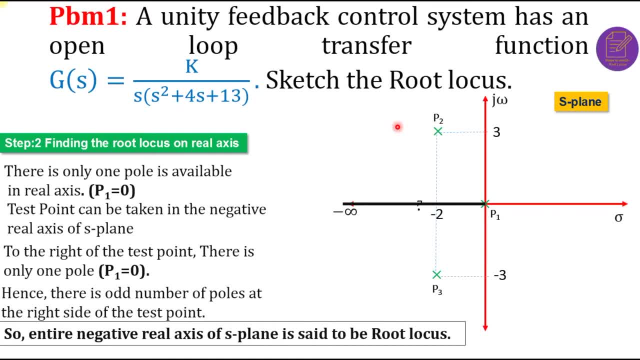 branches, if you want to draw the second branches, if you want to draw the second and third quadrant root locus branches and third quadrant root locus branches and third quadrant root locus branches. we need a very good guidance, we need a very good guidance, we need a very good guidance. so these are all the guiding, guiding. 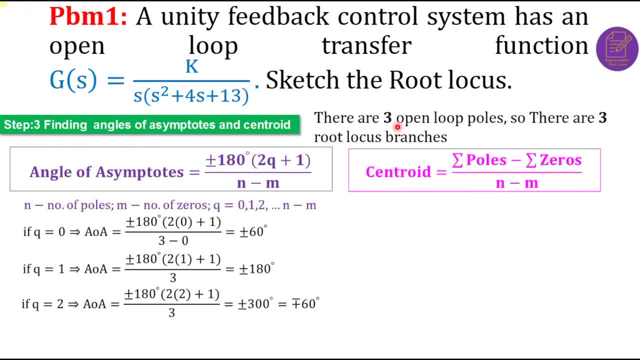 so these are all the guiding guiding. so these are all the guiding guiding parameters. what are all the guiding parameters? what are all the guiding parameters? what are all the guiding parameters? angles of asymptotes and parameters. angles of asymptotes and parameters. angles of asymptotes and centroids. 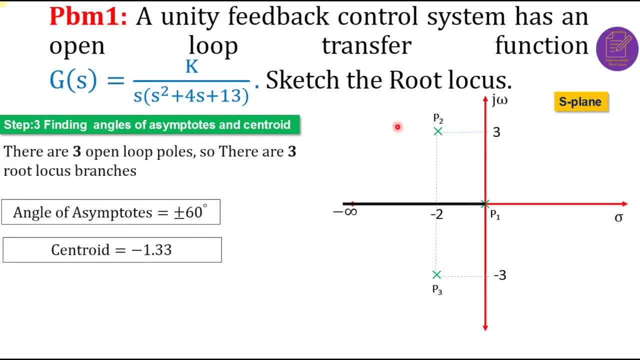 centroids, centroids. okay, so we are going to. okay, so we are going to okay, so we are going to take centroid as minus 1.3, take centroid as minus 1.3, take centroid as minus 1.3. so what we have to do is okay, so. 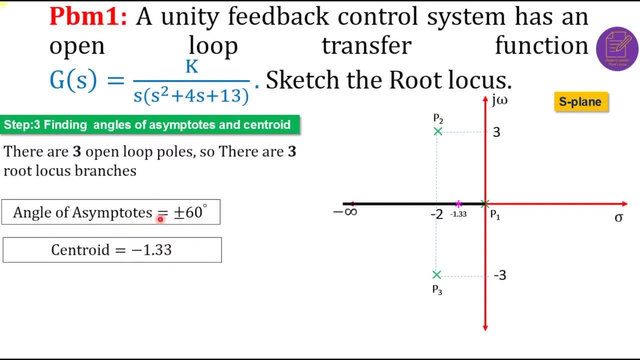 so what we have to do is okay, so, so what we have to do is okay. so we are, we need to locate this point in. we are, we need to locate this point in. we are, we need to locate this point in our real axis, because this is only having 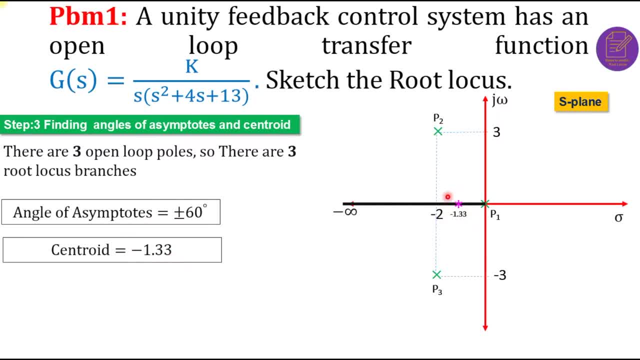 our real axis, because this is only having our real axis, because this is only having real value, negative real value. so here real value, negative real value. so here real value, negative real value. so here you can able to see minus 1.33 is. you can able to see minus 1.33 is. 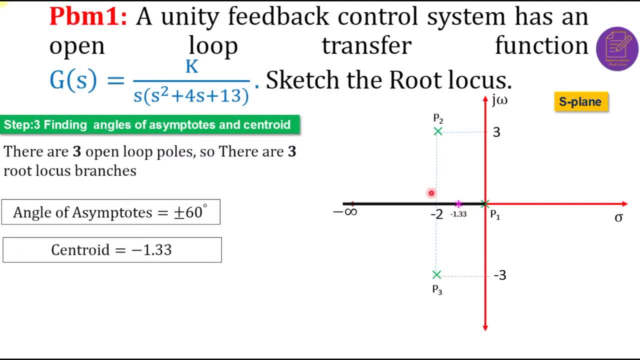 you can able to see. minus 1.33 is located here. you need to take your located here. you need to take your located here. you need to take your protector and make the angle plus 60 protector and make the angle plus 60 protector and make the angle plus 60 degree over here and minus 60 degree. 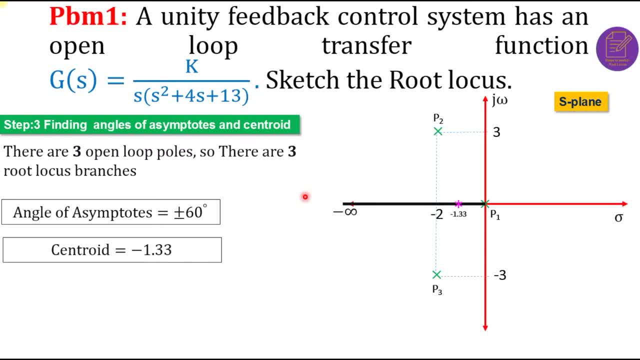 degree over here and minus 60 degree. degree over here and minus 60 degree. plus 60 degree means you need to go in plus 60 degree means you need to go in. plus 60 degree means you need to go in negative- i mean anti-clockwise- direction. 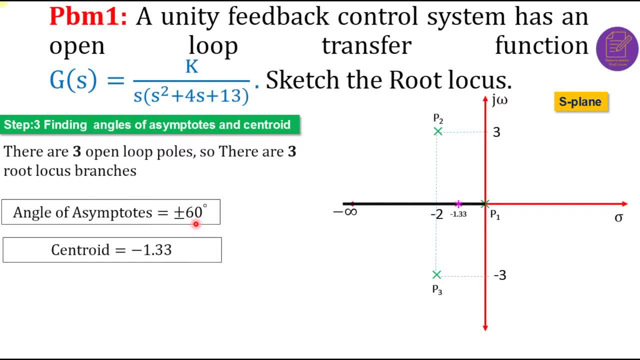 negative i mean anti-clockwise direction. negative i mean anti-clockwise direction. okay, minus 60 degree means you need to go. okay. minus 60 degree means you need to go. okay. minus 60 degree means you need to go into clockwise direction. okay, into clockwise direction, okay. 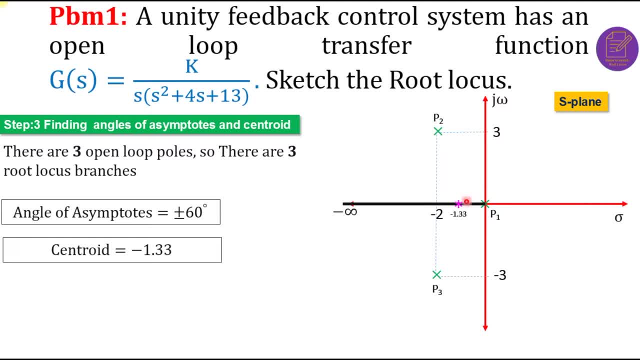 into clockwise direction. okay, so take your protector in this direction, so take your protector in this direction, so take your protector in this direction, and take, and take and take 60 degree- okay, that is one asymptote. 60 degree- okay, that is one asymptote. 60 degree: okay, that is one asymptote. okay, and kindly reverse your protector. 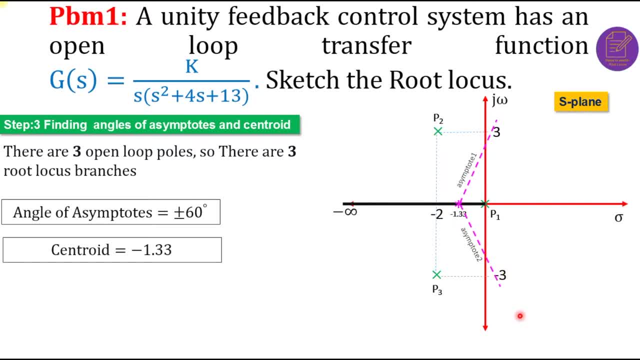 okay, and kindly reverse your protector. okay, and kindly reverse your protector and find the 60 degree angle over here, and find the 60 degree angle over here, and find the 60 degree angle over here, and this is what we are called as, and this is what we are called as. 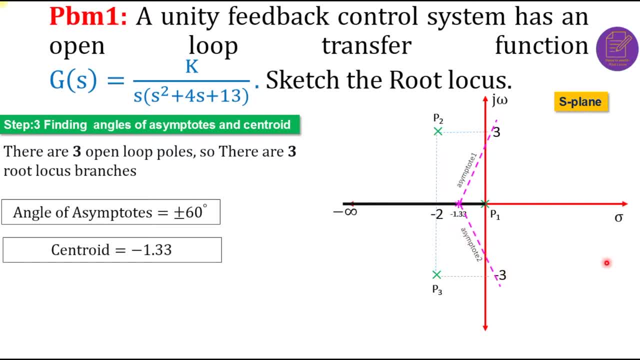 and this is what we are called as asymptote 2: asymptote 2, asymptote 2: okay, this is the pathway or guidance, okay. okay, this is the pathway or guidance, okay. okay, this is the pathway or guidance, okay. in parallel with this line, only our. 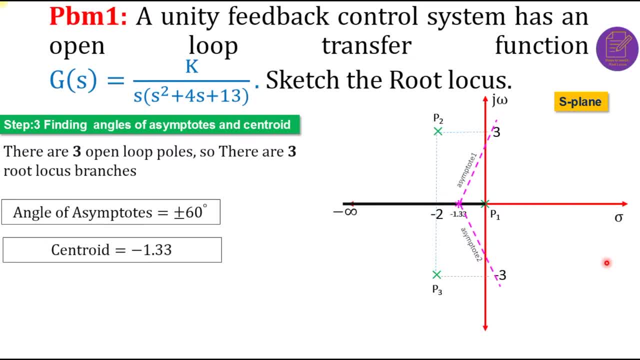 in parallel with this line, only our, in parallel with this line, only our second and third root locus branches will second and third root locus branches, will second and third root locus branches will be there, be there, be there. okay, this is the simple guidance, okay, okay, this is the simple guidance okay. 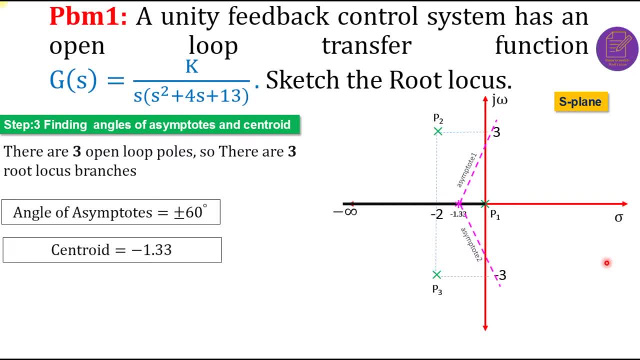 okay, this is the simple guidance. okay, based on this direction, we can able to. based on this direction, we can able to. based on this direction, we can able to draw, the draw, the draw the second and third root locus branches: okay, second and third root locus branches: okay. 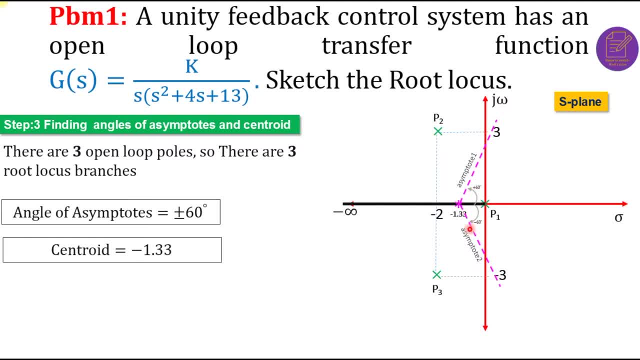 second and third root locus branches: okay, so the angle is plus 60 degree here. so the angle is plus 60 degree here. so the angle is plus 60 degree here, here, minus 60 degree. okay, so this is the here minus 60 degree. okay, so this is the. 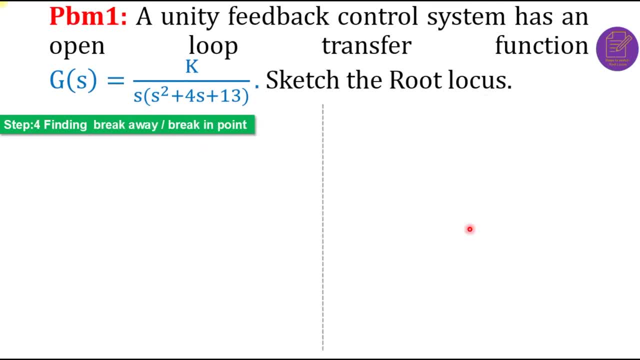 here minus 60 degree. okay, so this is the third step. okay, after completing the third step. okay, after completing the third step. okay, after completing the third step. what we have to do is: we need third step. what we have to do is we need third step. what we have to do is we need to go for finding the break away, or 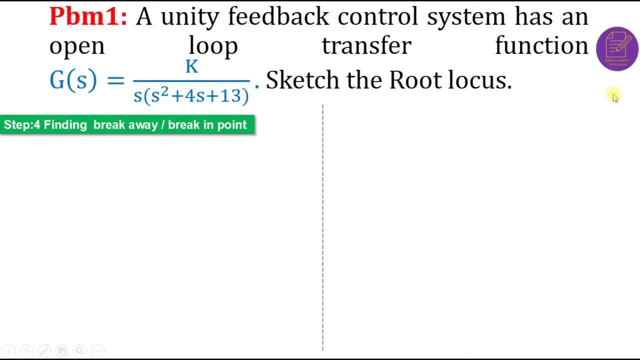 to go for finding the break away, or to go for finding the break away or break-in point. okay, this is very break-in point. okay, this is very break-in point. okay, this is very important. step right, important, step right, important, step right. let's refer our guidebook, rule book, see: 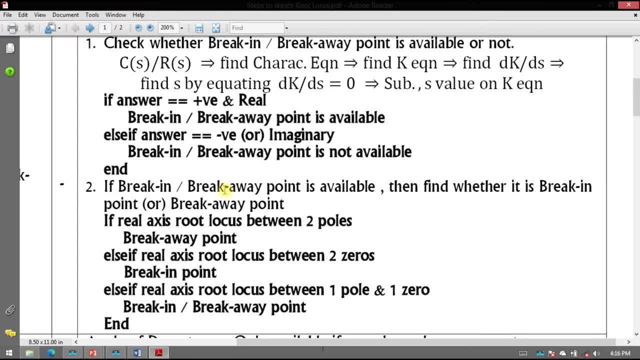 let's refer our guidebook rule book: see. let's refer our guidebook rule book: see. this is our fourth step. quite. this is our fourth step. quite, this is our fourth step. quite difficult to understand, okay. difficult to understand, okay. difficult to understand, okay. let me try our level. first, check whether. 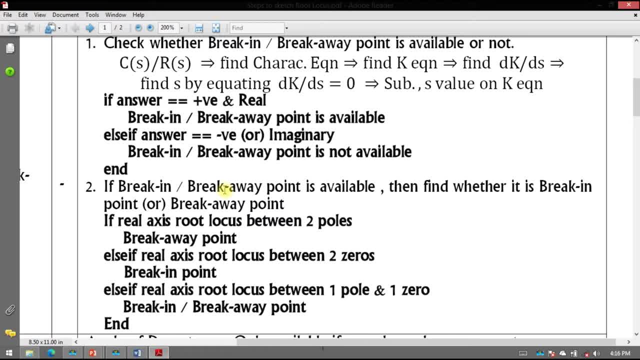 let me try our level first. check whether. let me try our level first. check whether break-in or break-away point is break-in or break-away point is break-in or break-away point is available or not okay, available or not okay, available or not okay? which point is available you need to? 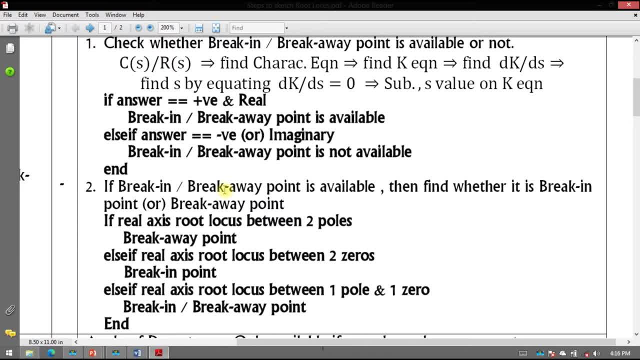 which point is available. you need to. which point is available. you need to identify that first. okay, whether the identify that first, okay. whether the identify that first, okay, whether the system, the problem is having break away system, the problem is having break away system, the problem is having break away point or break in point. okay, that is one. 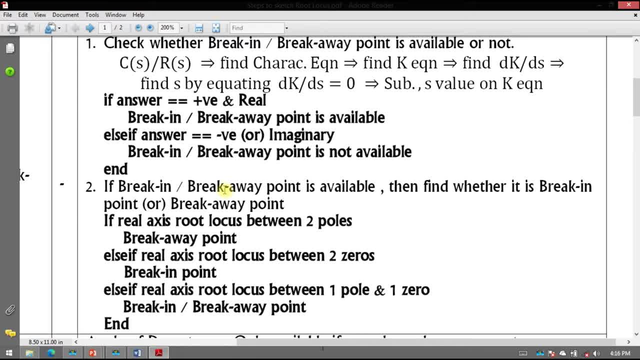 point or break in point. okay, that is one point or break in point, okay, that is one. one can one condition is there, so for one can. one condition is there, so for one can. one condition is there. so for this step we need to, this step we need to. 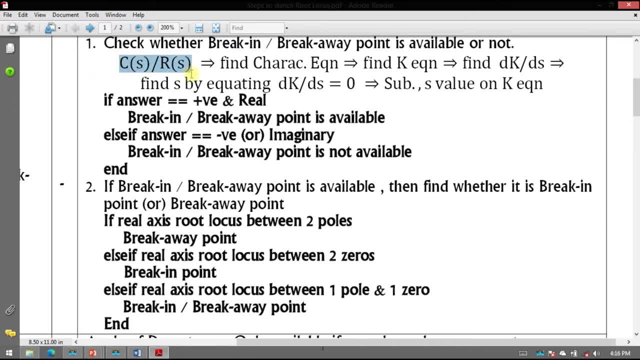 this step. we need to calculate the closed loop response. okay, calculate the closed loop response. okay, calculate the closed loop response. okay, closed loop transfer function. we need to closed loop transfer function. we need to closed loop transfer function. we need to find out. and from the closed loop. 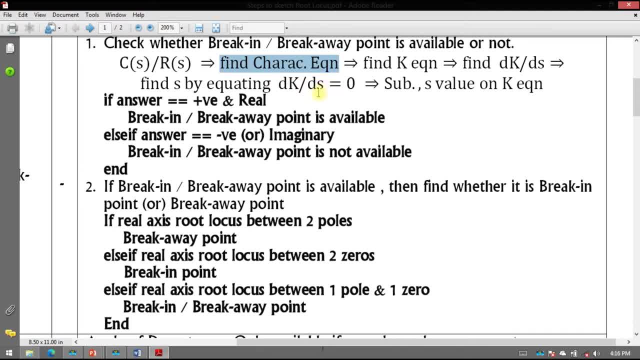 find out and from the closed loop find out. and from the closed loop transfer function itself. we can able to transfer function itself. we can able to transfer function itself. we can able to polynomial of closed loop transfer. polynomial of closed loop transfer. polynomial of closed loop transfer function. okay, so from the closed loop. 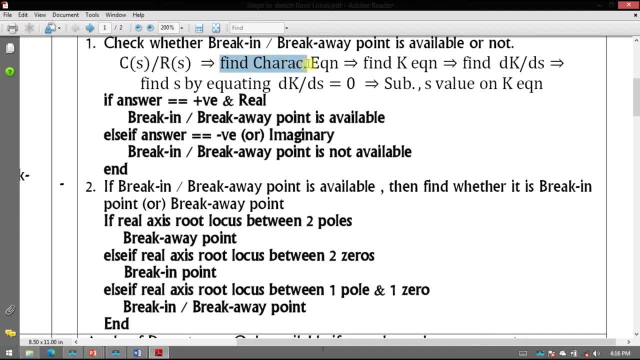 function. okay, so from the closed loop function. okay, so from the closed loop transfer function. take the denominator transfer function. take the denominator transfer function. take the denominator polynomial. that is your characteristic polynomial, that is your characteristic polynomial, that is your characteristic equation, and find out the K value. okay, 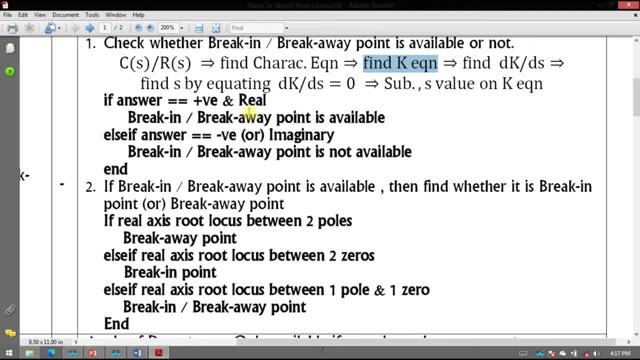 equation and find out the K value. okay, equation and find out the K value. okay, see what you are calculating the closed: see what you are calculating the closed: see what you are calculating the closed loop transfer function. the open loop loop transfer function. the open loop loop transfer function. the open loop transfer function is having some gain. 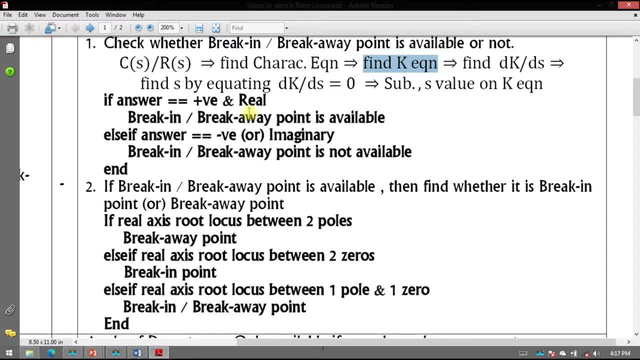 transfer function is having some gain. transfer function is having some gain value called K. so your closed loop value called K, so your closed loop value called K, so your closed loop transfer function, as well as the transfer function, as well as the transfer function, as well as the characteristic equation, will be in the 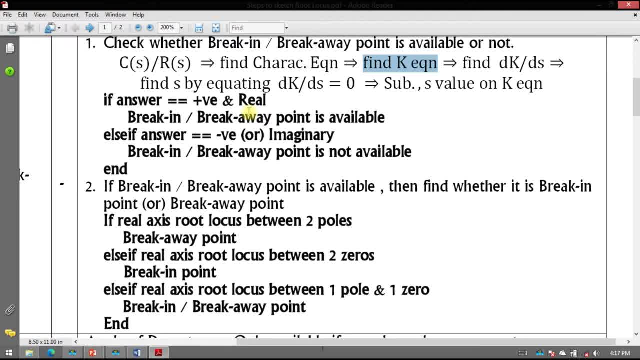 characteristic equation will be in. the characteristic equation will be in the form of K. okay, so K. just keep the K in form of K. okay, so K. just keep the K in form of K. okay, so K. just keep the K in your left hand, left side, and bring all. 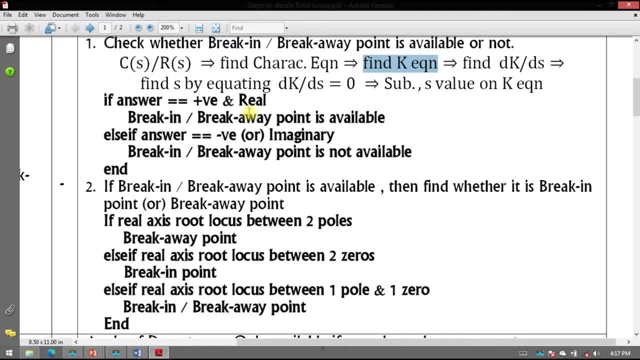 your left hand, left side and bring all your left hand, left side and bring all the terms in your right side. you will the terms in your right side. you will the terms in your right side. you will have the K equation and find out the. have the K equation and find out the. 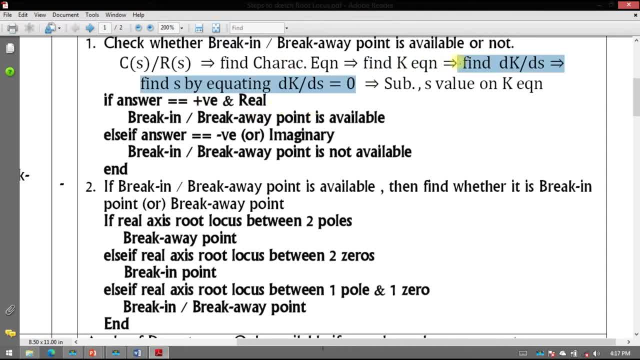 have the K equation and find out the maxima. okay, how to find out the maxima maxima. okay, how to find out the maxima maxima. okay, how to find out the maxima of a particular polynomial you need to, of a particular polynomial you need to. 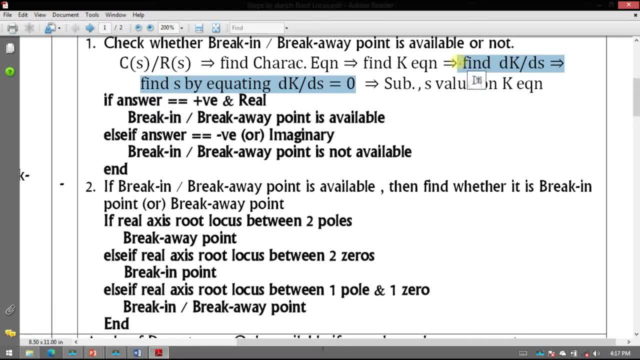 of a particular polynomial. you need to differentiate and you need to compare differentiate and you need to compare differentiate and you need to compare with the zero, I mean equate with the. with the zero, I mean equate with the. with the zero, I mean equate with the zero. okay, so that here the equation is: 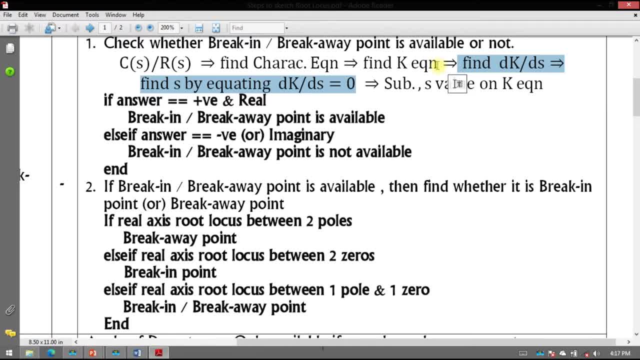 zero. okay, so that here the equation is zero. okay, so that here the equation is with: is with the help of is being with is with the help of is being with is with the help of is being available with the help of our s domain, available with the help of our s domain. 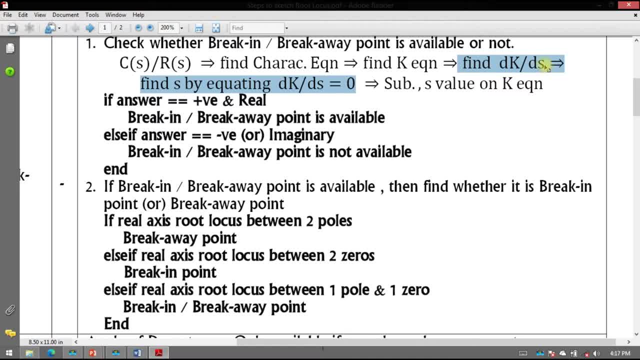 available with the help of our s domain. so differentiate the K equation with. so differentiate the K equation with. so differentiate the K equation with respect to D: yes, sorry with respect to respect to D. yes, sorry with respect to respect to D. yes, sorry with respect to yes. we need to differentiate and then 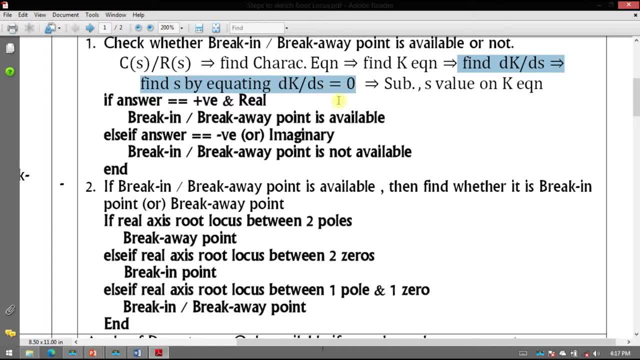 yes, we need to differentiate. and then, yes, we need to differentiate and then equate with the zero. okay, you will have equate with the zero. okay, you will have equate with the zero. okay, you will have one. yes, equation, am I right if you are one? yes, equation, am I right if you are? 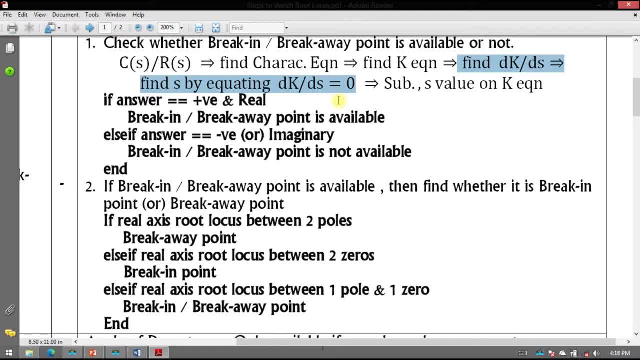 one. yes, equation, am I right? if you are substituting this? if you are, if you are substituting this, if you are, if you are substituting this, if you are, if you are, you are having K equation in terms of s. you are having K equation in terms of s. 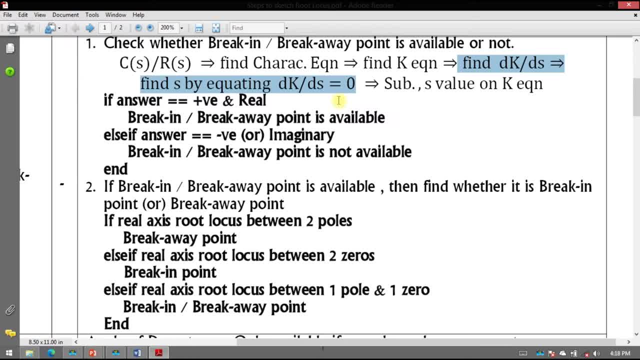 you are having K equation in terms of s, you are differentiating that equation. you are differentiating that equation. you are differentiating that equation with respect to s and you are making with respect to s. and you are making with respect to s and you are making equate with the zero you will get you. 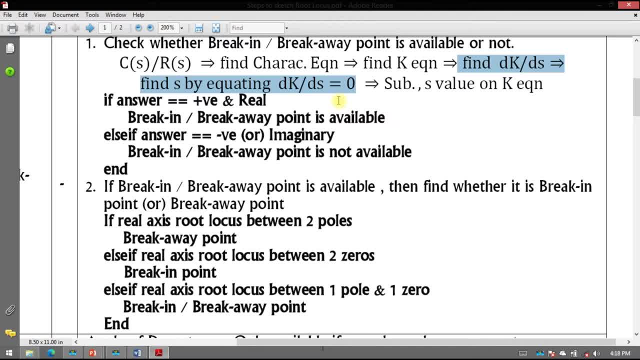 equate with the zero, you will get you. equate with the zero, you will get. you will get some yes value. am I right? so will get some yes value. am I right? so will get some yes value. am I right? so substitute those s values in your K. 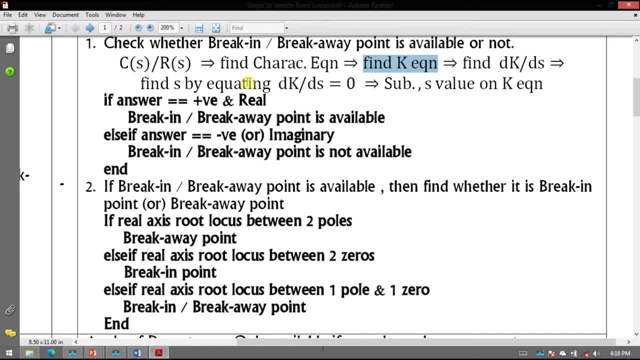 substitute those s values in your K. substitute those s values in your K equation: okay. so if the answer is after equation, okay. so if the answer is after equation, okay. so if the answer is after: substituting the s value we will have. substituting the s value we will have. 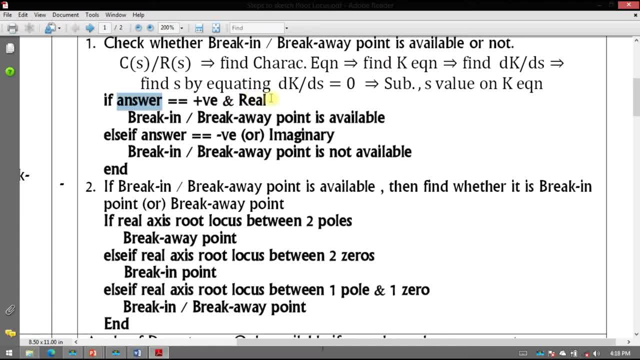 substituting the s value, we will have one K value. am I right if the K value is one K value? am I right if the K value is one K value? am I right if the K value is positive real, that may be one break-in? positive real, that may be one break-in. 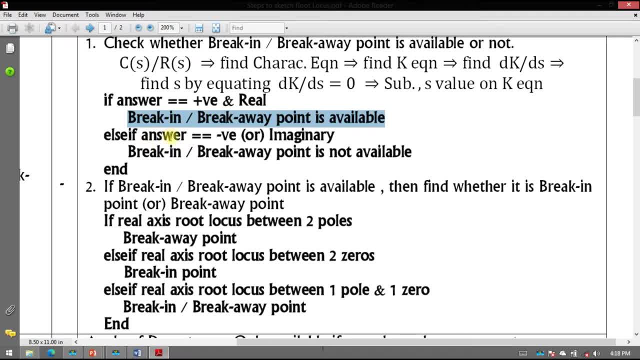 positive real, that may be one break-in or break away point is available else. if or break away point is available else, if or break away point is available else. if it is, it is giving negative our imaginary it is. it is giving negative our imaginary it is. it is giving negative our imaginary value. that is not. there is no. 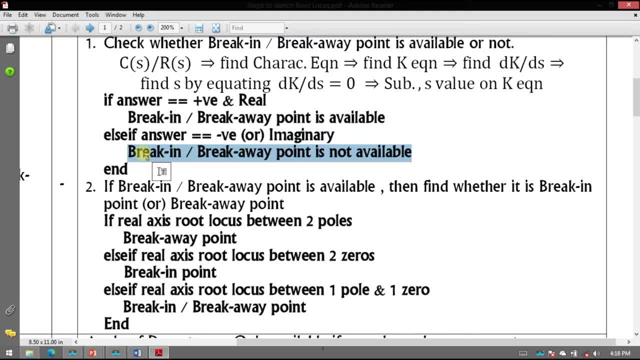 value. that is not. there is no value. that is not. there is no possibility of having break-in or possibility of having break-in or possibility of having break-in or break-away point. okay, in our problem we break-away point. okay, in our problem we break-away point. okay, in our problem we are not having any break-in or break. 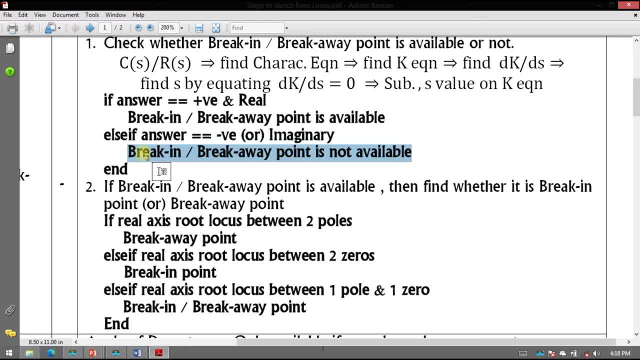 are not having any break-in or break. are not having any break-in or break away point. okay, so let me solve some away point. okay, so, let me solve some away point. okay, so let me solve some more problems in this series or so while. more problems in this series or so while. 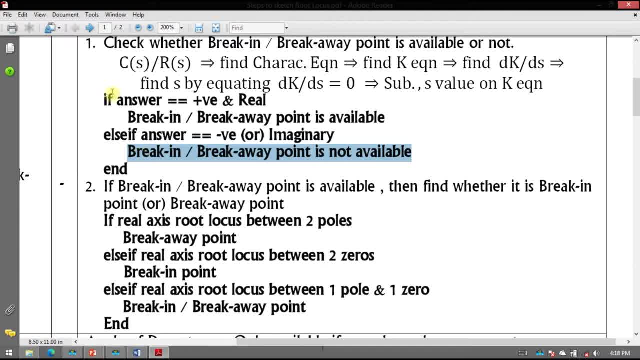 more problems in this series or so, while solving the problem, we will discuss solving the problem. we will discuss solving the problem. we will discuss when the answer is positive and real. when the answer is positive and real. when the answer is positive and real, there may be a break-in or break away. 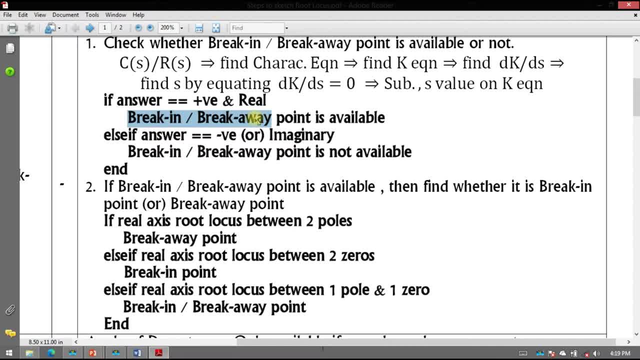 there may be a break-in or break away. there may be a break-in or break away point. okay, how to calculate the break-in point. okay, how to calculate the break-in point. okay, how to calculate the break-in or break away point. how to predict or break away point. how to predict. 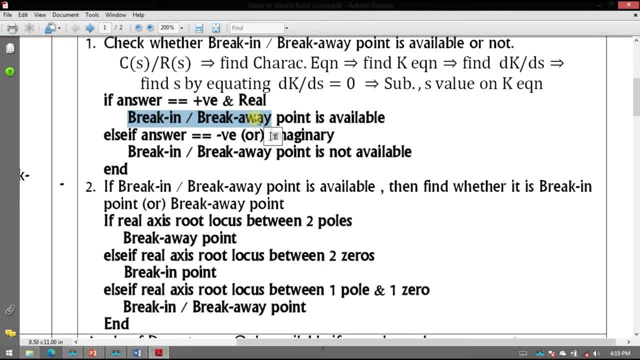 or break away point. how to predict whether the system is having surely any, whether the system is having surely any, whether the system is having surely any. one of the point is the system is having. one of the point is the system is having. one of the point is the system is having okay. further, we need to calculate. 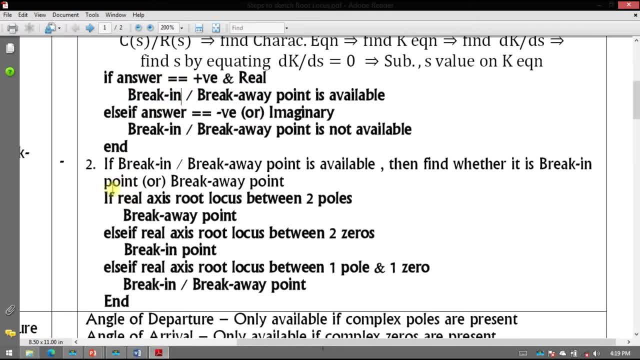 okay, further, we need to calculate. okay, further, we need to calculate whether it is break-in or break away. whether it is break-in or break away. whether it is break-in or break away. that is one more condition is also there. that is one more condition is also there. 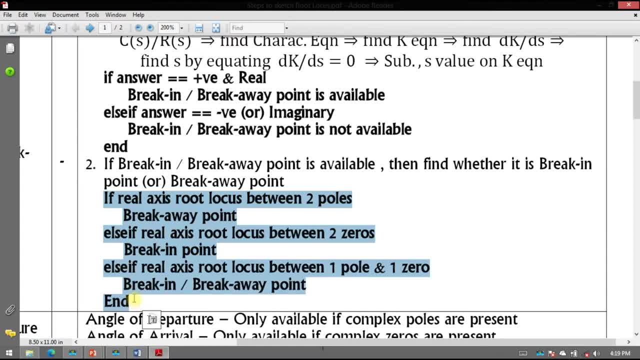 that is, one more condition is also there. so, while solving the problem number two, so, while solving the problem number two, so while solving the problem number two, we we can able to understand this step, we we can able to understand this step, we we can able to understand this step because that problem will have break-in. 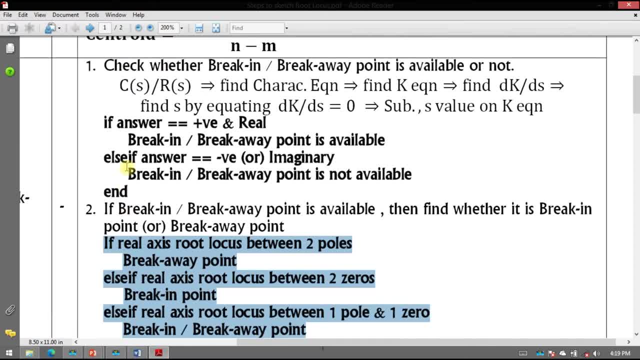 because that problem will have break-in. because that problem will have break-in or break away point. okay. so for this for or break away point. okay, so for this for or break away point. okay. so for this. for our problem we were not having break-in. our problem we were not having break-in. 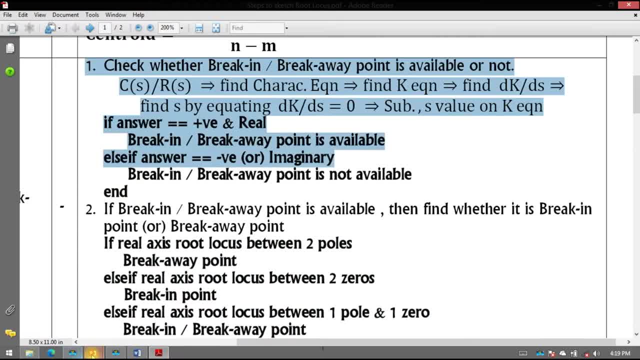 our problem. we were not having break-in or break away point, so we will end up or break away point. so we will end up or break away point. so we will end up with this discussion and we will go and with this discussion and we will go and. 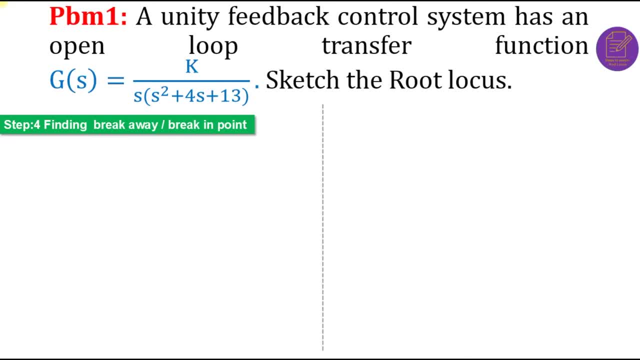 with this discussion and we will go and solve the problem here. okay, so we know, solve the problem here. okay, so we know, solve the problem here. okay, so we know that sorry we are we. we know that the that sorry we are we. we know that the that sorry we are we. we know that the closed-loop transfer function is G of s. 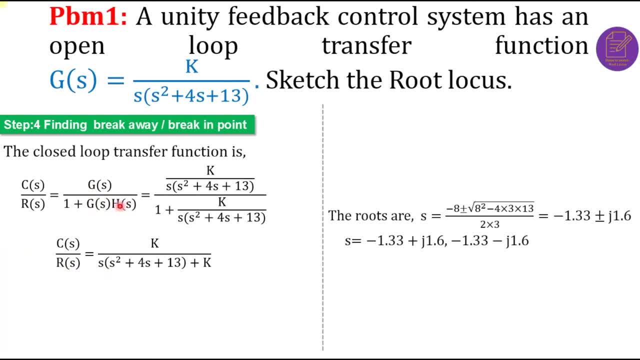 closed-loop transfer function is G of s. closed-loop transfer function is G of s divided by 1 plus G of s into H of s. divided by 1 plus G of s into H of s. divided by 1 plus G of s into H of s. you may know that. okay, just I am taking. 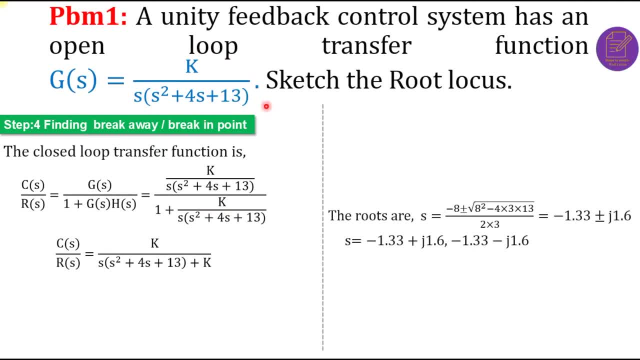 you may know that, okay, just I am taking. you may know that, okay, just I am taking. this is, this is this is G of s and H of this is: this is this is G of s and H of this is: this is: this is G of s and H of s is 1. because the unity feedback system. 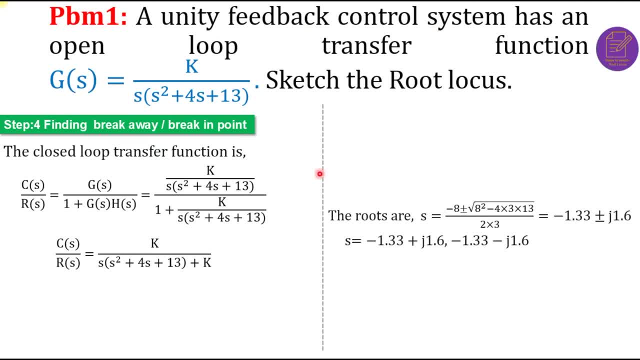 is 1 because the unity feedback system is 1, because the unity feedback system, the system statement itself having unity, the system statement itself having unity, the system statement itself having unity feedback system. so H of s is equal to 1 feedback system, so H of s is equal to 1. 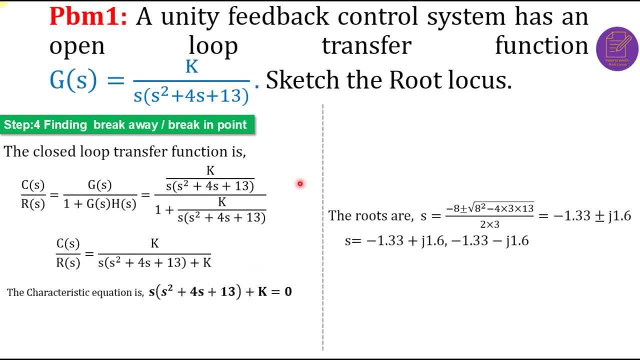 feedback system. so H of s is equal to 1. so this is the closed-loop transfer. so this is the closed-loop transfer. so this is the closed-loop transfer function. we know that the closed-loop function, we know that the closed-loop function, we know that the closed-loop transfer function is having characteristic. 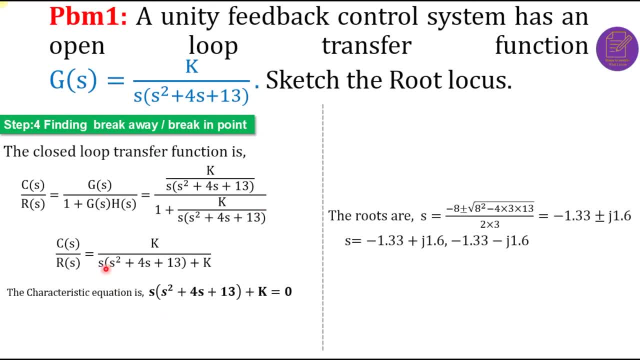 transfer function is having characteristic transfer function is having characteristic equation, which means the denominator equation, which means the denominator equation, which means the denominator polynomial is called as characteristic polynomial is called as characteristic polynomial is called as characteristic equation. so I am going to take the equation, so I am going to take the. 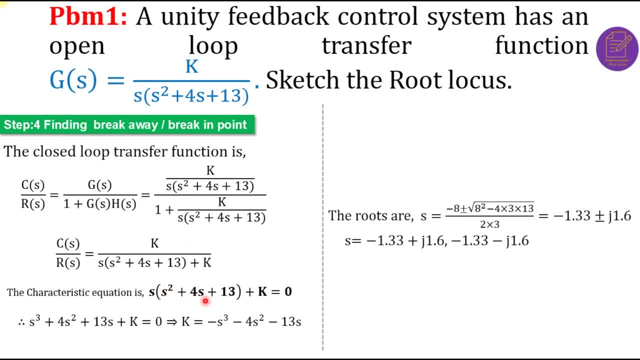 equation. so I am going to take the characteristic equation and equate with characteristic equation and equate with characteristic equation and equate with the 0. I am getting one yes. equation like the 0. I am getting one. yes. equation like the 0. I am getting one. yes. equation like s. square is Q plus 4 square plus 13 s. 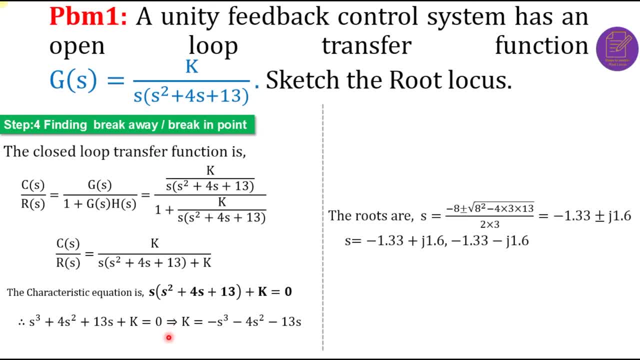 s square is Q plus 4 square plus 13 s s square is Q plus 4 square plus 13 s plus K equal to 0, and we know that we plus K equal to 0, and we know that we plus K equal to 0, and we know that we need to find out the K value. I mean K. 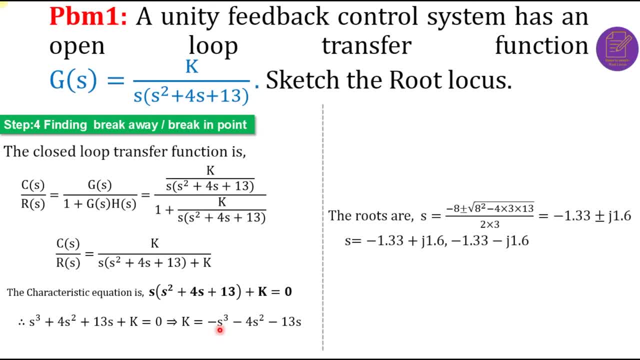 need to find out the K value. I mean K. need to find out the K value. I mean K- equation. we need to find out K equal to equation. we need to find out K equal to equation. we need to find out K equal to minus s, 3, minus 4 s square minus 13. yes, 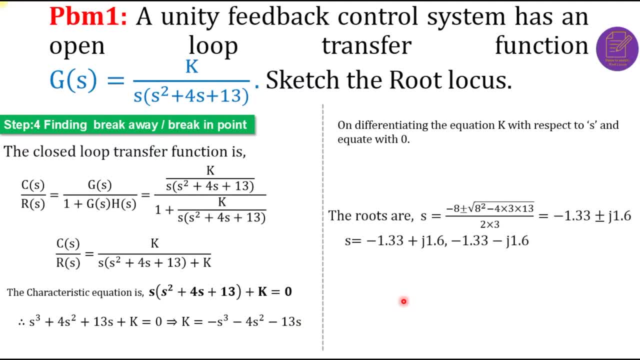 minus s 3 minus 4 s square minus 13: yes. minus s 3 minus 4 s square minus 13: yes, and then on differentiating, differentiating, and then on differentiating, differentiating, and then on differentiating, differentiating the equation K, with respect. 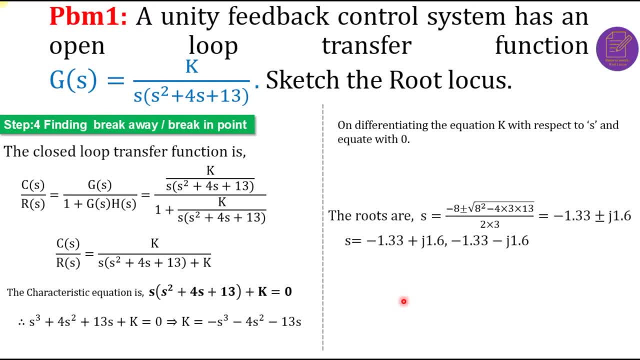 the equation K with respect. the equation K with respect to yes and equate with the 0. this is the to yes and equate with the 0. this is the to yes and equate with the 0. this is the principle of finding the maxima right. so 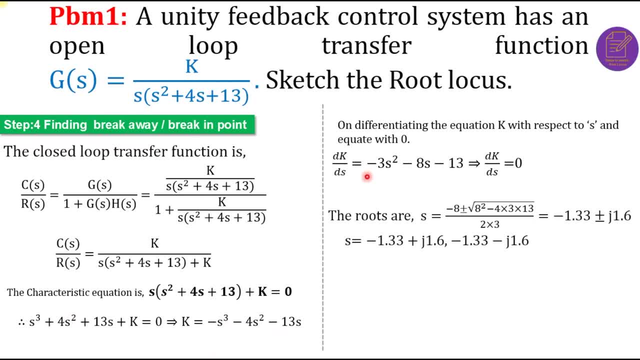 principle of finding the maxima right. so, principle of finding the maxima right. so I am differentiating this equation with. I am differentiating this equation with. I am differentiating this equation with respect to s. I am getting this value. respect to s: I am getting this value. 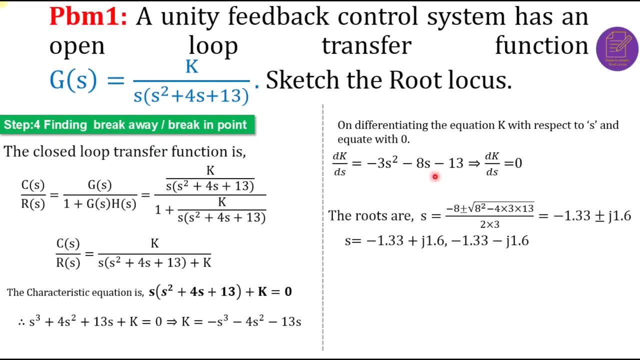 respect to s, I am getting this value minus 3 s square minus 8 s minus 13, and minus 3 s square minus 8 s minus 13, and minus 3 s square minus 8 s minus 13, and- and I'm going to equate the equation- 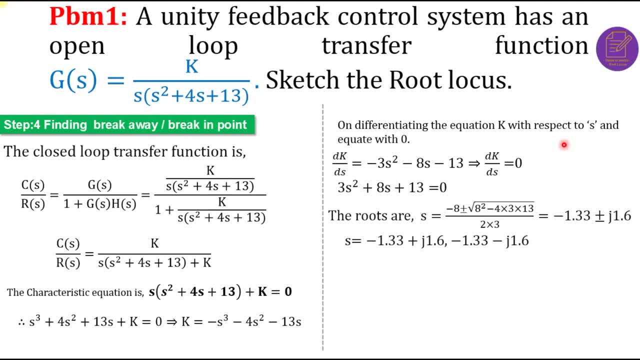 and I'm going to equate the equation. and I'm going to equate the equation with respect to: with equal to 0. okay. so, with respect to with equal to 0. okay. so, with respect to with equal to 0. okay. so 3 s square plus 8 s plus 13, okay, I'm. 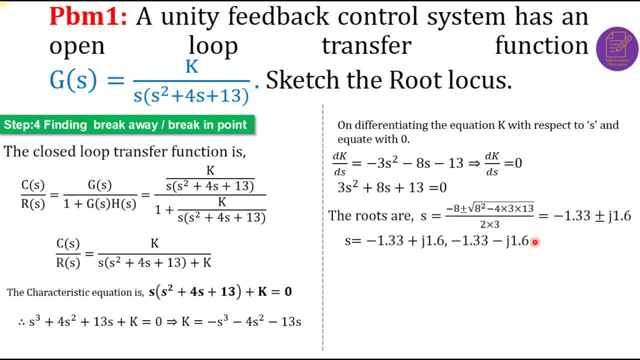 3 s square plus 8 s plus 13. okay, I'm 3 s square plus 8 s plus 13. okay, I'm going to find the root of this equation. going to find the root of this equation. going to find the root of this equation and getting these roots, I mean minus 1.33. 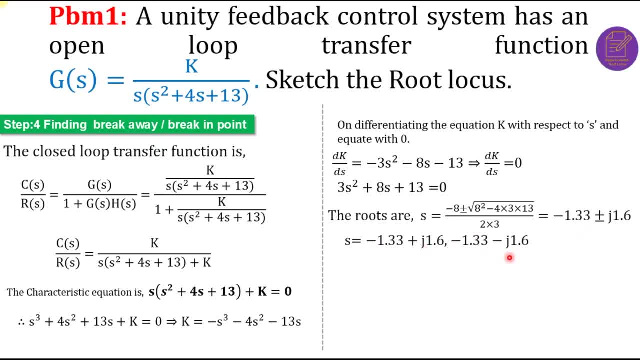 and getting these roots, I mean minus 1.33. and getting these roots, I mean minus 1.33, plus J 1.6 minus 1.33 minus J 1.6. okay. plus J 1.6 minus 1.33 minus J 1.6- okay. 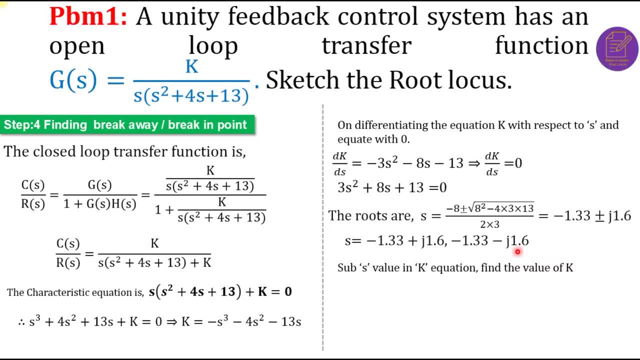 plus J, 1.6. okay, so what we have to do is we need to substitute the s value in. so what we have to do is we need to substitute the s value in. so what we have to do is we need to substitute the s value in our K equation. okay, this is K equation. 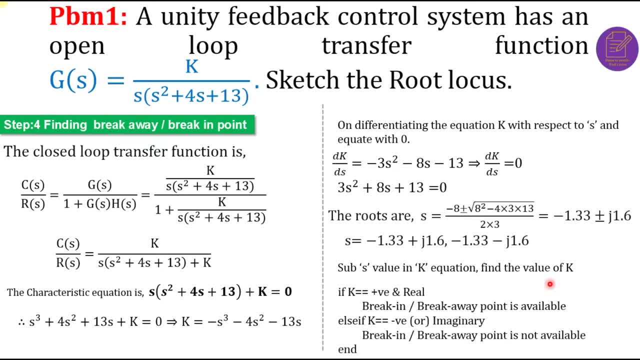 our K equation. okay, this is K equation. our K equation: okay, this is K equation. am I right? yeah, and find the K value. so am I right? yeah, and find the K value. so am I right? yeah, and find the K value. so, based upon the K value, we told right K. 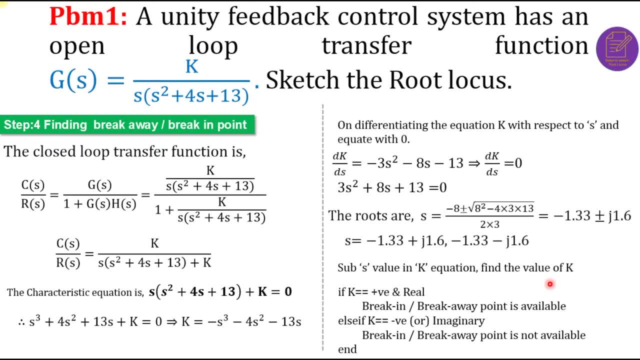 based upon the K value, we told right K. based upon the K value, we told right K is equal to positive and real value is equal to positive and real value is equal to positive. and real value means there is one point is available, means there is one point is available. 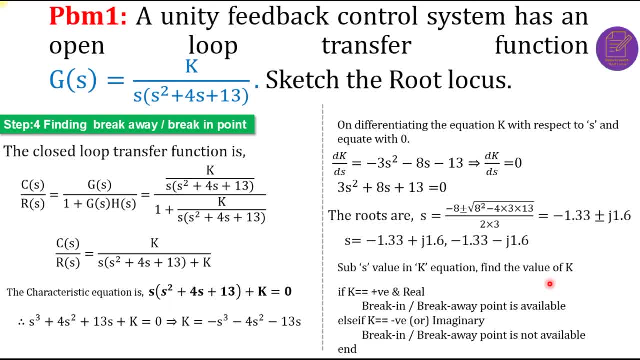 means there is one point is available. okay, either it may be break-in or break. okay, either it may be break-in or break. okay, either it may be break-in or break away part, but else if if it is having away part, but else if if it is having. 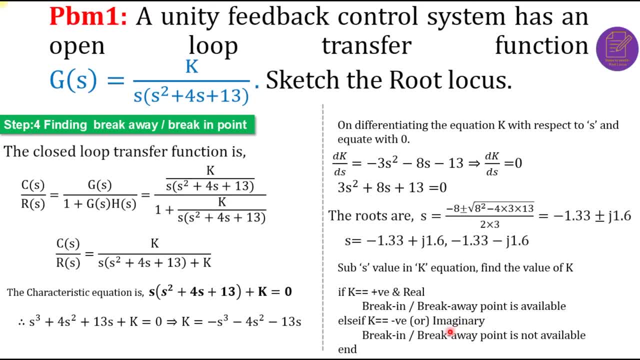 away part, but else, if if it is having negative or imaginary value means it is negative or imaginary value means it is negative or imaginary value means it is, it is giving negative or imaginary, it is giving negative or imaginary, it is giving negative or imaginary values means no need to worry about it. we 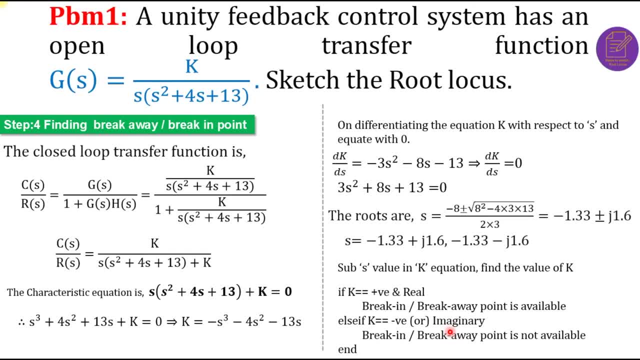 values means no need to worry about it. we values means no need to worry about it. we are not having either break-in or are not having either break-in or are not having either break-in or break away part. okay, so in this equation, we break away part. okay, so in this equation, we 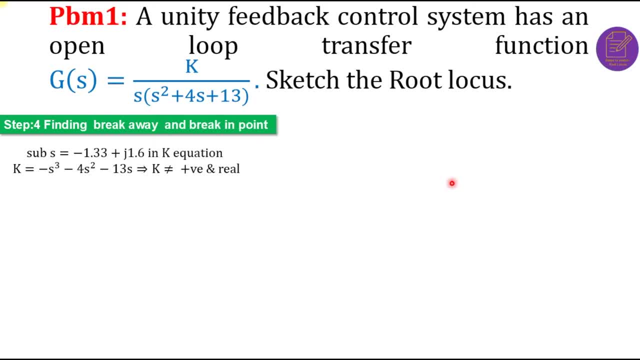 break away part. okay, so in this equation, we are getting, we are having two s values, are getting, we are having two s values are getting, we are having two s values. am I right? so first I am substituting the. am I right? so first I am substituting the. 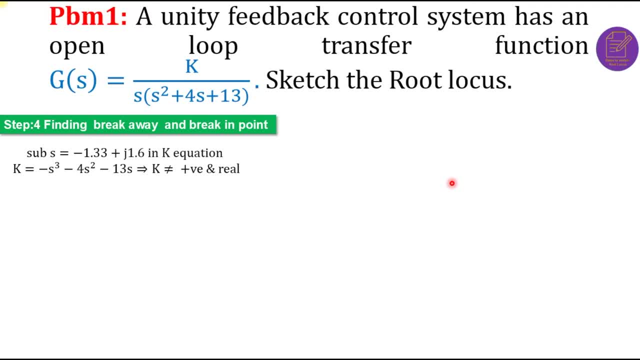 am I right? so first I am substituting the value of minus 1.33 plus J 1.6 in our value of minus 1.33 plus J 1.6 in our value of minus 1.33 plus J 1.6 in our K equation. this is K equation correct as a. 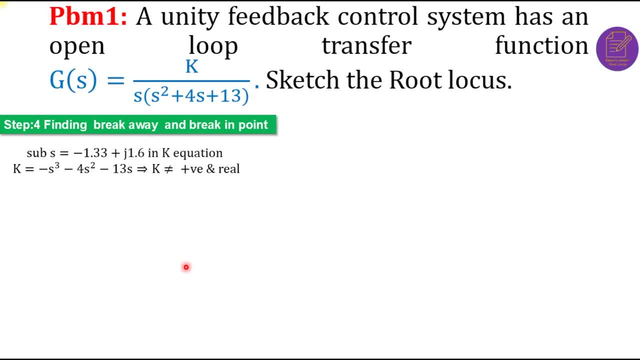 K equation. this is K equation correct as a K equation. this is K equation correct. as a result, our K value will have only result. our K value will have only result. our K value will have only positive, will not have sorry will not. positive will not have, sorry will not. 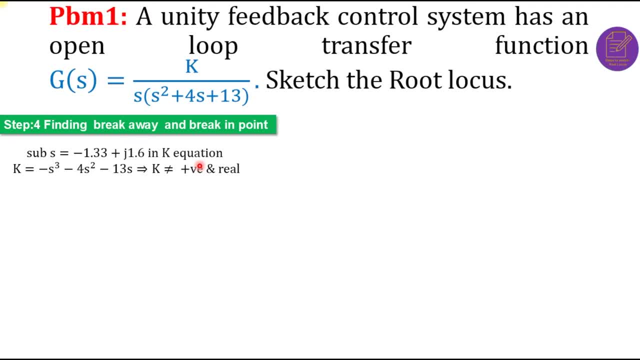 positive will not have, sorry, will not have positive and real axis. and you make have positive and real axis and you make have positive and real axis and you make this calculation in your calculator and this calculation in your calculator and this calculation in your calculator and also for these values, also the K value. 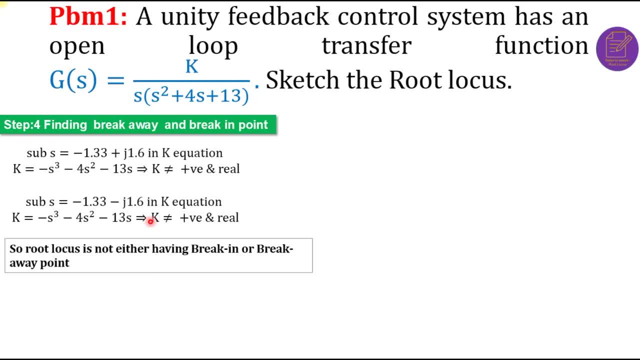 also for these values also, the K value, also for these values also, the K value will not give any positive and real will not give any positive and real will not give any positive and real value, so that we can say that root locus value, so that we can say that root locus. 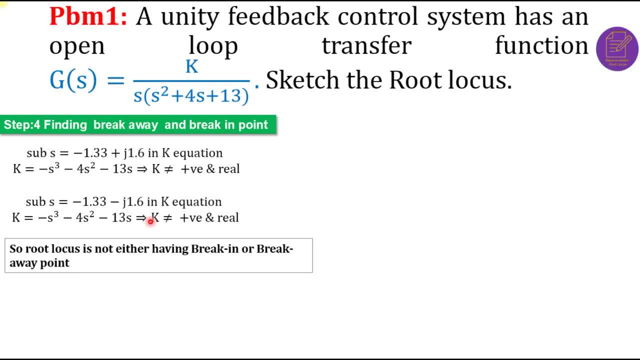 value, so that we can say that root locus is not, either having break-in or break is not. either having break-in or break is not, either having break-in or break away point. so in our problem we are not away point. so in our problem we are not. 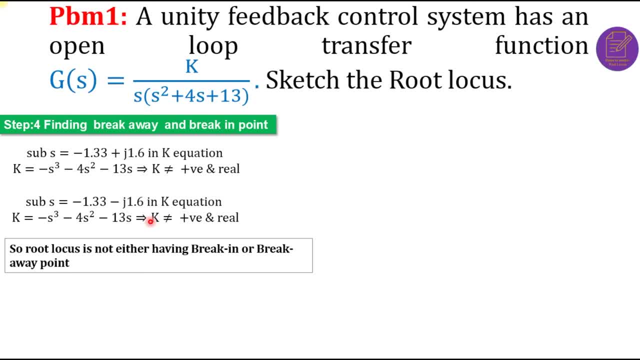 away point. so in our problem we are not having any break-in or break-away point. having any break-in or break-away point. having any break-in or break-away point? okay. then fifth one, so this step is okay. then fifth one, so this step is okay. then fifth one. so this step is finding angle of departure, our angle of. 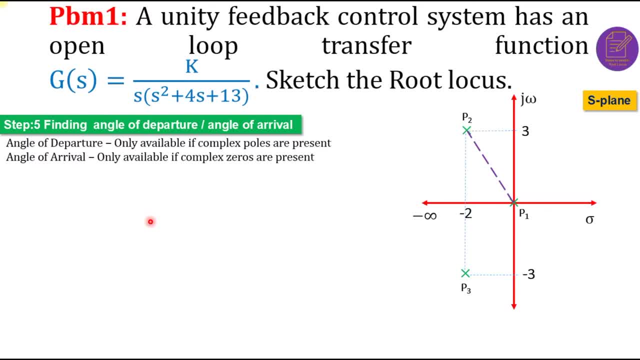 finding angle of departure. our angle of finding angle of departure, our angle of arrival. okay so, angle of departure is arrival. okay so, angle of departure is arrival. okay, so, angle of departure is nothing. but this is an angle, only nothing. but this is an angle, only nothing. but this is an angle only available if the complex poles are. 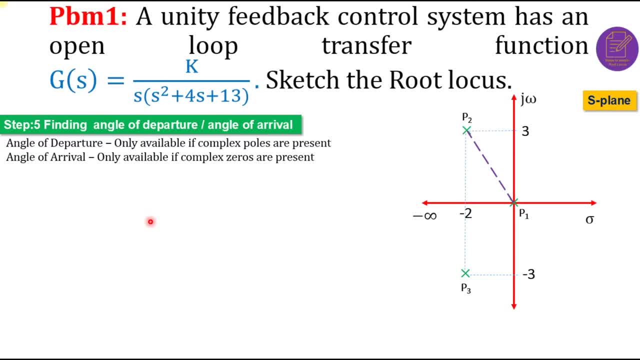 available. if the complex poles are available. if the complex poles are present, okay in which? if the system is present, okay in which. if the system is present, okay in which. if the system is having complex poles, you need to having complex poles, you need to having complex poles, you need to calculate and love departure if the 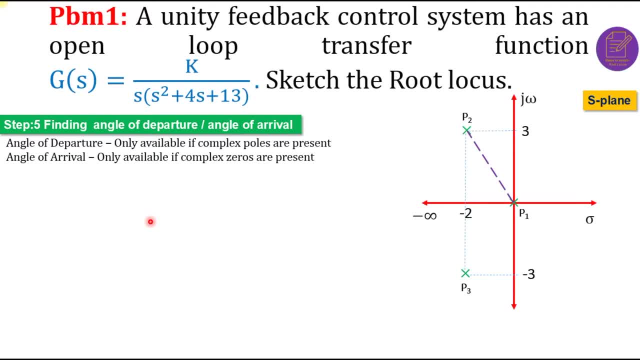 calculate and love departure. if the calculate and love departure, if the system is having and complex zeros, the system is having and complex zeros, the system is having and complex zeros. the system is having you need to calculate system is having you need to calculate. system is having you need to calculate angle of arrival. okay, so both, if the 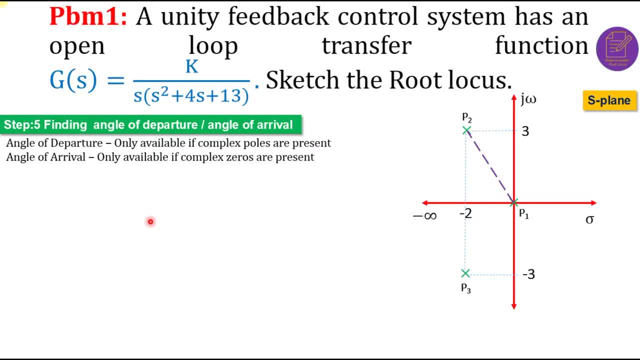 angle of arrival okay, so both if the angle of arrival okay, so both. if the system is having both complex poles and system is having both complex poles and system is having both complex poles. and complex zero means you need to calculate. complex zero means you need to calculate. 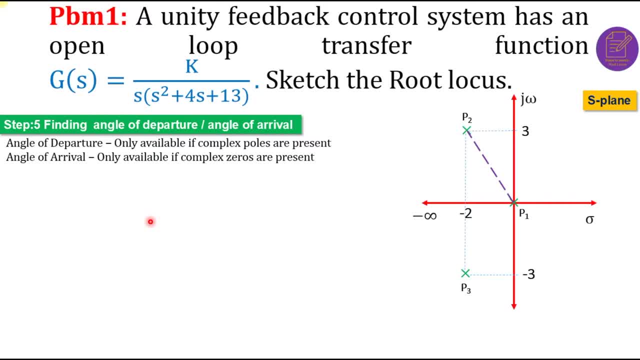 complex. zero means you need to calculate both a of D to the angle of departure, both a of D to the angle of departure, both a of D to the angle of departure and angle of arrival. okay, so in our and angle of arrival. okay, so in our and angle of arrival. okay, so in our system we are having only complex poles. 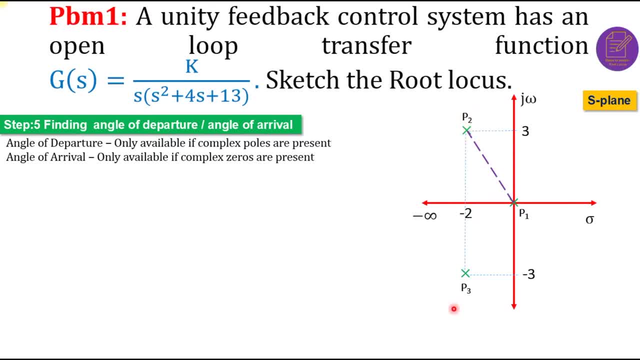 system. we are having only complex poles system. we are having only complex poles ever at P 2 and P 3. this is somewhat ever at P 2 and P 3. this is somewhat ever at P 2 and P 3. this is somewhat two complex poles we are having okay. so 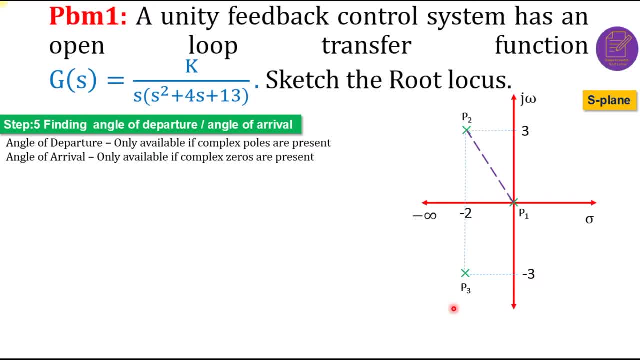 two complex poles we are having, okay. so two complex poles we are having, okay. so we are having, only we need to, only we are having, only we need to, only we are having, only we need to only calculate a OD, the root locus is only calculate a OD, the root locus is only. 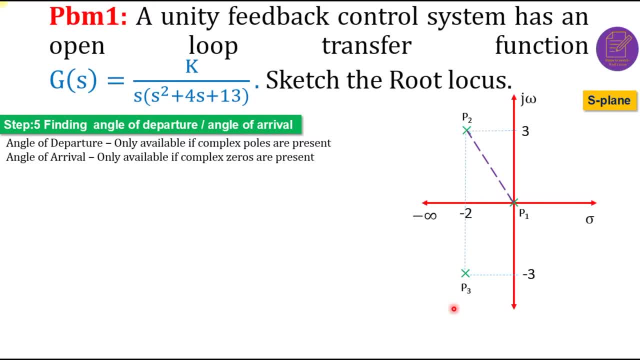 calculate a OD. the root locus is only having angle of departure. so that we can having angle of departure, so that we can having angle of departure, so that we can proceed with the angle of departure, proceed with the angle of departure, proceed with the angle of departure calculation. okay, the next angle of 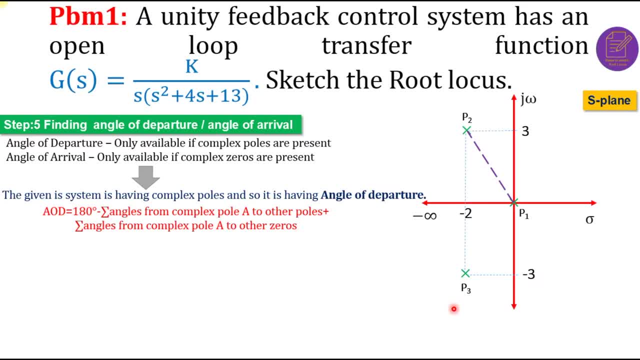 calculation. okay, the next angle of calculation, okay, the next angle of departure is having one particular departure, is having one particular departure is having one particular formula. okay, I think for this step also formula okay. I think for this step also formula okay. I think for this step also, we no need to go for our rule book, okay. 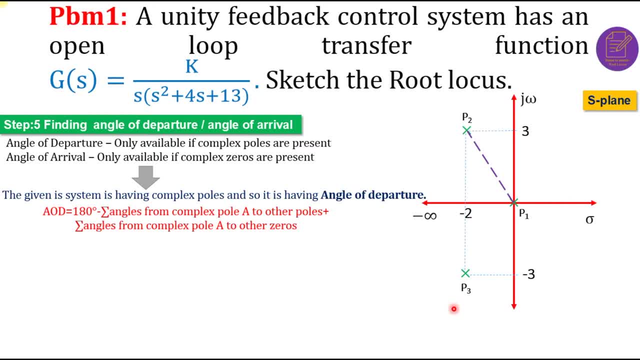 we no need to go for our rule book. okay, we no need to go for our rule book. okay, all the simple. all the problems are all, all the simple. all the problems are all, all the simple. all the problems are all not having break in a breaker point and 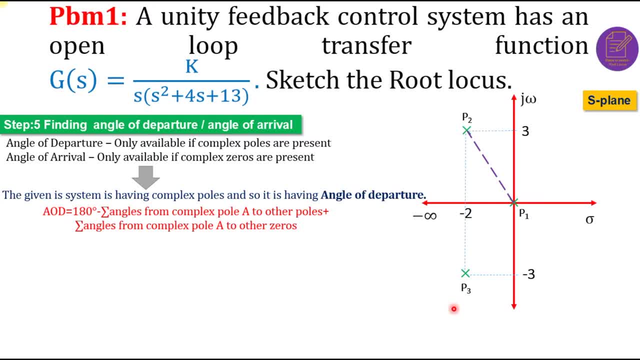 not having break in a breaker point and not having break in a breaker point, and also this is having only two number of. also this is having only two number of. also this is having only two number of complex poles. okay, the AOD calculation. complex poles. okay, the AOD calculation. 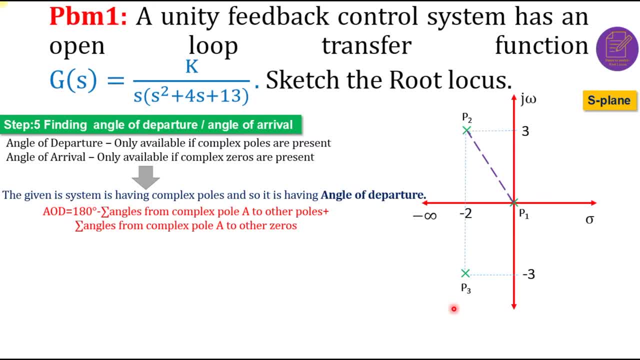 complex poles. okay, the AOD calculation will be very simple, but if you are going will be very simple. but if you are going will be very simple. but if you are going to our rule book, that the diagrams and to our rule book, that the diagrams and to our rule book, that the diagrams and the formulas which is given present in 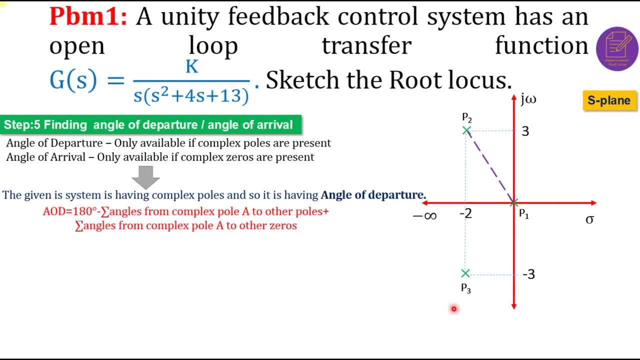 the formulas which is given present in the formulas which is given present in that particular section is somewhat large. that particular section is somewhat large. that particular section is somewhat large. okay, so for this basic level problem. okay, so for this basic level problem. okay, so for this basic level problem, no need to go for the rule book for step. 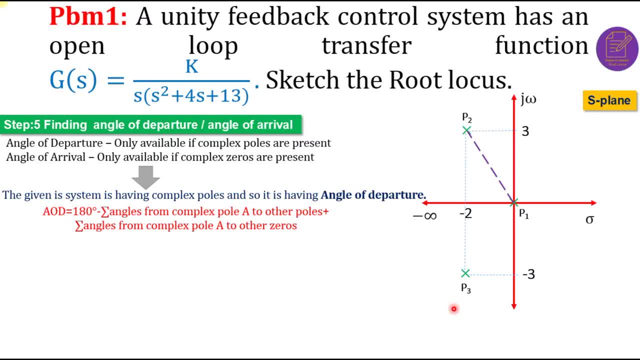 no need to go for the rule book for step. no need to go for the rule book for step number 5. okay, we can complete with this number 5. okay, we can complete with this number 5. okay, we can complete with this slide itself. okay, let's solve. AOD is. 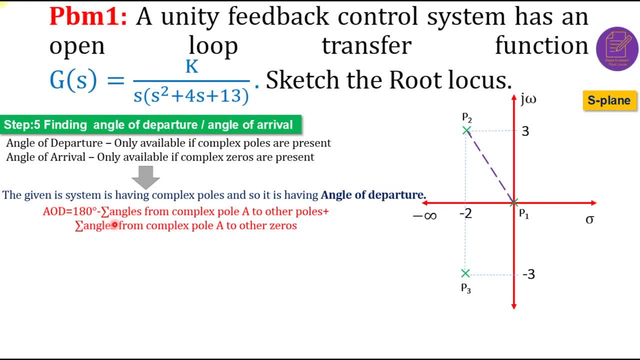 slide itself. okay, let's solve. AOD is slide itself. okay, let's solve. AOD is equal to 180 degree minus sum of angles equal to 180 degree minus sum of angles equal to 180 degree minus sum of angles from complex poles a to other poles. 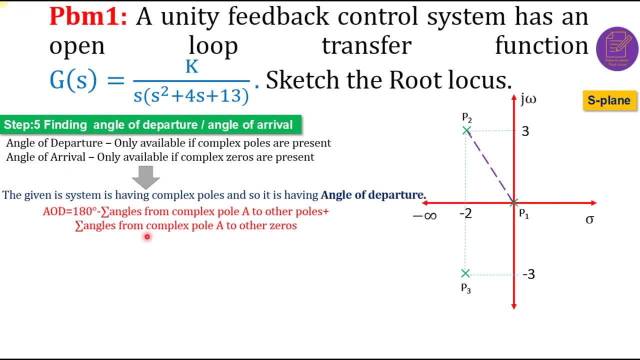 from complex poles a to other poles, from complex poles a to other poles, plus sum of angles from complex pole to plus sum of angles from complex pole to plus sum of angles from complex pole to other zeros: okay, see, this is the general. other zeros: okay, see, this is the general. 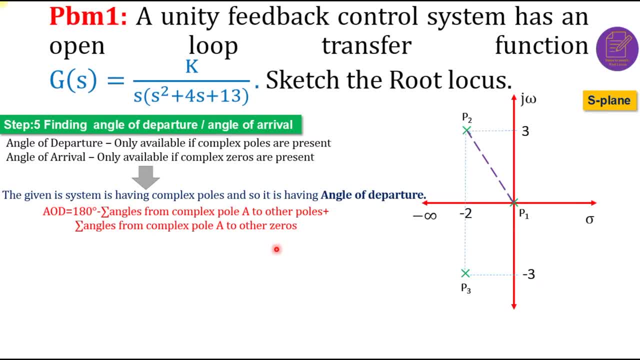 other zeros. okay, see, this is the general formula for angle of departure, right? so formula for angle of departure, right, so formula for angle of departure, right? so what we have to do is we need to find what we have to do is we need to find what we have to do is we need to find out the angles from complex pole there. 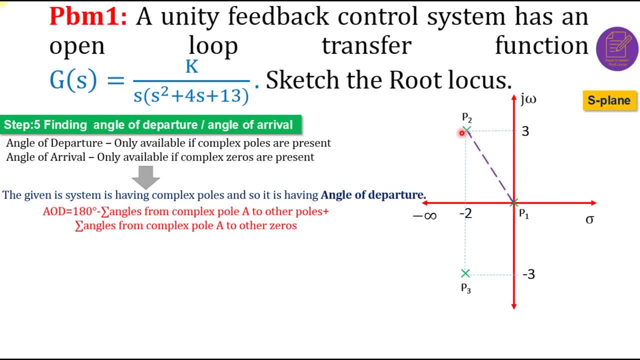 out the angles from complex pole. there out the angles from complex pole. there are two complex poles. here, am I right? are two complex poles? here, am I right? are two complex poles? here am I right, there are two complex pole. this is first. there are two complex pole. this is first. 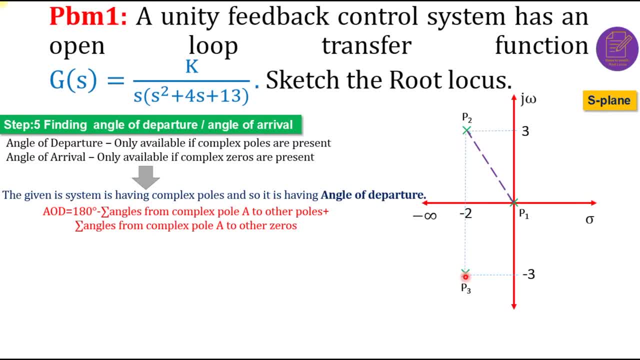 there are two complex pole. this is first complex pole. this is the conjugate of complex pole. this is the conjugate of complex pole. this is the conjugate of that complex pole. anyway, it is in second, that complex pole, anyway. it is in second, that complex pole, anyway, it is in second conjugate pole. okay, second complex pole. 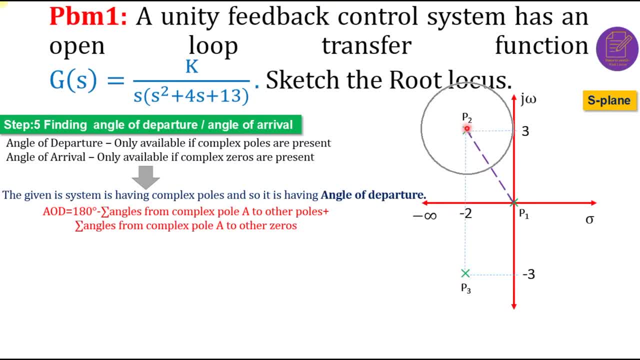 conjugate pole: okay. second complex pole: conjugate pole: okay. second complex pole: sorry, okay. so what you have to do is we sorry, okay. so what you have to do is we sorry, okay. so what you have to do is we need to find out the angle from this. 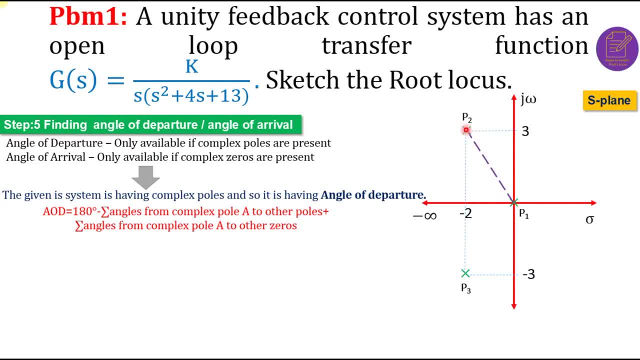 need to find out the angle from this, need to find out the angle from this complex pole to other pole, P 1, and the complex pole to other pole, P 1, and the complex pole to other pole, P 1, and the angle between P 2 to P 3. likewise we 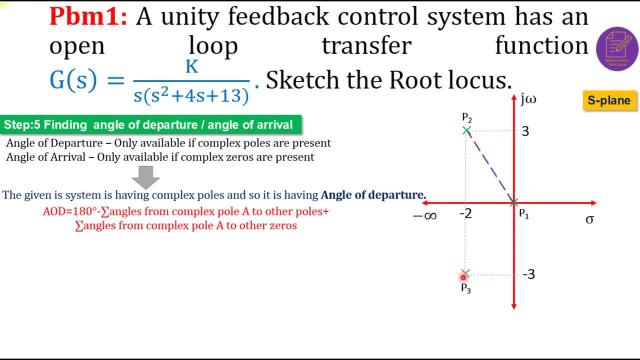 angle between P 2 to P 3. likewise we angle between P 2 to P 3, likewise we have to find out the complex pole, to have to find out the complex pole, to have to find out the complex pole to other pole angle. and we need to sum of: 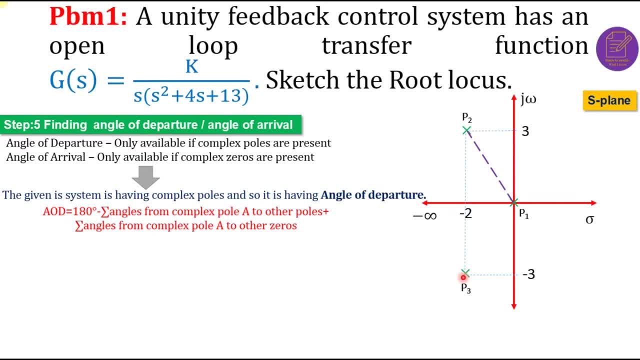 other pole angle and we need to sum of other pole angle and we need to sum of all, some, all of them, and we need to all some, all of them, and we need to all some, all of them, and we need to subtract from 180 degree. this is the. 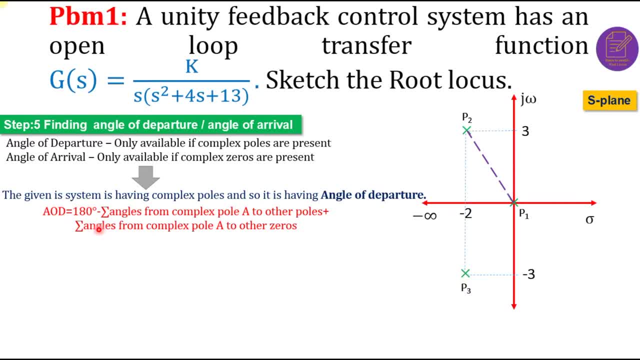 subtract from 180 degree. this is the subtract from 180 degree. this is the concept and also we need to. we need to concept and also we need to, we need to concept and also we need to. we need to sum the angles of complex pole to other. 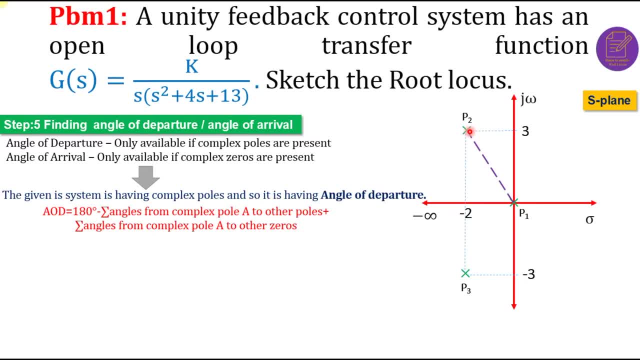 sum the angles of complex pole to other. sum the angles of complex pole to other. zeros in our problem there is no zeros. zeros in our problem there is no zeros. zeros in our problem there is no. zeros are available, so we don't worry about. are available, so we don't worry about. 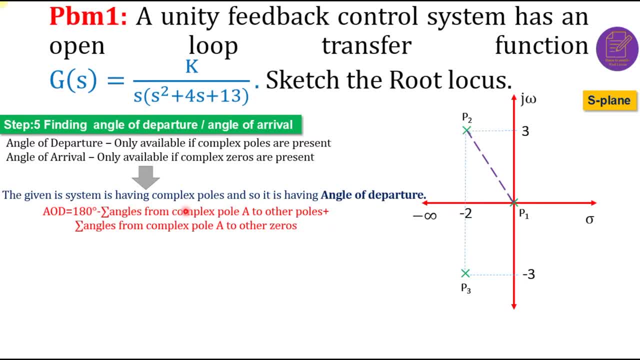 are available, so we don't worry about this third section. okay, we need to only this third section. okay, we need to only this third section. okay, we need to only calculate these values. okay, so angle of calculate these values. okay, so angle of calculate these values. okay. so angle of departure with respect to 0.2. I mean. 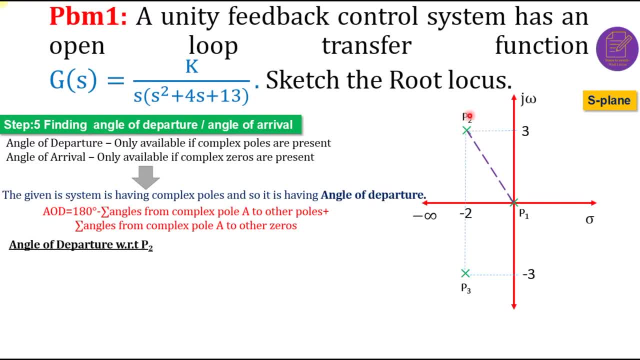 departure with respect to 0.2. I mean departure with respect to 0.2. I mean pole 2 are able to get it. this is pole. pole 2 are able to get it. this is pole: pole 2 are able to get it. this is pole 2 with respect to pole 2. we are initially 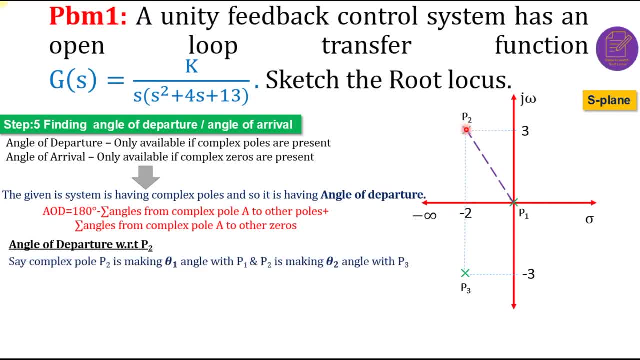 2 with respect to pole 2. we are initially 2 with respect to pole 2. we are initially finding the angle of departure. okay, finding the angle of departure- okay, finding the angle of departure, okay, right. so so we know that angle of right. so so we know that angle of. 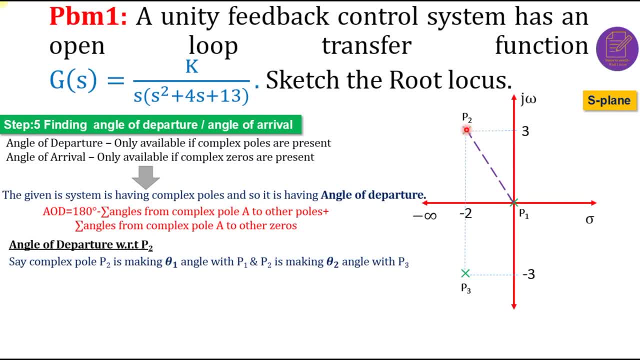 right. so so we know that angle of departure or arrival. am I right? departure, departure or arrival? am I right? departure, departure or arrival? am I right? departure means from that point itself, the means from that point itself, the means from that point itself, the root locus, start traveling, okay. angle of. 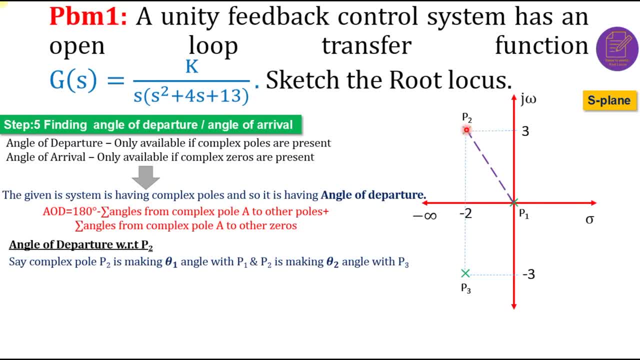 root locus start traveling okay. angle of root locus: start traveling okay. angle of arrival means to that point, only the arrival means to that point, only the arrival means, to that point, only the branch. one branch of the root locus is branch one branch of the root locus is: 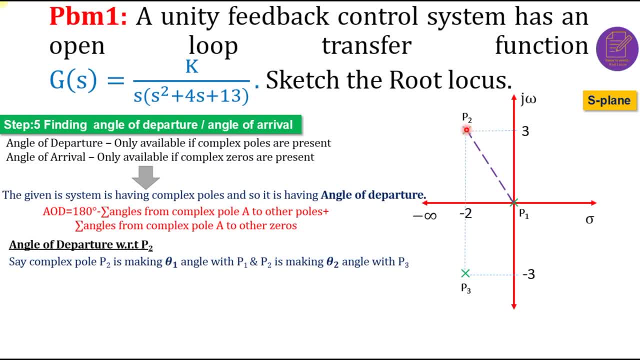 branch, one branch of the root locus, is reaching the ending point. okay so, angle reaching the ending point. okay so, angle reaching the ending point. okay so, angle of departure: we are calculating now, so of departure. we are calculating now, so of departure. we are calculating now. so say, the pole P 2 is making theta 1 angle. 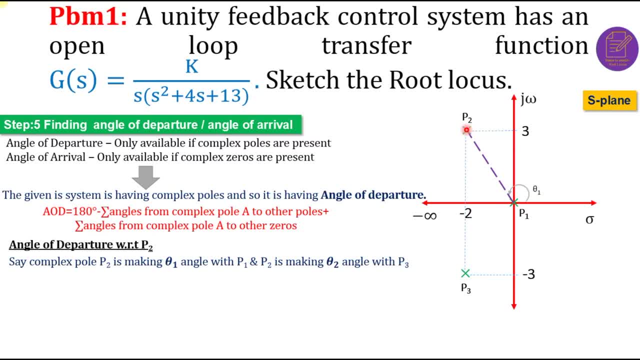 say the pole P 2 is making theta 1 angle. say the pole P 2 is making theta 1 angle with P 1: okay, are able to get it. P 2 with P 1: okay, are able to get it. P 2 with P 1: okay, are able to get it. P 2 complex pole is making theta 1 angle. 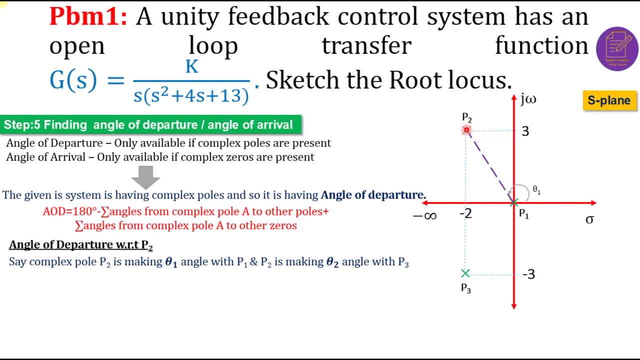 complex pole is making theta 1 angle. complex pole is making theta 1 angle with P 1 and P 2 is making did theta 2 with P 1 and P 2 is making did theta 2 with P 1 and P 2 is making did theta 2 angle with P 3? this is an assumption. 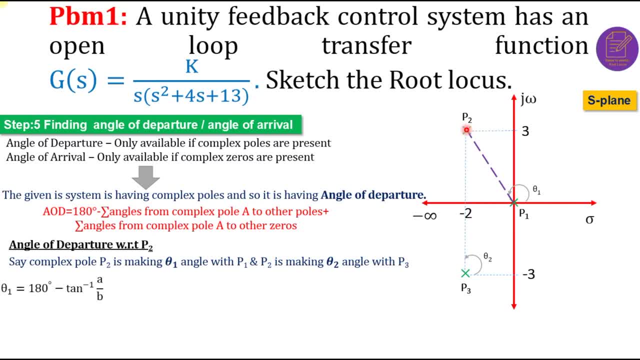 okay, so we we need to. theta 1 can be okay, so we we need to. theta 1 can be okay, so we we need to. theta 1 can be calculated with the help of this formula. calculated with the help of this formula, calculated with the help of this formula. time: 180 degree minus tan, inverse of a. 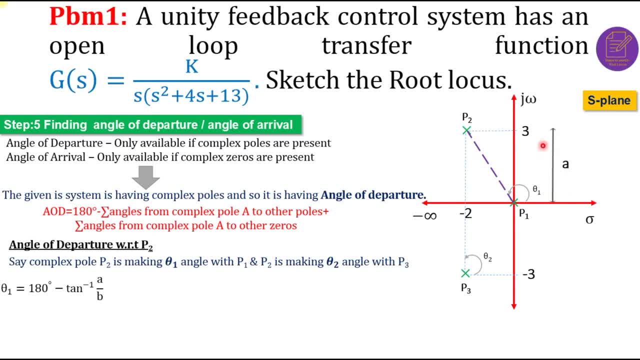 time: 180 degree minus tan. inverse of a time: 180 degree minus tan, inverse of a. by B a is nothing but this imaginary by B a is nothing but this imaginary by B a is nothing but this imaginary axis, this height of this rectangle and axis, this height of this rectangle and. 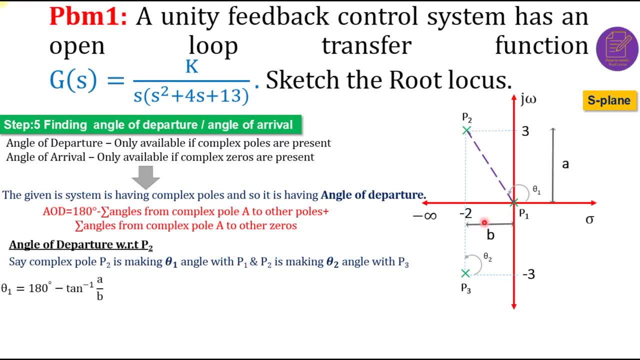 axis. this height of this rectangle and also B is nothing, but this width of also B is nothing, but this width of also B is nothing but this width of this rectangle. okay, this is considered this rectangle. okay, this is considered this rectangle. okay, this is considered. this is a rectangle. okay, so this is this. 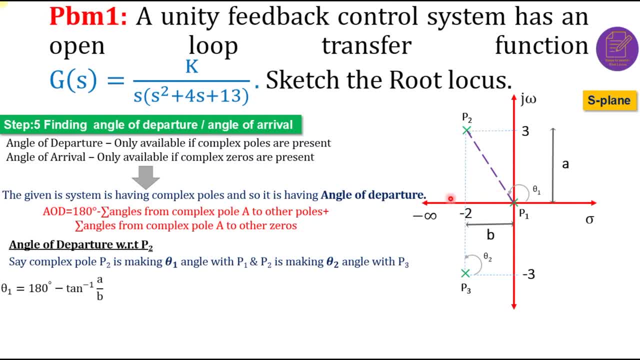 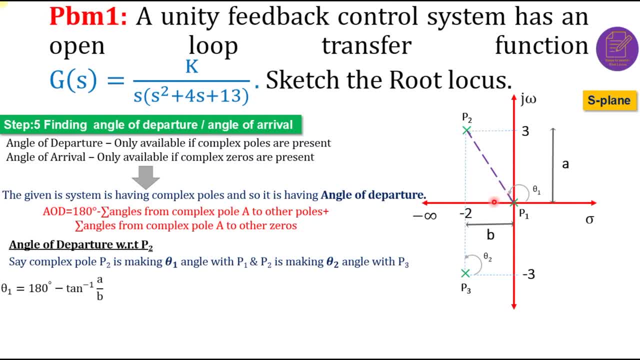 rectangle. okay, so this is this rectangle, if it is, if it is available in this, if it is, if it is, if it is available in this, if it is, if it is, if it is available in this section means this is simple. section means this is simple. section, means this is simple. opposite side, by adjacent side: tan theta. 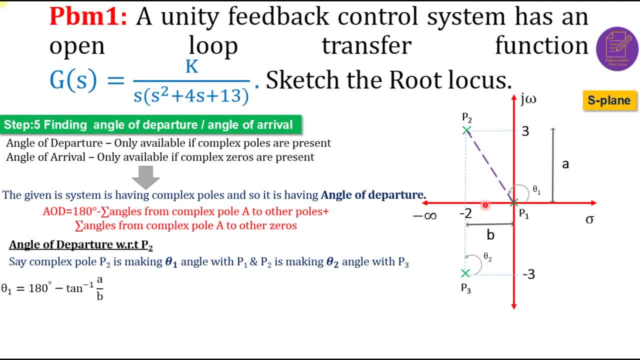 opposite side by adjacent side: tan theta. opposite side by adjacent side: tan theta is equal to opposite side. by adjacent is equal to opposite side. by adjacent is equal to opposite side by adjacent side. my right so theta equal to tan side. my right so theta equal to tan. 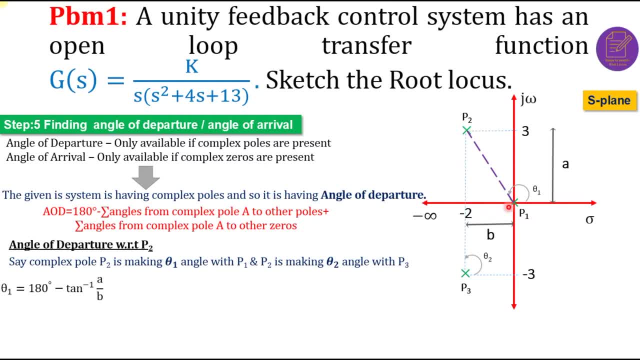 side, my right. so theta equal to tan. inverse of opposite side a adjacent side B. inverse of opposite side a adjacent side B. inverse of opposite side a adjacent side B. if it is, if it is the angle, I mean I. if it is, if it is the angle, I mean I. 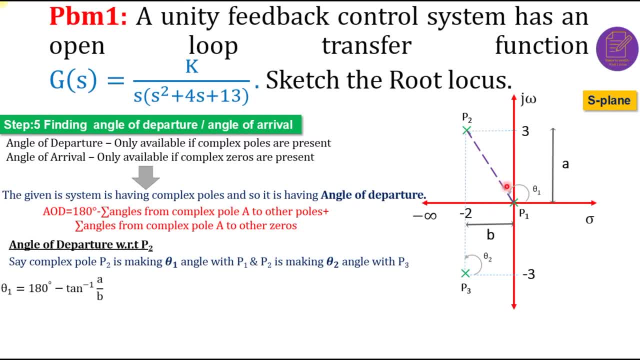 if it is, if it is the angle I mean, I mean the theta 1 is. if the theta 1 is mean the theta 1 is. if the theta 1 is mean the theta 1 is. if the theta 1 is available in this section, we can use the. 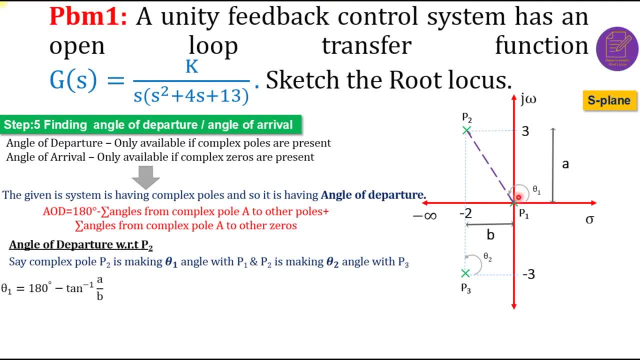 available in this section. we can use the available in this section. we can use the formula tan inverse of a by B, but the formula tan inverse of a by B, but the formula tan inverse of a by B, but the theta 1 is available here, so we need to. 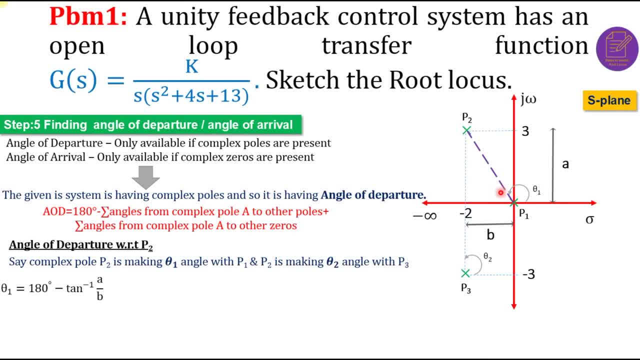 theta 1 is available here, so we need to. theta 1 is available here, so we need to. subtract the angle from 180 degree. subtract the angle from 180 degree. subtract the angle from 180 degree. am I right? this is simple formula, I think. am I right? this is simple formula, I think. 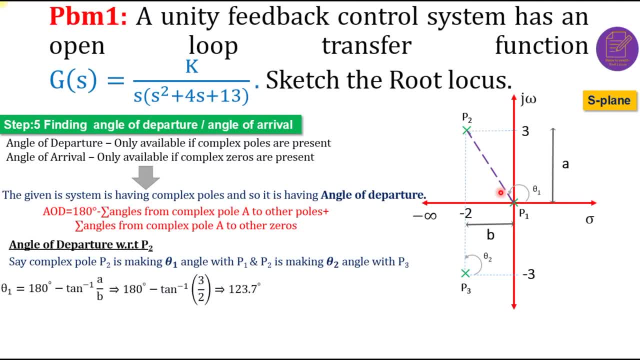 am I right? this is simple formula. I think you can able to get it. okay, just you can able to get it. okay, just you can able to get it. okay, just substitute all the known value. okay, this substitute all the known value. okay, this substitute all the known value. okay, this a value is 3, this is height 3, this is 2. a value is 3. this is height 3, this is 2. a value is 3. this is height 3, this is 2, am I right? so the angle is 123, point 7, am I right? so the angle is 123, point 7? 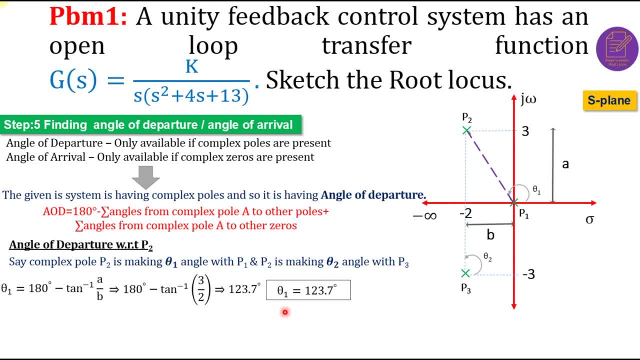 am I right? so the angle is 123 point 7 degree. so subtract this: well sorry degree. so subtract this: well, sorry degree. so subtract this, well sorry. theta 1 is 123 and theta 2 this is 90. theta 1 is 123 and theta 2 this is 90. 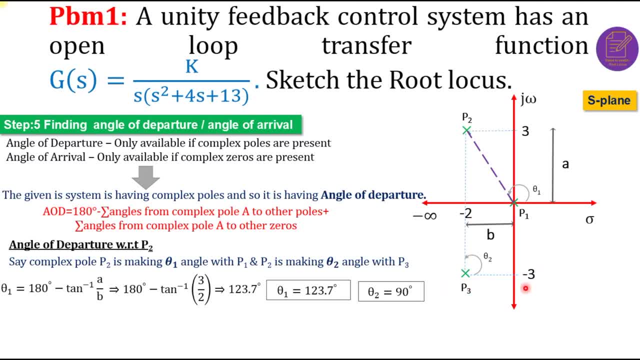 theta 1 is 123 and theta 2: this is 90 degree. am I right? this is exactly 90 degree. am I right? this is exactly 90 degree, am I right? this is exactly 90 degree. so theta 2 is 90 degree. the AOD: 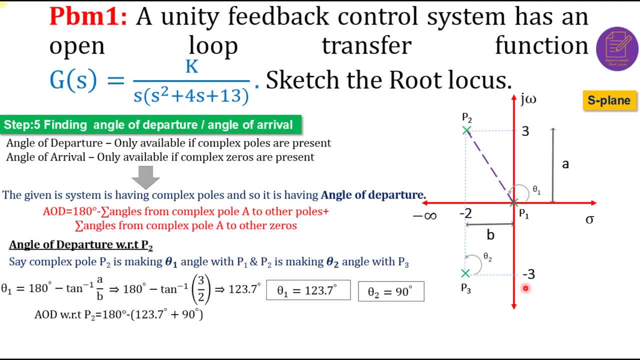 degree, so theta 2 is 90 degree. the AOD degree, so theta 2 is 90 degree. the AOD formula is nothing but 180 degree minus. formula is nothing but 180 degree minus formula is nothing but 180 degree minus sum of angles from complex poles. here: 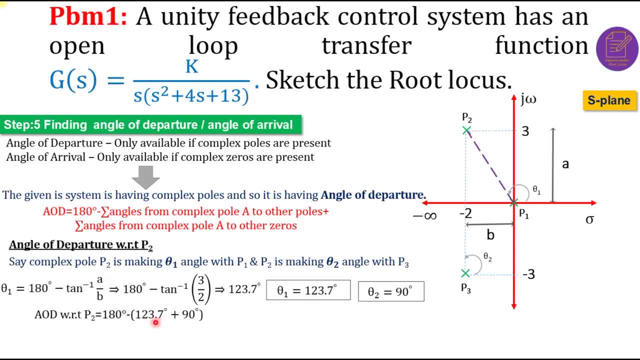 sum of angles from complex poles here, sum of angles from complex poles here to other poles. okay, so 123, 123 point 7 to other poles. okay so, 123, 123 point 7 to other poles. okay so, 123, 123 point 7 degree plus 90 degree. these are all the. 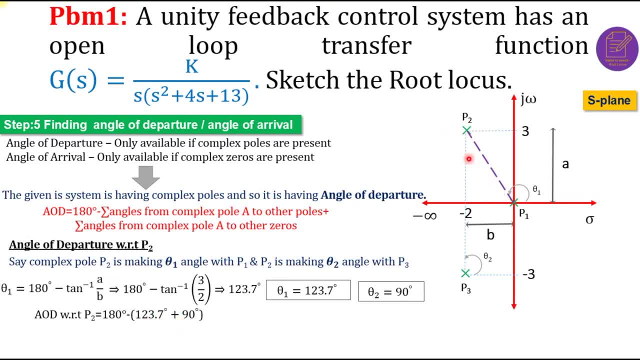 degree plus 90 degree. these are all the degree plus 90 degree. these are all the sum of and sum of angles from complex sum of and sum of angles from complex sum of and sum of angles from complex pole to other poles. am I right the pole to other poles? am I right the? 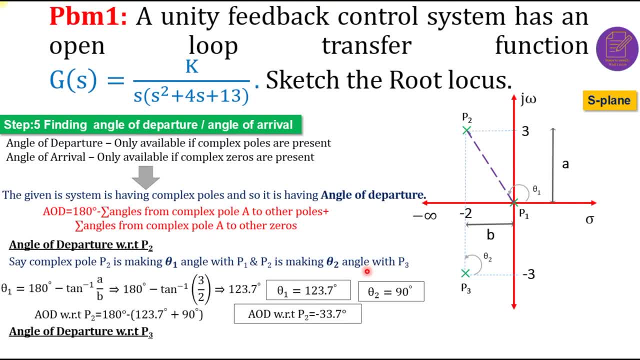 pole to other poles, am I right? the answer is minus 33 point 7 degree, okay. answer is minus 33 point 7 degree, okay. answer is minus 33 point 7 degree, okay. and also angle of departure with respect. and also angle of departure with respect. 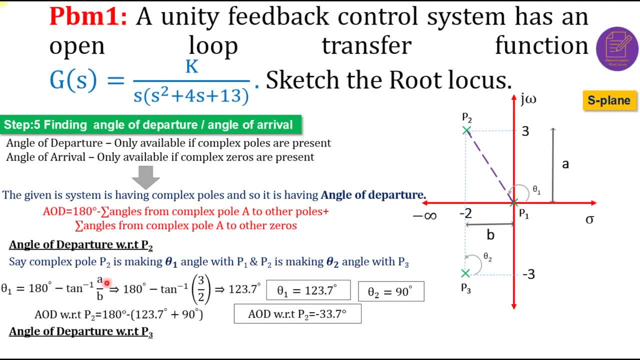 and also angle of departure with respect to pole 3. okay, no need to mess with to pole 3. okay, no need to mess with to pole 3. okay, no need to mess with this formula again. okay, because p3 is this formula again. okay, because p3 is. 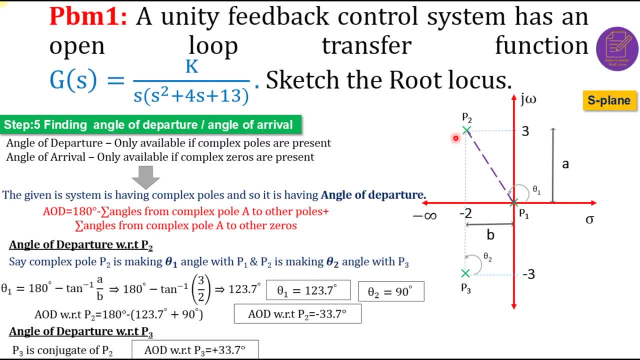 this formula again: okay, because p3 is conjugate of p2. okay, you can take the conjugate of p2. okay, you can take the conjugate of p2. okay, you can take the. you can. you can inverse the sign of the. you can. you can inverse the sign of the. 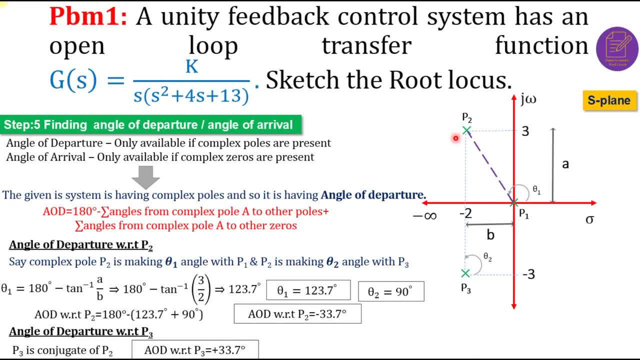 you can. you can inverse the sign of the AOD of point pole 2. okay, if AOD with AOD of point pole 2. okay, if AOD with AOD of point pole 2. okay, if AOD with respect to pole 2 is minus 33, point 7. 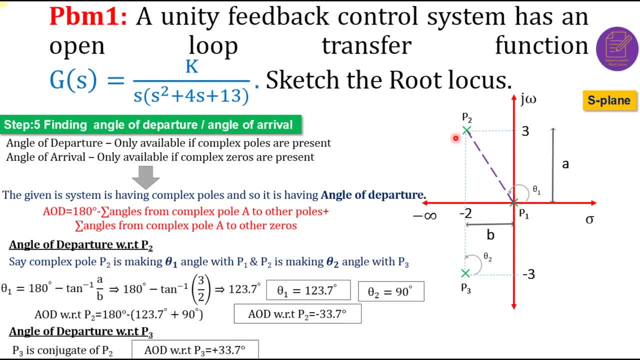 respect to pole 2 is minus 33 point 7. respect to pole 2 is minus 33 point 7 degree AOD. with respect to pole 3 is 33 degree AOD with respect to pole 3 is 33 degree AOD. with respect to pole 3 is 33 point 7 degree. I mean plus 33 point 7. 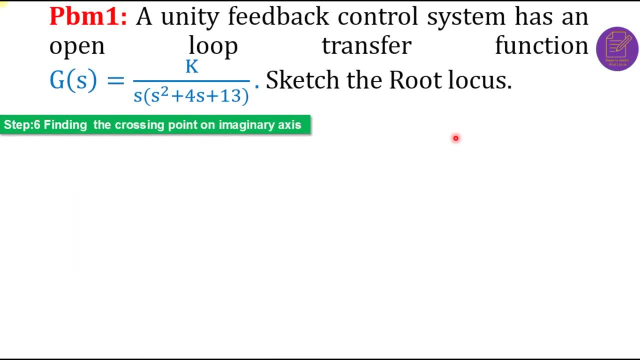 point 7 degree, I mean plus 33 point 7 point 7 degree, I mean plus 33 point 7 degree. okay, this is that step 5 okay degree. okay. this is that step 5, okay degree. okay. this is that step 5, okay, well, solving the root locus while. 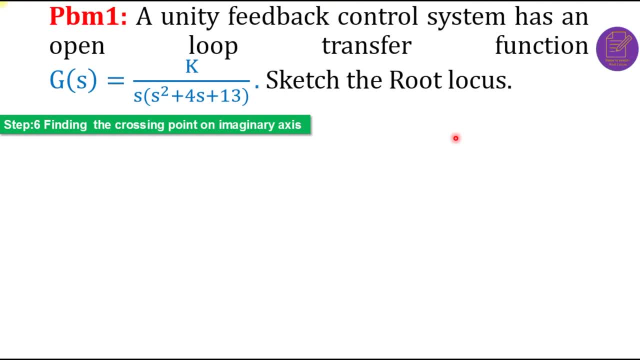 well solving the root locus. while well solving the root locus. while sketching the root locus in last, we will sketching the root locus in last. we will sketching the root locus in last. we will locate. I will explain how to locate this. locate. I will explain how to locate this. 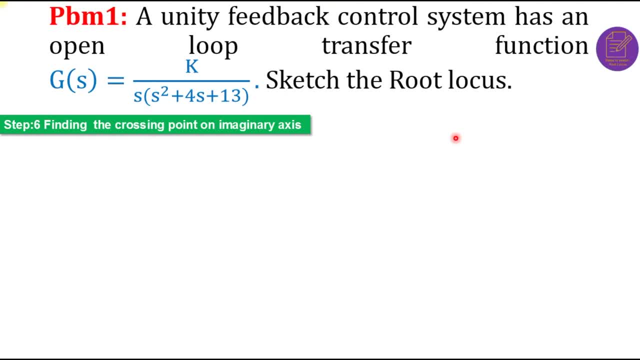 locate. I will explain how to locate this AOD. okay, let me go to the step 6 AOD. okay, let me go to the step 6 AOD. okay, let me go to the step 6: directly finding the closed loop for I. directly finding the closed loop for I. 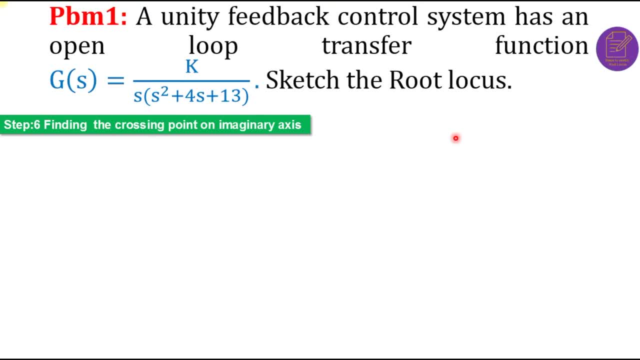 directly finding the closed loop, for I mean finding the cross point on mean, finding the cross point on mean. finding the cross point on imaginary axis. okay, this is six step I. imaginary axis. okay, this is six step I imaginary axis. okay, this is six step I think. okay, so you can go to the rule. 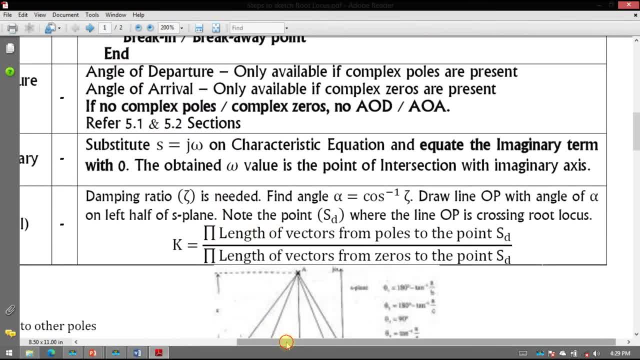 think okay, so you can go to the rule. think okay, so you can go to the rule book now. okay, so this is step number six book now. okay, so this is step number six book now. okay, so this is step number six. finding the point of intersection with: 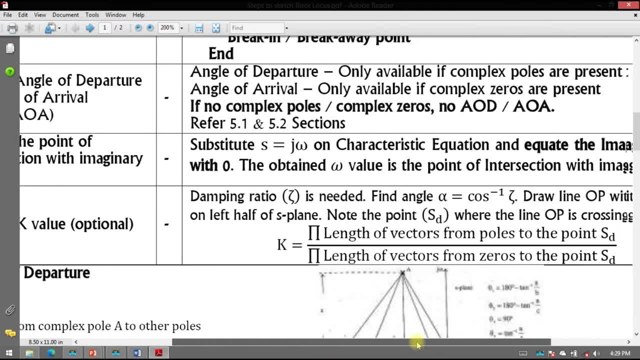 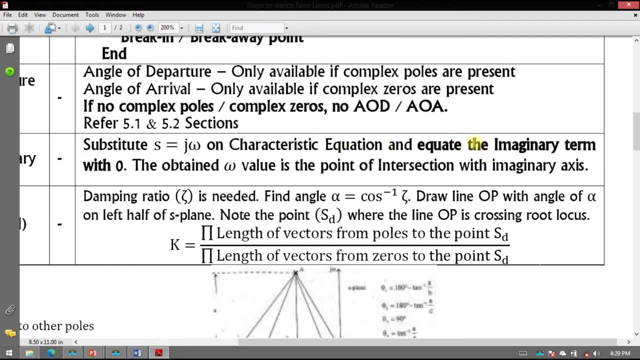 finding the point of intersection with finding the point of intersection with cross point, or the point of intersection, cross point, or the point of intersection, cross point, or the point of intersection. everything is same, right, so substitute. everything is same, right, so substitute. everything is same, right, so substitute the imaginary term with zero: the obtained. 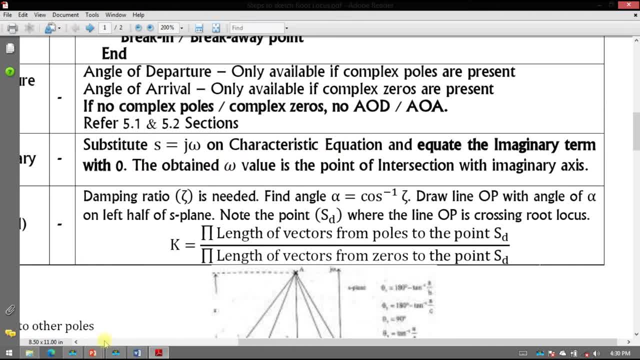 the imaginary term with zero. the obtained the imaginary term with zero. the obtained. the Omega value is the point of the Omega value. is the point of the Omega value. is the point of intersection with the imaginary axis. okay, intersection with the imaginary axis. okay, intersection with the imaginary axis. okay, let's go and solve this. this is: 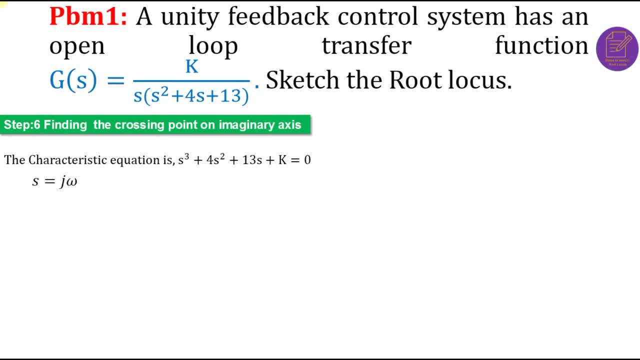 let's go and solve this. this is: let's go and solve this. this is characteristic equation: here you need to. characteristic equation. here you need to. characteristic equation: here you need to. substitute s equal to 0. am I right? yeah, substitute s equal to 0. am I right? yeah? 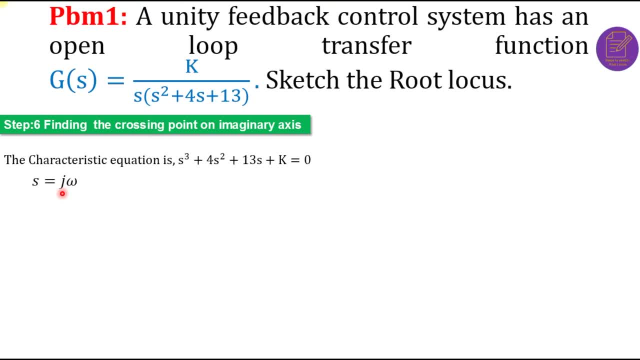 substitute s equal to 0. am I right? yeah s equal to yes, I s equal to J Omega. we s equal to yes, I s equal to J Omega. we s equal to yes, I s equal to J Omega. we need to substitute, okay, so this is the. 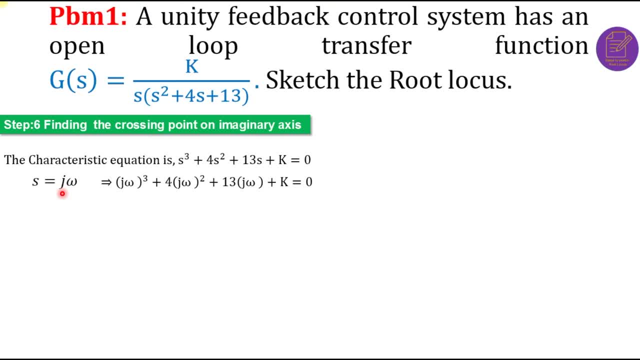 need to substitute. okay, so this is the need to substitute. okay, so this is the response. okay. minus J Omega whole cube response: okay. minus J Omega whole cube response: okay. minus J Omega whole cube plus 4 J Omega whole square plus 13 J. plus 4 J Omega whole square plus 13 J. 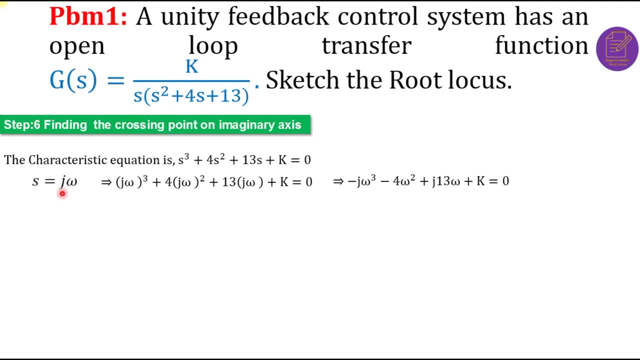 plus 4 J Omega whole square plus 13 J Omega plus K equal to 0. we are getting Omega plus K equal to 0. we are getting Omega plus K equal to 0. we are getting this equation okay minus J Omega Q. this equation okay minus J Omega Q. 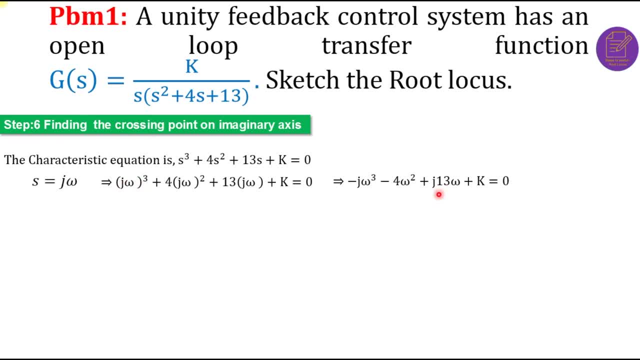 this equation: okay, minus J, Omega Q. because J cube is minus J. okay, so we are. because J cube is minus J. okay, so we are. because J cube is minus J. okay, so we are. getting this equation equal, equate the. getting this equation equal, equate the. 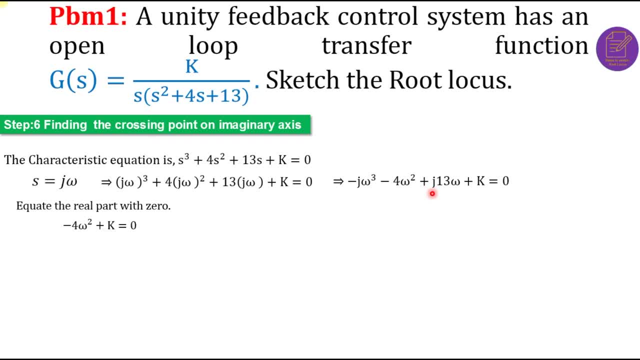 getting this equation equal. equate: the real part with respect to Z with to 0. real part with respect to Z with to 0. real part with respect to Z with to 0. okay, so I'm taking this real parts 4 J. okay, so I'm taking this real parts 4 J. 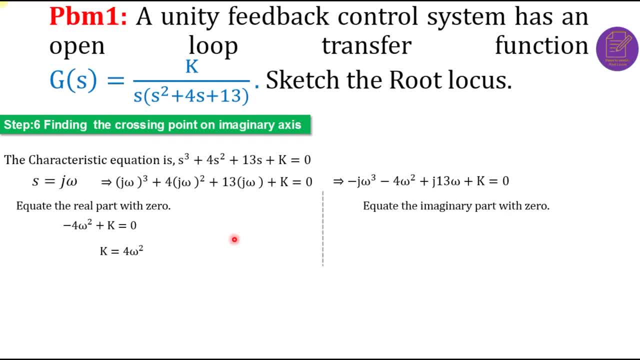 okay, so I'm taking this real, parts 4, J, Omega square, and then I am going to Omega square and then I am going to Omega square and then I am going to equate the imaginary part with the 0. I am. equate the imaginary part with the 0, I am. 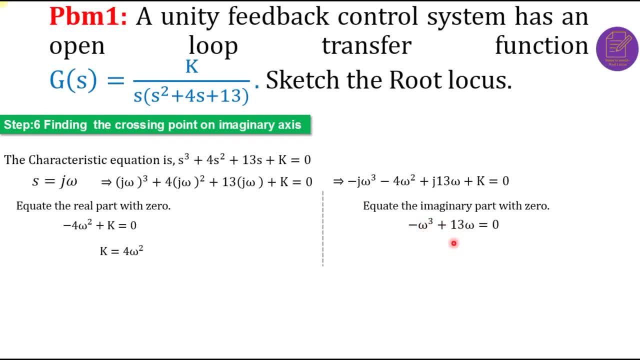 equate the imaginary part with the 0, I am getting okay, minus Omega cube plus 13. getting okay, minus Omega cube plus 13. getting okay, minus Omega cube plus 13 Omega: okay, this is equivalent to minus Omega. okay, this is equivalent to minus Omega. okay, this is equivalent to minus Omega square plus 13, so Omega square. 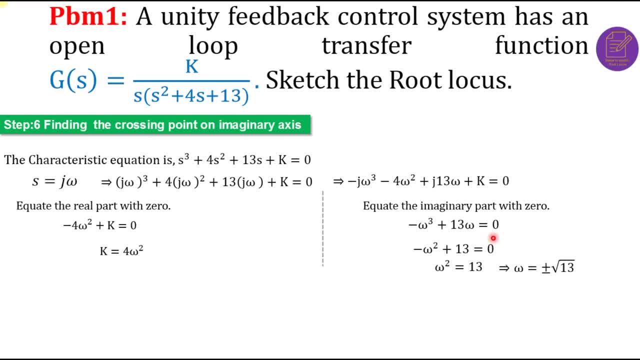 Omega square plus 13, so Omega square. Omega square plus 13, so Omega square equal to 13. Omega equal to plus or equal to 13. Omega equal to plus or equal to 13. Omega equal to plus or minus root 13 and Omega equal to plus or. 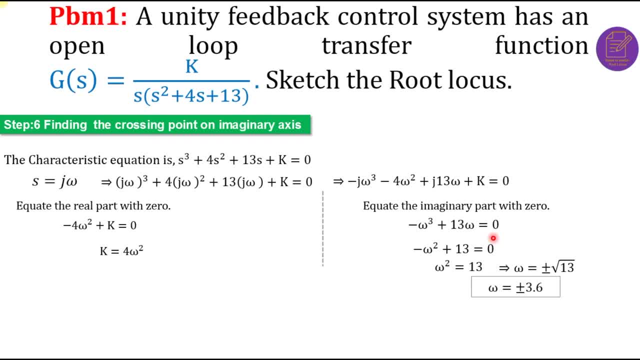 minus root 13 and Omega equal to plus or minus root 13 and Omega equal to plus or minus 3.6. so we can also calculate the K minus 3.6. so we can also calculate the K minus 3.6, so we can also calculate the K value here. okay, so for if you want to. 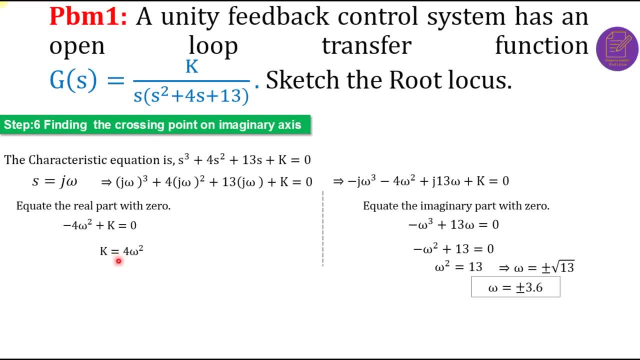 value here: okay. so for if you want to value here, okay, so for if you want to find out the open loop- I mean closed, find out the open loop, I mean closed, find out the open loop, I mean closed. loop gain: okay, substitute Omega square. loop gain: okay, substitute Omega square. 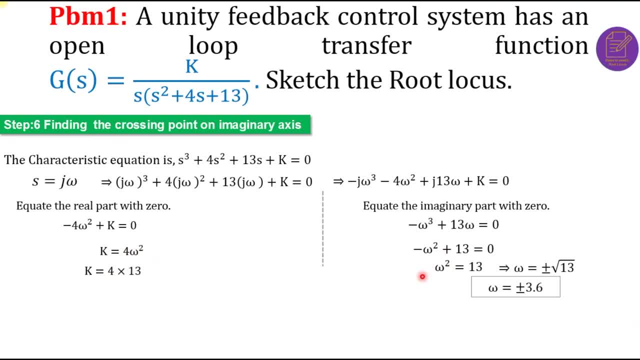 loop gain: okay, substitute: Omega square equal to 13. am I right? so Omega square equal to 13, am I right? so Omega square equal to 13, am I right? so Omega square equal to 13 and K equal to 52? okay, so equal to 13 and K equal to 52, okay so. 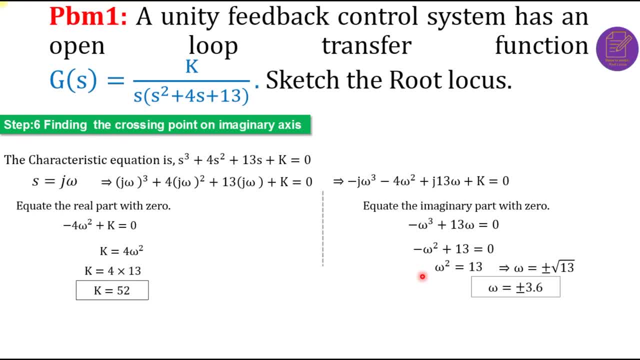 equal to 13 and K equal to 52. okay, so far to sketch the root locus. we need far to sketch the root locus. we need far to sketch the root locus. we need only the intersecting intersection point, only the intersecting intersection point, only the intersecting intersection point with the imaginary axis right so? 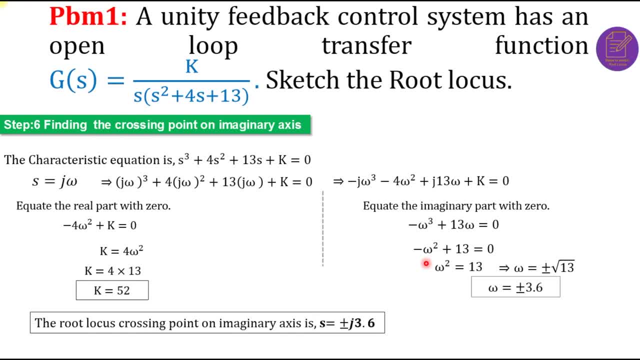 with the imaginary axis right. so with the imaginary axis, right. so intersection point, I mean the crossing intersection point, I mean the crossing intersection point. I mean the crossing point on imaginary axis is equal to plus. point on imaginary axis is equal to plus. point on imaginary axis is equal to plus R minus J, 3.6. okay, so these are all the. 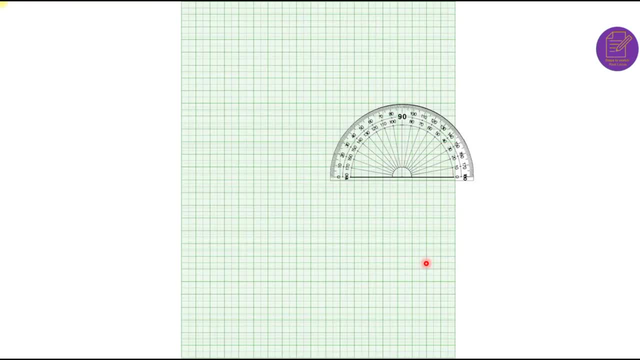 R minus J 3.6. okay, so these are all the R minus J 3.6. okay, so these are all the stick six steps, okay, and then we will stick six steps, okay, and then we will stick six steps. okay, and then we will take the sorry, we will take the what. 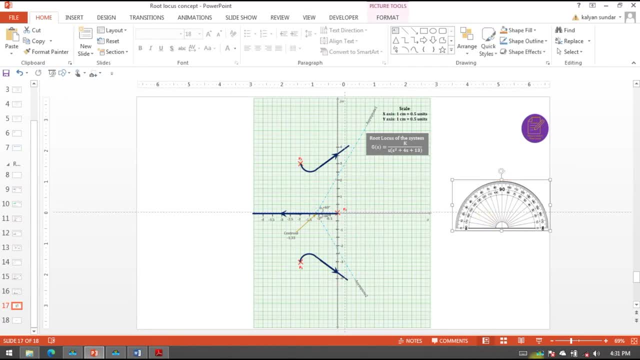 take the sorry. we will take the what. take the sorry. we will take the what graph sheet like this: okay, so we will graph sheet like this: okay, so we will graph sheet like this: okay, so we will take the graph sheet like this and take the graph sheet like this and. 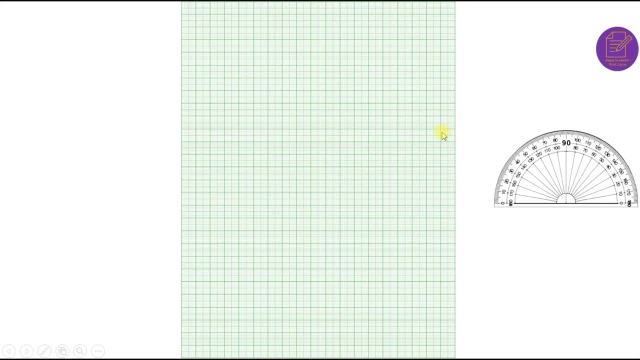 take the graph sheet like this and we'll sketch the root locus here. okay, we'll sketch the root locus here. okay, we'll sketch the root locus here. okay, initially I am taking real axis in X initially. I am taking real axis in X initially. I am taking real axis in X axis and I am taking the imaginary axis. 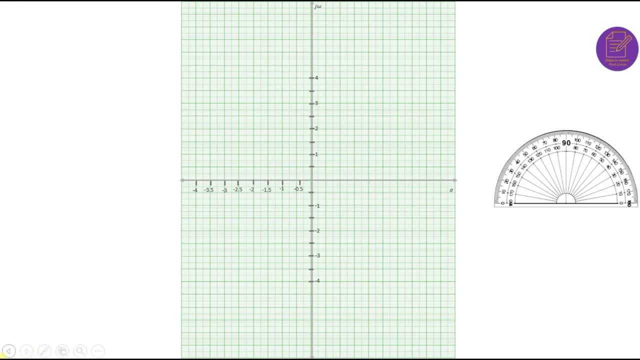 axis and I am taking the imaginary axis axis and I am taking the imaginary axis in y-axis. okay, step number one is okay in y- axis. okay, step number one is okay in y- axis. okay, step number one is okay, please wait. yeah, this is step number one. 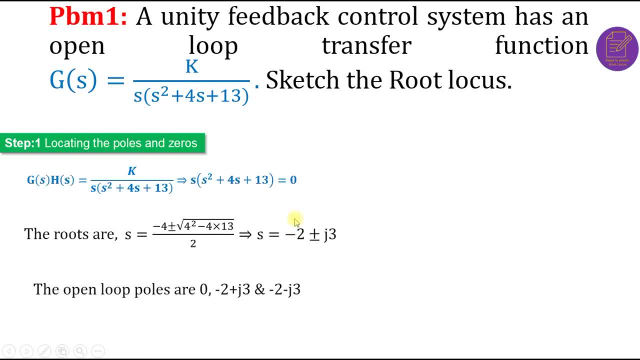 please wait. yeah, this is step number one. please wait, yeah, this is step number one. am I right? locating the poles, okay. so am I right, locating the poles, okay. so am I right? locating the poles, okay. so locating the poles means we are having. locating the poles means we are having. 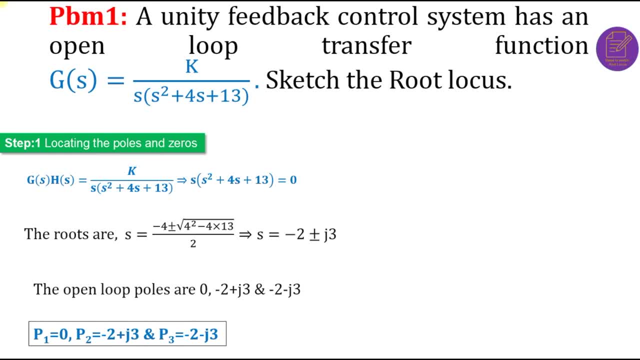 locating the poles means we are having three poles 0 minus 2 minus 2 plus J 3. three poles 0 minus 2 minus 2 plus J 3. three poles 0 minus 2 minus 2 plus J 3 minus 2 minus J 3, my right. so this is: 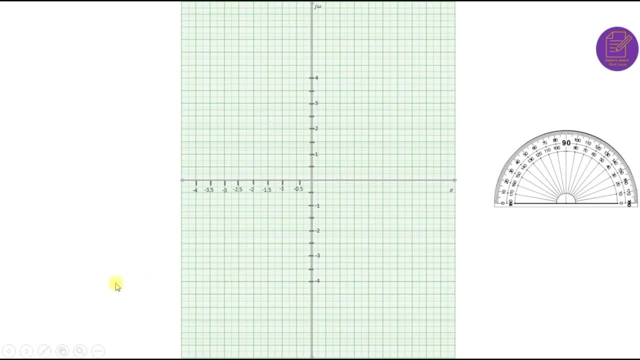 minus 2 minus J 3, my right. so this is minus 2 minus J 3, my right. so this is our step 1. I mean locating the open loop. our step 1. I mean locating the open loop. our step 1. I mean locating the open loop poles. okay, P 1, P 2 and P 3. step 2 is: 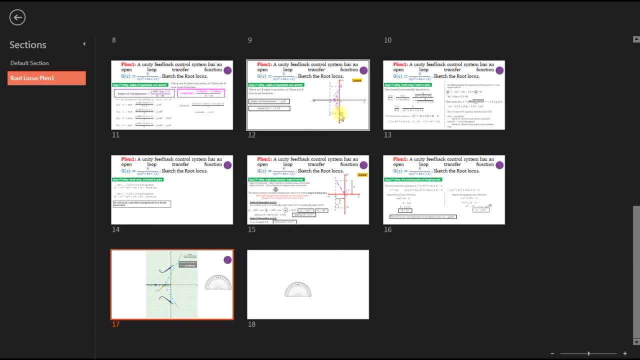 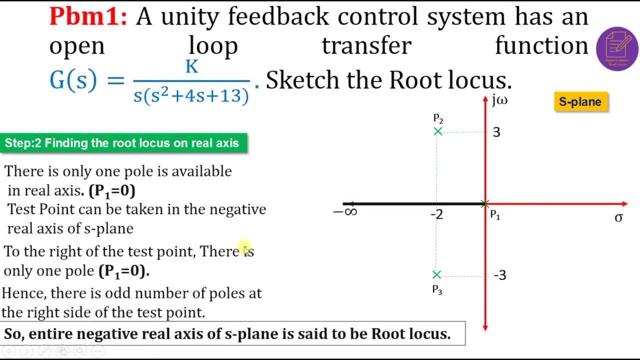 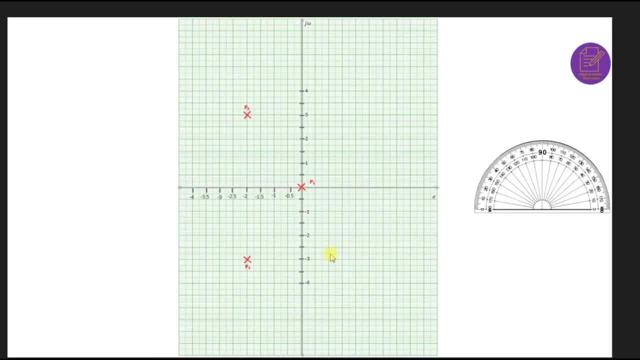 this is we what we found in our second. this is we what we found in our second step. okay, so let's solve the second step step. okay, so let's solve the second step step. okay, so let's solve the second step is: this is the root locus present at the: 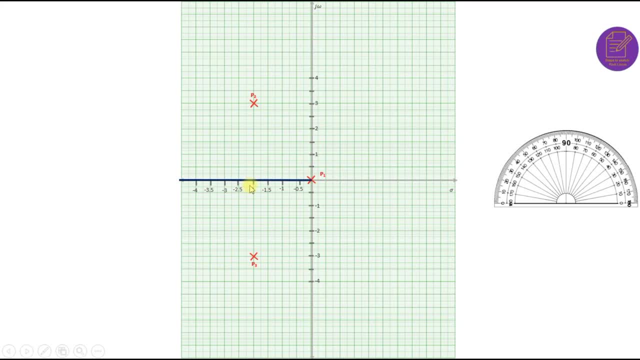 is. this is the root locus present at the. is. this is the root locus present at the negative real axis: the entire negative, negative real axis, the entire negative, negative real axis, the entire negative real axis. we need to highlight, okay, we real axis. we need to highlight, okay, we. 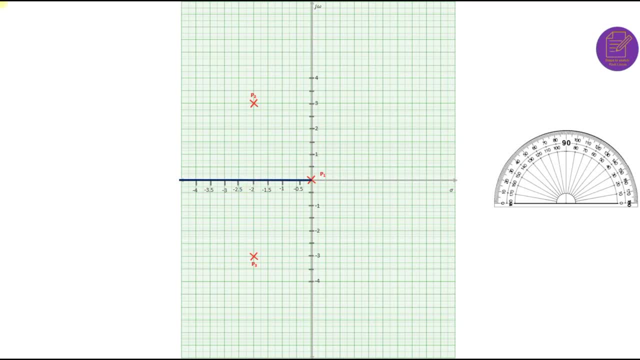 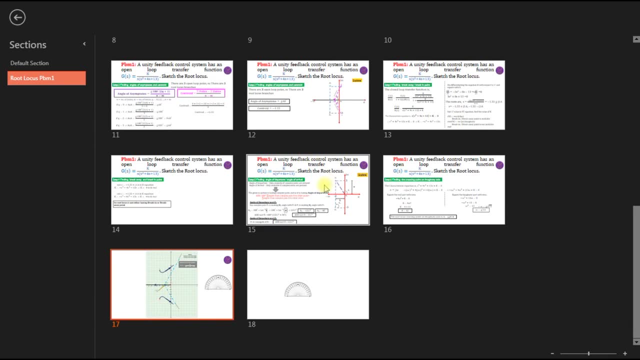 real axis we need to highlight. okay, we need to draw with the thick line. okay, so need to draw with the thick line. okay, so need to draw with the thick line, okay, so the third step is okay. the third step, the third step, the third step. what is third step? yeah, this is the third. 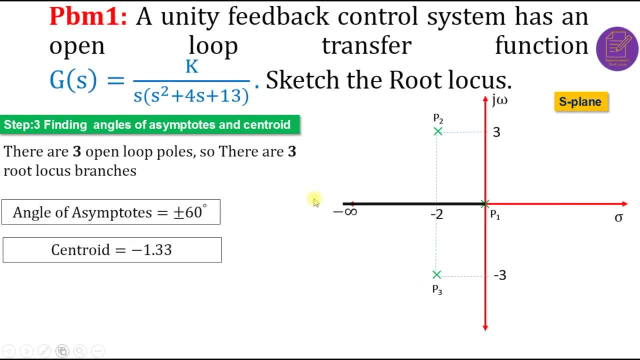 what is third step? yeah, this is the third. what is third step? yeah, this is the third step. yeah, this is centroid angle of step. yeah, this is centroid angle of step. yeah, this is centroid angle of asymptotes and centroid. okay, so we mark asymptotes and centroid. okay, so we mark. 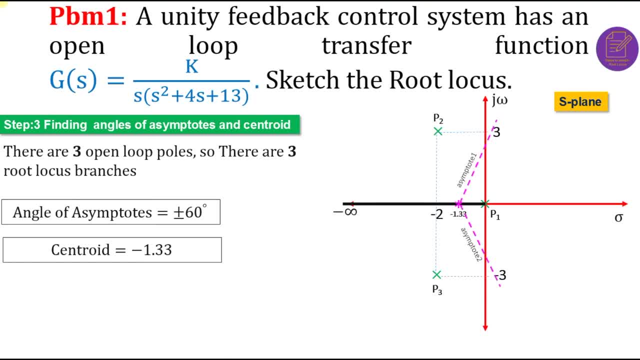 asymptotes and centroid. okay, so we mark with the centroid point and on that, with the centroid point and on that with the centroid point and on that point itself. we need to draw the point itself. we need to draw the point itself. we need to draw the asymptotes 1 and 2, am I right? so here, 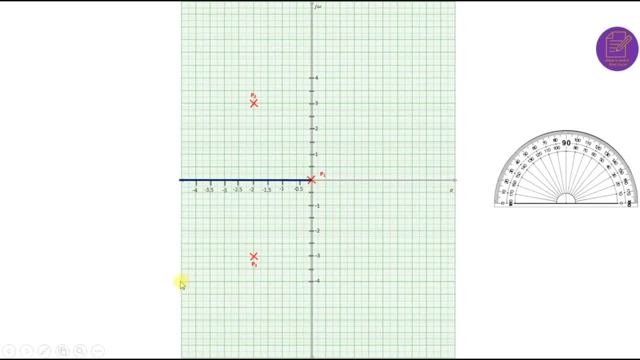 asymptotes 1 and 2, am I right? so here, asymptotes 1 and 2, am I right? so here also, in our graph sheets itself, we need also in our graph sheets itself. we need also in our graph sheets itself. we need to place the protector on this point. are 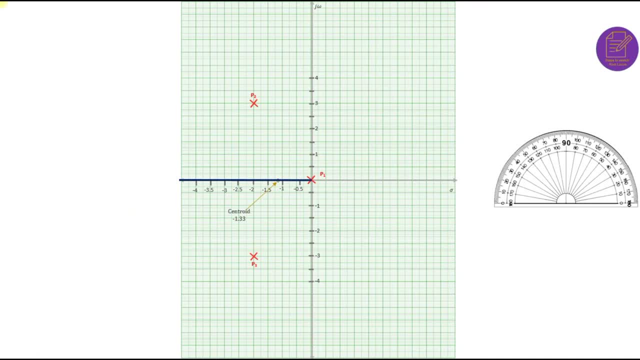 to place the protector on this point are to place the protector on this point. are you able to understand one point minus you able to understand one point minus? you able to understand one point minus 1.33? this is the exact centroid point: 1.33. this is the exact centroid point. 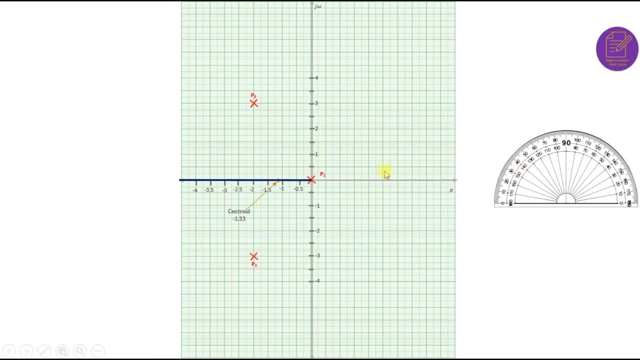 1.33. this is the exact centroid point. just place the protector here. take the just place the protector here. take the just place the protector here. take the anti-clockwise 60 degree. this is anti-clockwise 60 degree. this is anti-clockwise 60 degree. this is asymptote 1, and just place the protector. 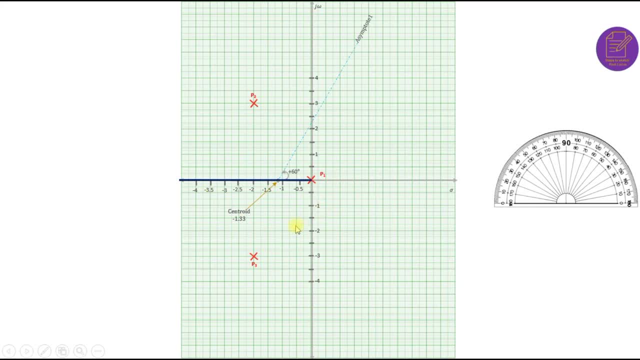 asymptote 1- and just place the protector- asymptote 1- and just place the protector in reverse direction. here, the point in reverse direction here, the point in reverse direction, here the point should be in centroid. okay, then the should be in centroid. okay, then the should be in centroid. okay, then the origin, I mean this origin- should be: 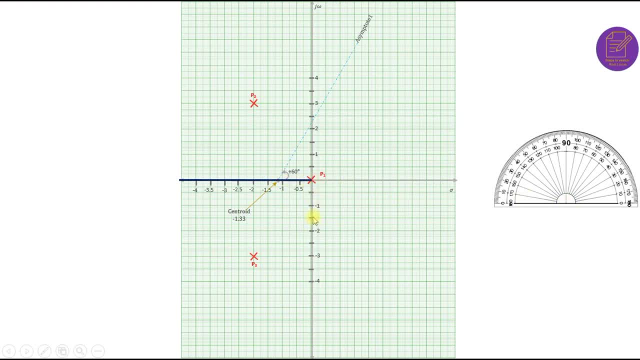 origin. I mean this origin should be origin. I mean this origin should be coincide with this centroid and take the coincide with this centroid and take the coincide with this centroid and take the clockwise 60 degree. this is asymptote 2. clockwise 60 degree: this is asymptote 2. 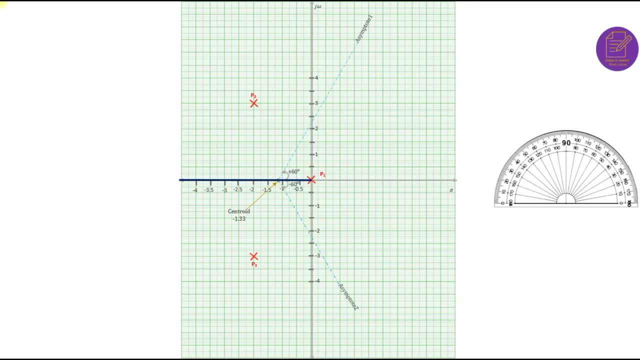 clockwise 60 degree. this is asymptote 2. okay, I am telling that. okay, my root. okay, I am telling that. okay, my root, okay, I am telling that. okay, my root locus on second or third quadrant, locus on second or third quadrant, locus on second or third quadrant should follow the same direction. so, okay, 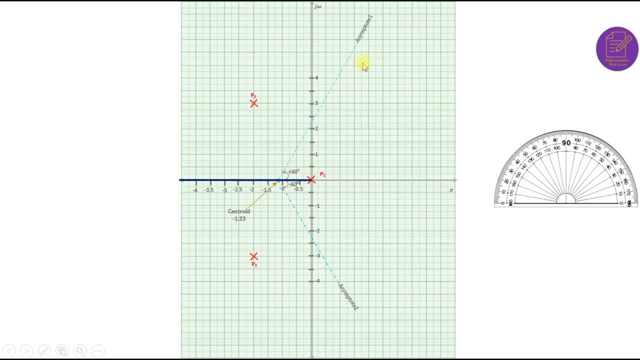 should follow the same direction. so, okay, should follow the same direction. so, okay, this is the asymptote line. okay, as in. this is the asymptote line. okay, as in. this is the asymptote line. okay, as in: toward me, this is a guidelines. okay, toward me, this is a guidelines okay. 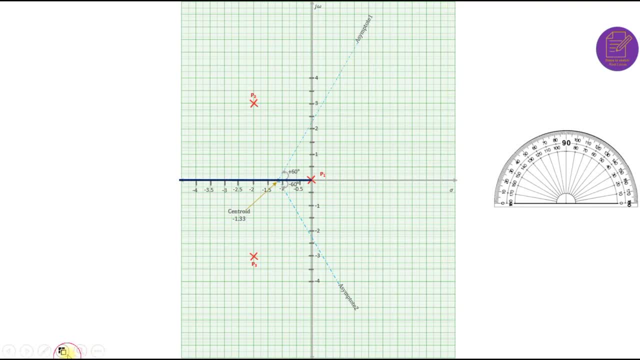 toward me. this is a guidelines. okay, step number four. what is step number four? step number four. what is step number four? step number four. what is step number four? yeah, step number four. we told that, yeah, step number four. we told that, yeah, step number four. we told that we have checked some conditions. okay, based. 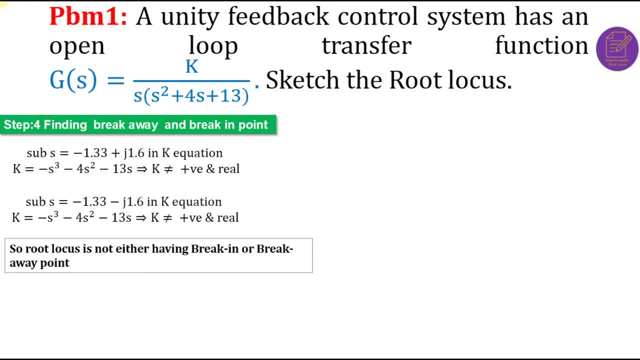 we have checked some conditions okay based. we have checked some conditions okay. based on that, we are tell, we already told on that. we are tell, we already told on that. we are tell, we already told: right, the root locus is not having any right, the root locus is not having any. 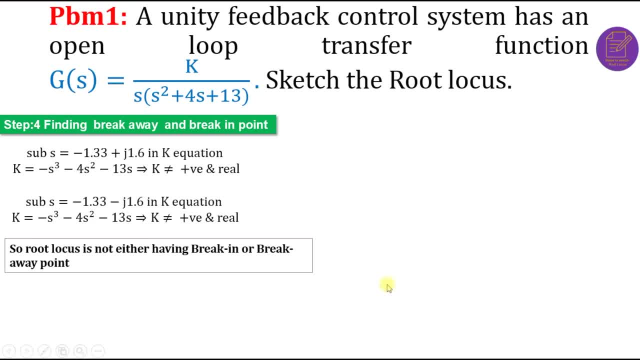 right, the root locus is not having any. either break in or break away point okay. either break in or break away point okay. either break in or break away point. okay. so no issues. there is no fourth, I mean, so no issues. there is no fourth, I mean, so no issues. there is no fourth, I mean there is no break in or break away point. 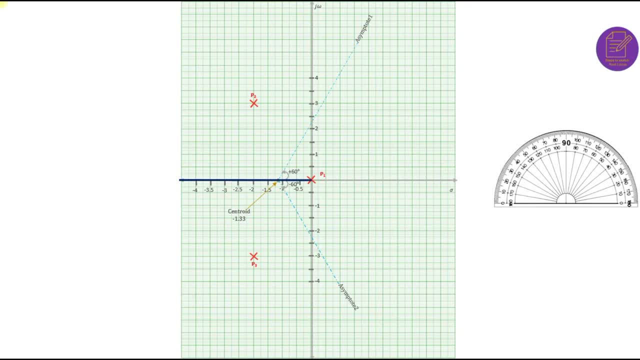 there is no break in or break away point. there is no break in or break away point for our root locus diagram. so we can move for our root locus diagram. so we can move for our root locus diagram. so we can move on to the step number five. okay, what? 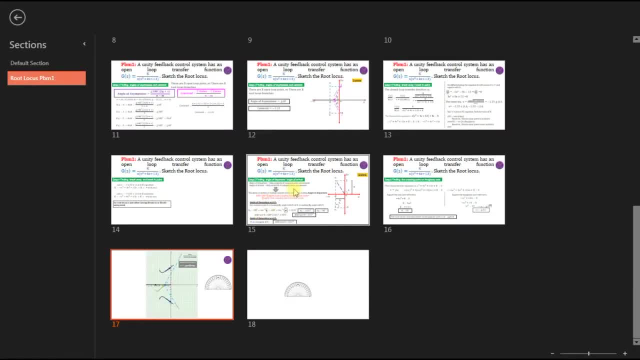 on to the step number five. okay. what on to the step number five? okay, what is step number five? step number five is is step number five. step number five is is step number five. step number five is nothing but angle of departure and angle, nothing but angle of departure and angle. 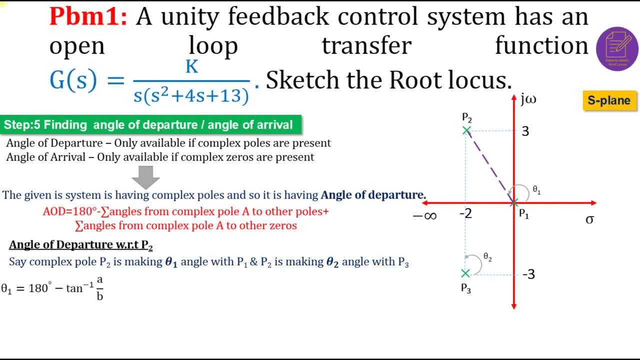 nothing but angle of departure and angle of arrival. okay in our problem we are of arrival. okay in our problem we are of arrival. okay in our problem we are having only angle of what angle, of having only angle of what angle, of having only angle of what angle of departure? the angle of departure is: 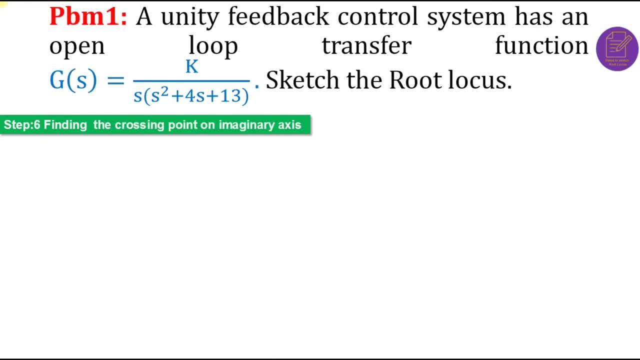 departure, the angle of departure is departure, the angle of departure is nothing but, and this is the sorry, this, nothing but. and this is the sorry, this, nothing but, and this is the sorry. this is the value of angle of departure for is the value of angle of departure for? 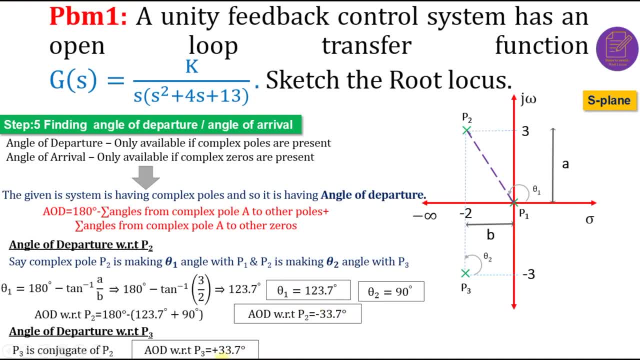 is the value of angle of departure for pole 2- this is minus 33.7 degree, and pole 2- this is minus 33.7 degree. and pole 2: this is minus 33.7 degree and pole 3: this is plus 33.7 degree. okay, so. 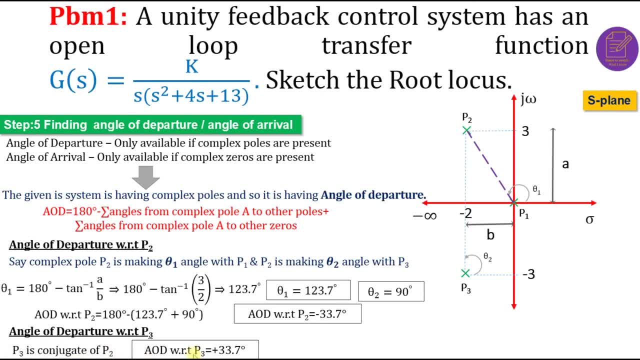 pole 3: this is plus 33.7 degree. okay. so, pole 3: this is plus 33.7 degree, okay. so that what we have to do is: let me let that. what we have to do is, let me let that. what we have to do is, let me let me solve- please wait, yeah. angle of. 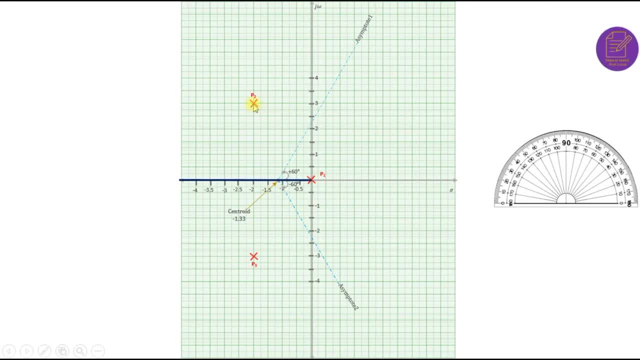 me solve, please wait. yeah, angle of me solve, please wait. yeah, angle of departure means you need to take 33 departure. means you need to take 33 departure. means you need to take 33 degree: 33.7 degree minus 33.7 degree. degree: 33.7 degree minus 33.7 degree. 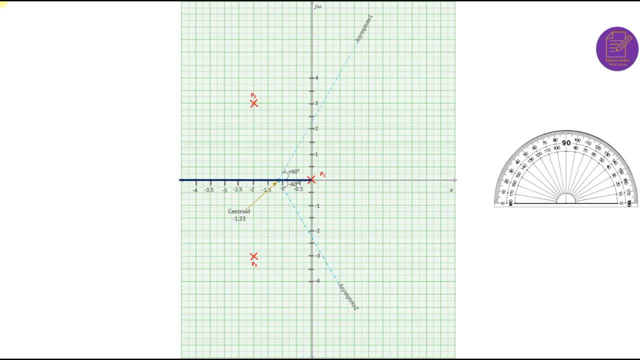 degree. 33.7 degree minus 33.7 degree means you need to take the take. the means you need to take the take, the means you need to take the take the angles in clockwise direction plus 33.7 angles in clockwise direction plus 33.7. 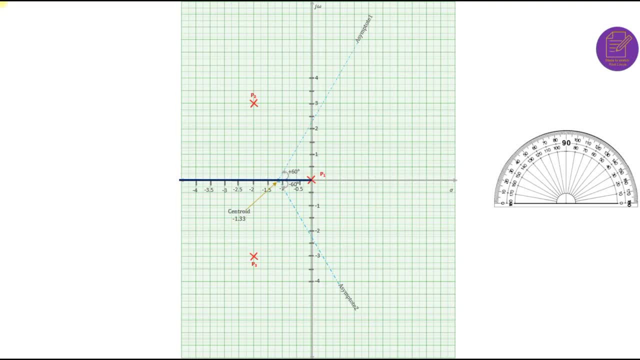 angles in clockwise direction. plus 33.7 degree means you need to take in reverse degree. means you need to take in reverse degree. means you need to take in reverse direction, anticlockwise direction. am I direction anticlockwise direction? am I direction anticlockwise direction? am I right? so plus 33 degree you need to take. 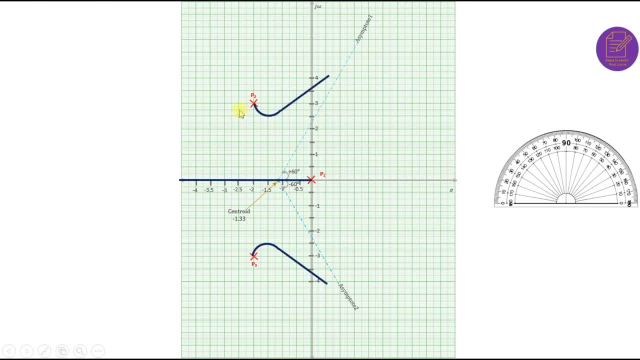 right. so plus 33 degree you need to take, right. so plus 33 degree you need to take means this is the angle okay. so this is means this is the angle okay, so this is means this is the angle okay, so this is the angle, I mean, and we are telling 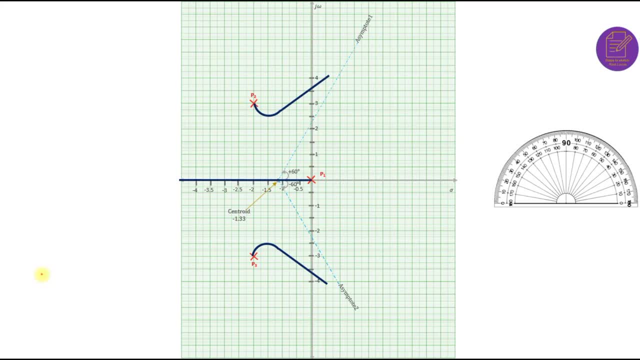 the angle. I mean, and we are telling the angle. I mean, and we are telling about this, I will. I will draw with the about this, I will. I will draw with the about this, I will. I will draw with the help of this pen. please consider the. yeah. 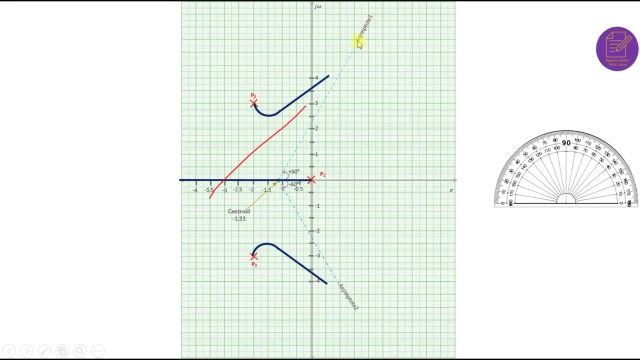 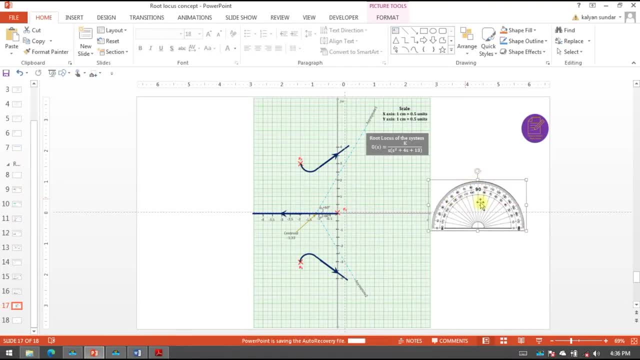 yeah, we are telling about with the angle, I mean. and we are telling about: yeah, we are telling about with the angle, I mean, and we are telling about: see minus 33 degree means we need to go. see minus 33 degree means we need to go. see minus 33 degree means we need to go. yeah, you need to go in clockwise. 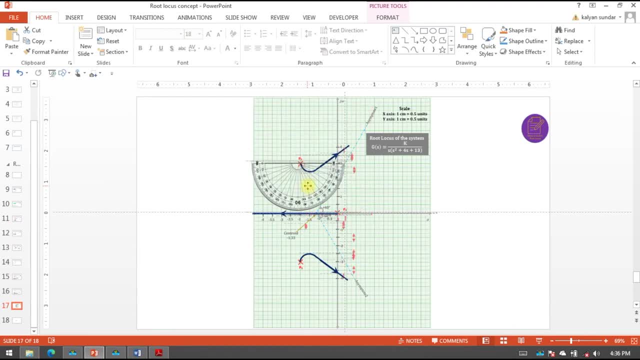 yeah, you need to go in clockwise. yeah, you need to go in clockwise direction, right. so I am going to fix the direction right. so I am going to fix the direction right. so I am going to fix the protector here. okay, I have approximately protector here. okay, I have approximately. 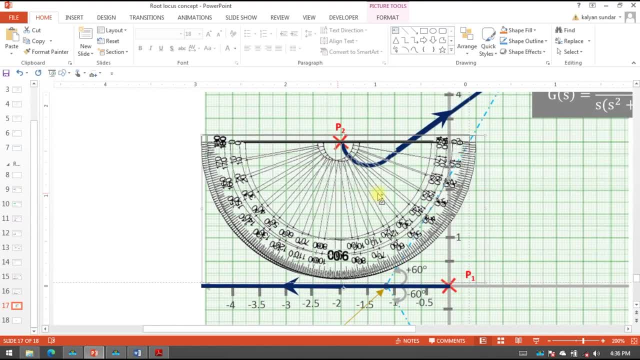 protector here. okay, I have approximately drawn the diagram, but exact point. okay, drawn the diagram, but exact point. okay, drawn the diagram, but exact point. okay, we were to understand, okay, and my, we were to understand okay, and my, we were to understand okay, and my protector is pointed over here. 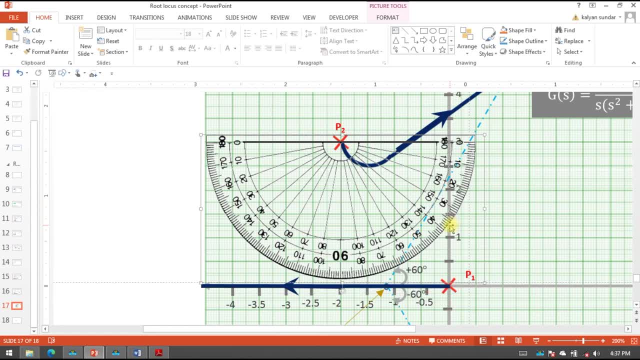 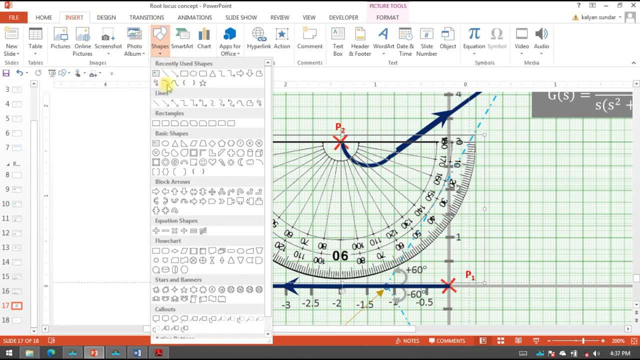 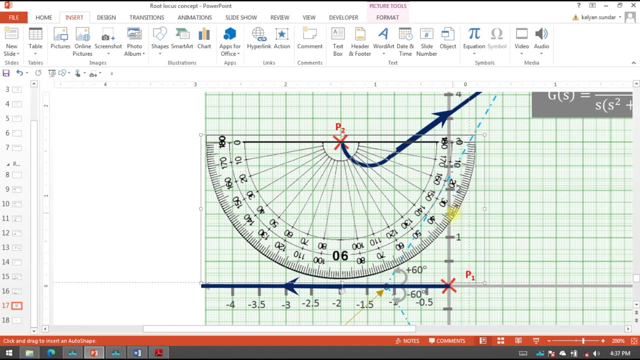 protector is pointed over here. protector is pointed over here. okay, 33.7 degree is actually here, okay, okay, 33.7 degree is actually here, okay, okay, 33.7 degree is actually here, okay, so we need to locate. yeah, see 33.7. 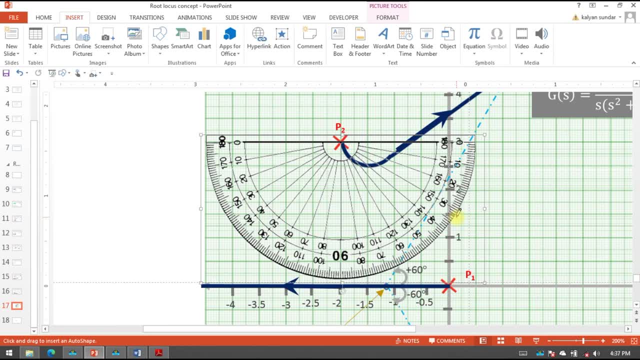 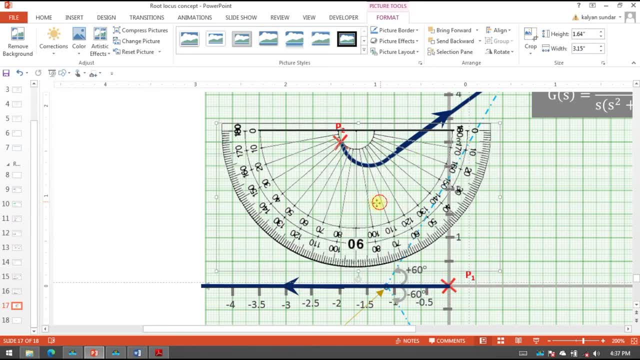 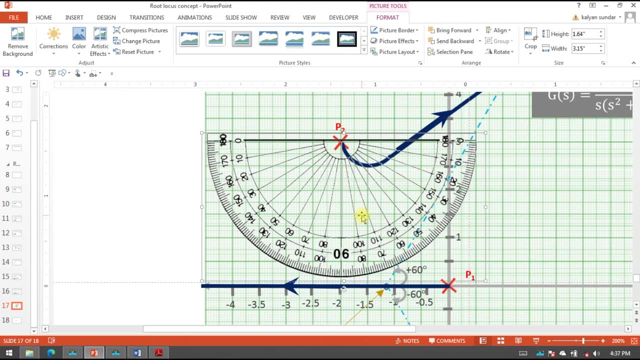 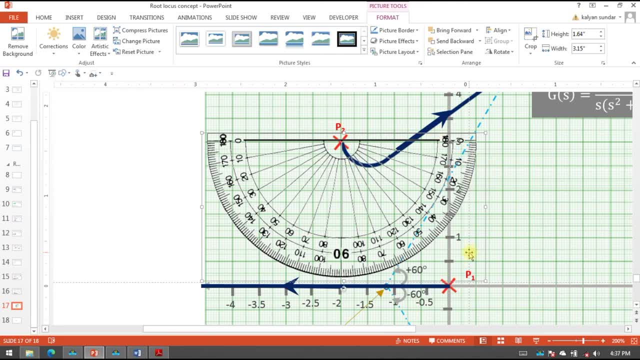 degree okay minus 33.7 degree means degree okay minus 33.7 degree means we need to go in this direction. I mean we need to go in this direction. I mean we need to go in this direction, I mean clockwise direction. so that is why the 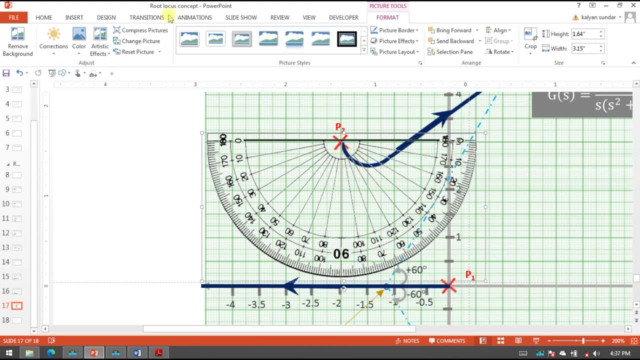 clockwise direction. so that is why the clockwise direction, so that is why the product is being fixed with this data product is being fixed with this data product is being fixed with this data direction. okay, so here I am going to direction. okay, so here I am going to. 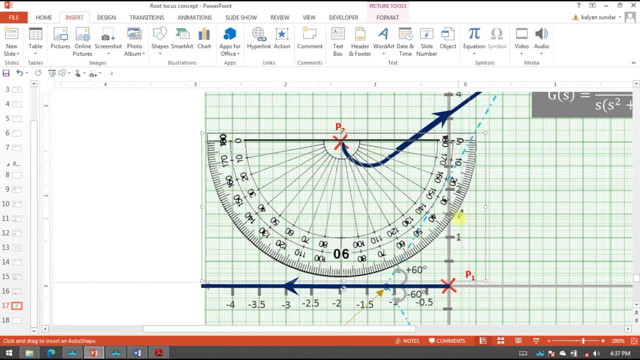 direction. okay, so here I am going to take 30, take 30, take 30. yeah, this is picture actually, so only I. yeah, this is picture actually, so only I. yeah, this is picture actually, so only I am not able to fix it. yeah, nearly here, am not able to fix it. yeah, nearly here. 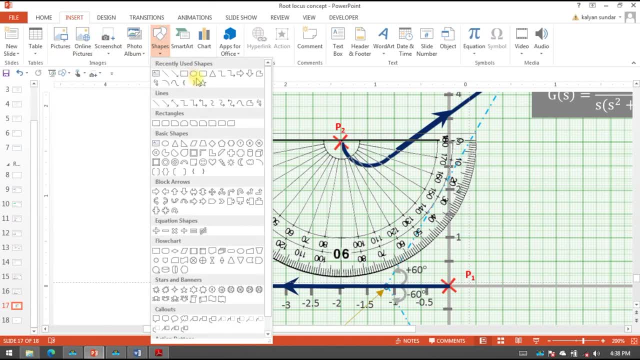 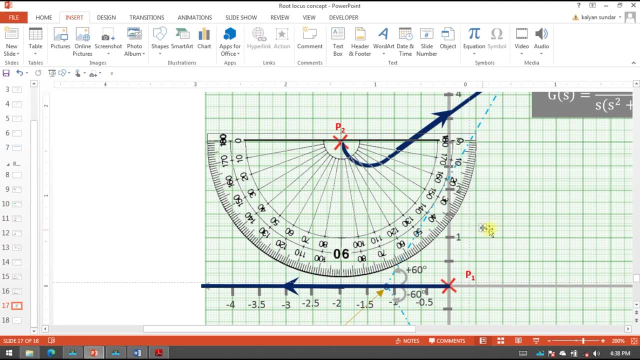 am not able to fix it. yeah, nearly here, okay, so sorry for this trouble. it is okay, so sorry for this trouble. it is okay, so sorry for this trouble. it is exactly, yeah, okay, are able to get it. so exactly, yeah, okay, are able to get it so. 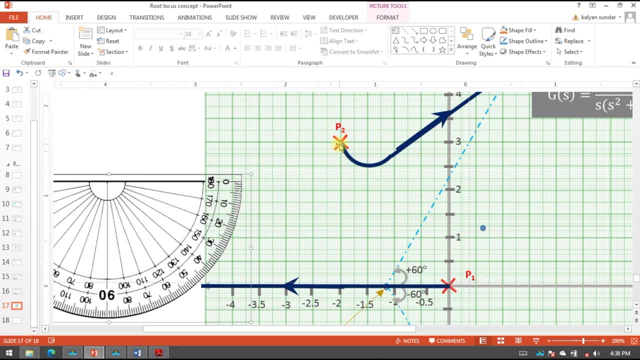 exactly. yeah, okay, are able to get it. so this is actually 33.7 okay. so we need. this is actually 33.7 okay. so we need. this is actually 33.7 okay. so we need to draw a daughter like like this: okay, to draw a daughter like like this: okay. 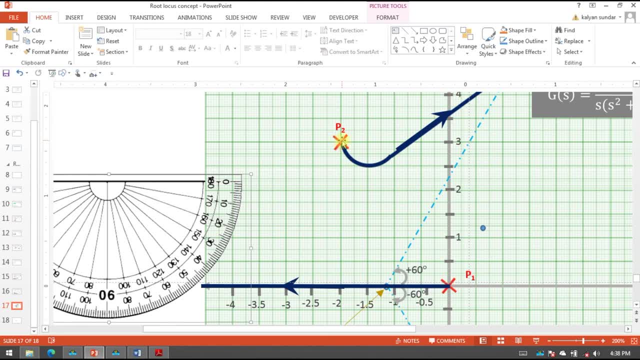 to draw a daughter, like like this: okay, from this pole p2 itself. there should be. from this pole p2 itself. there should be. from this pole p2 itself. there should be a angle of departure of 33.7 degree. okay, a angle of departure of 33.7 degree, okay. 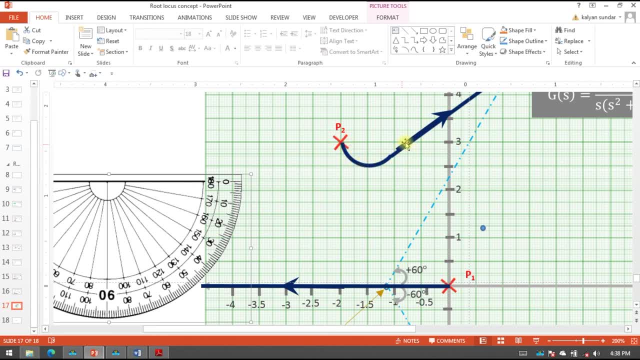 a angle of departure of 33.7 degree. okay, the root locus is start going and it, the root locus is start going and it, the root locus is start going and it is cutting at 3.6. okay, are able to. is cutting at 3.6? okay, are able to. 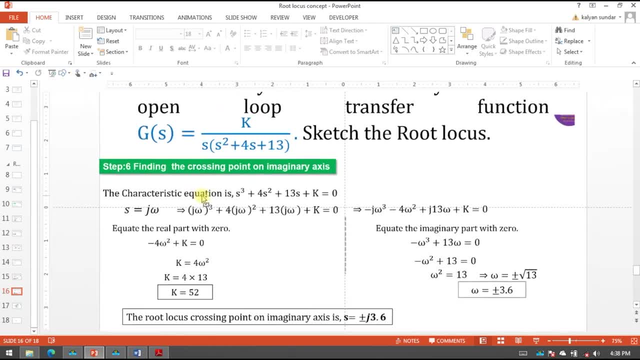 is cutting at 3.6. okay, are able to understand the imaginary axis crossing. understand the imaginary axis crossing. understand the imaginary axis crossing. point is 3.6. okay, so here you can able to. point is 3.6. okay, so here you can able to. 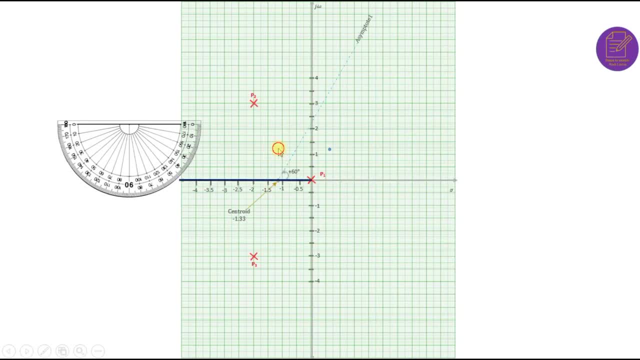 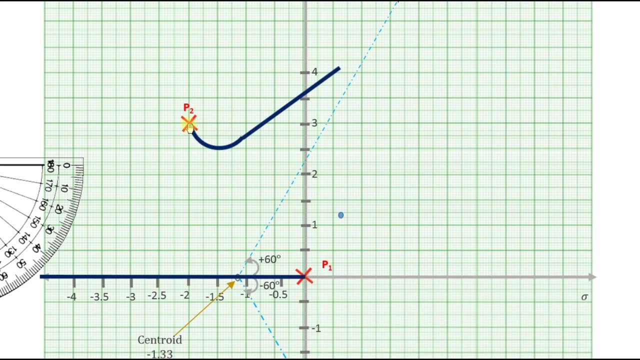 point is 3.6. okay, so here you can able to see. can able to see the pole from pole 2. see can able to see the pole from pole 2. see can able to see the pole from pole 2 itself. the root locus is. start getting. 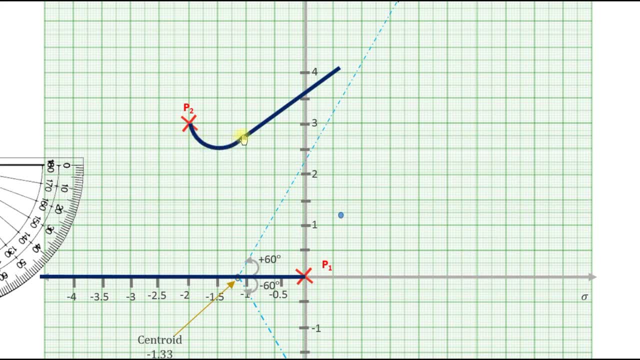 itself. the root locus is start getting itself. the root locus is start getting some diversion about minus 33.7 degree, some diversion about minus 33.7 degree, some diversion about minus 33.7 degree, and it is goes on like this and it is. 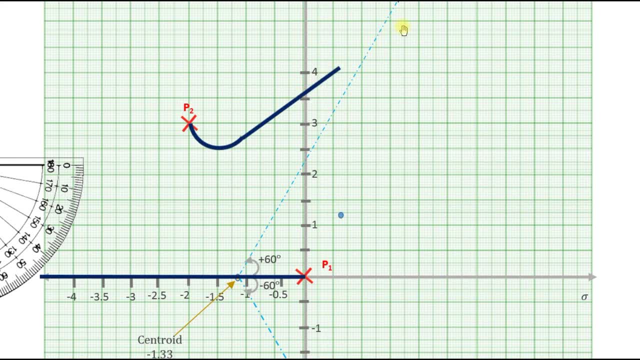 and it is goes on like this, and it is, and it is goes on like this, and it is cutting at 3.6 and goes in parallel with cutting at 3.6 and goes in parallel with cutting at 3.6 and goes in parallel with this as a total. okay, similarly in this: 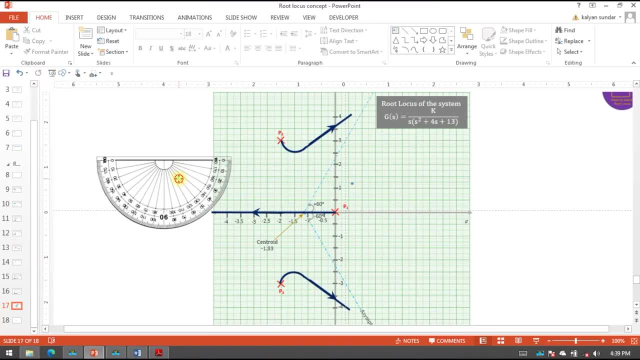 this as a total: okay. similarly in this, this as a total: okay. similarly in this pole 3. okay, in this pole 3. this is very pole 3. okay, in this pole 3. this is very pole 3. okay, in this pole 3. this is very important. okay, this is very very. 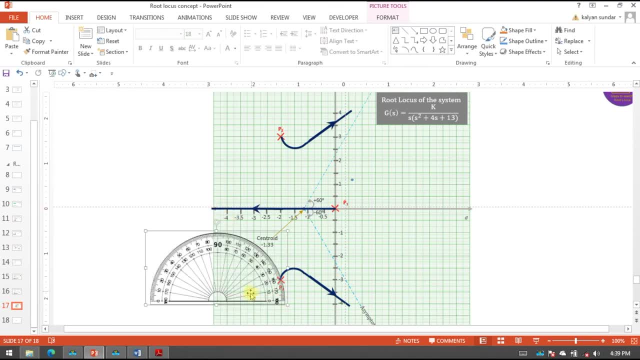 important. okay, this is very, very important. okay, this is very, very important in pole 3 itself. we are having important in pole 3 itself. we are having important in pole 3 itself. we are having the angle of departure s point sorry, the angle of departure s point sorry. 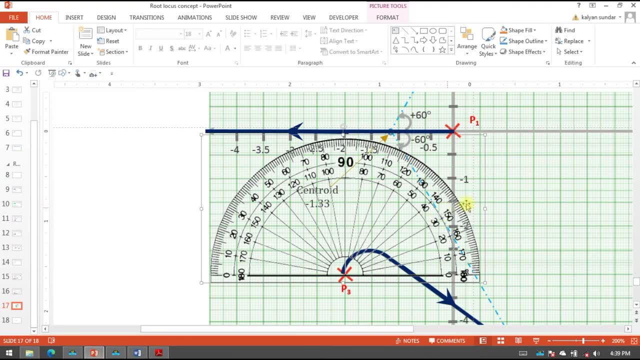 the angle of departure s point. sorry, plus 33.7 degree right. so we need to plus 33.7 degree, right, so we need to plus 33.7 degree, right. so we need to fix the line and we need to calculate the. fix the line and we need to calculate the. 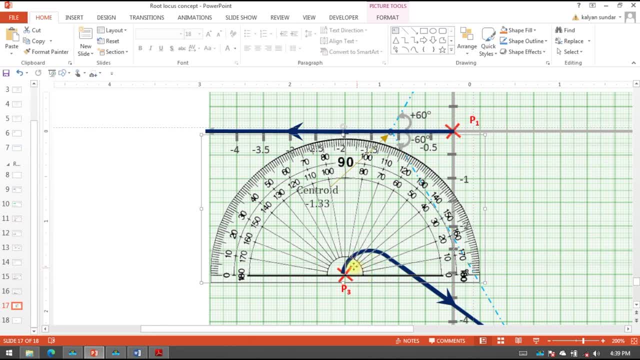 fix the line and we need to calculate the OD like this. we need to set the OD like this, we need to set the OD like this, we need to set the protector like this and I need to protector like this and I need to protector like this and I need to coincide with this point. okay, 33 degree. 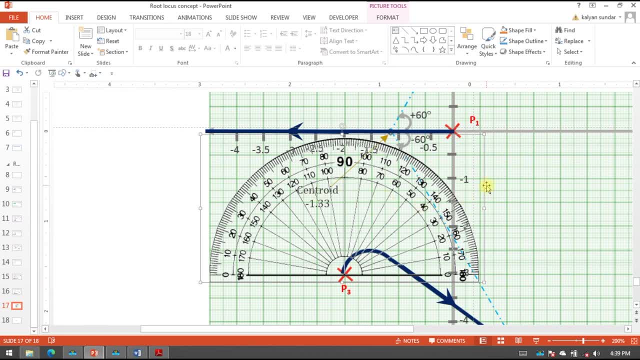 coincide with this point. okay, 33 degree coincide with this point. okay, 33 degree itself. 33.7 degree- is there that nearly itself. 33.7 degree: is there that nearly itself? 33.7 degree- is there that nearly 34? all right, so here we need to take. 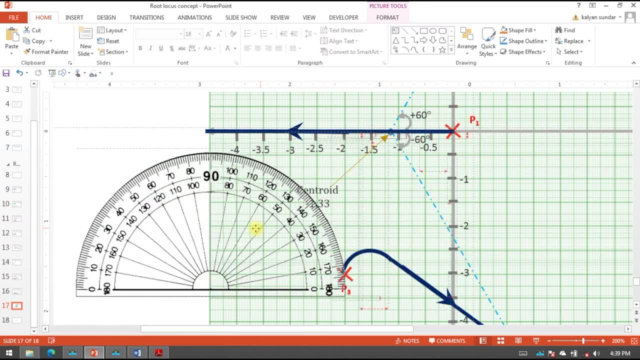 34. all right. so here we need to take 34, all right. so here we need to take this kind of diversion with the 33.7, this kind of diversion with the 33.7, this kind of diversion with the 33.7 degree. and also the crossing point is: 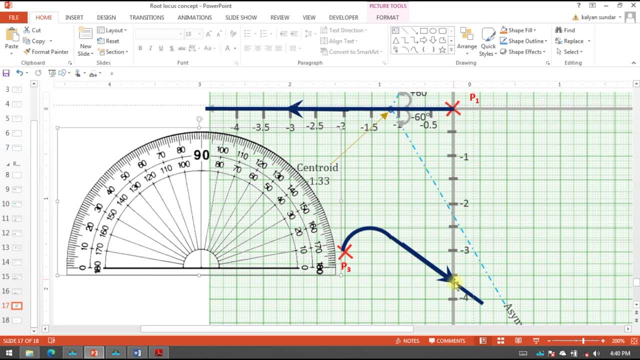 degree, and also the crossing point is degree and also the crossing point is plus or minus 3.6. so here also at plus or minus 3.6. so here also at plus or minus 3.6. so here also at exactly at 3.6 point. imaginary axis. 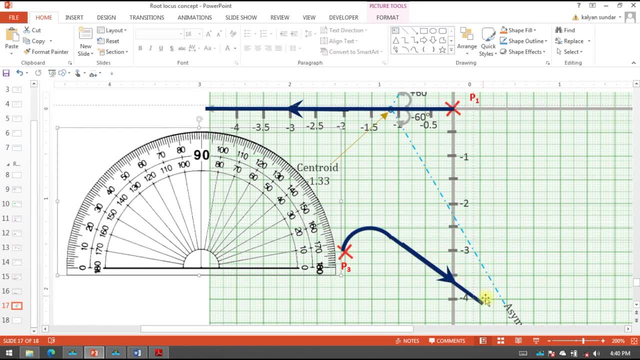 exactly at 3.6 point imaginary axis. exactly at 3.6 point imaginary axis. value: the root locus is crossing and it value the root locus is crossing and it value the root locus is crossing and it is going in parallel with the asymptote, is going in parallel with the asymptote. 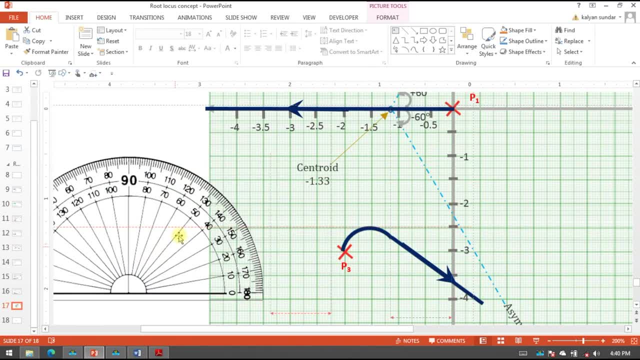 is going in parallel with the asymptote 2. okay, so this is the root locus diagram 2. okay, so this is the root locus diagram 2. okay, so this is the root locus diagram for the given system. please wait are for the given system. please wait are. 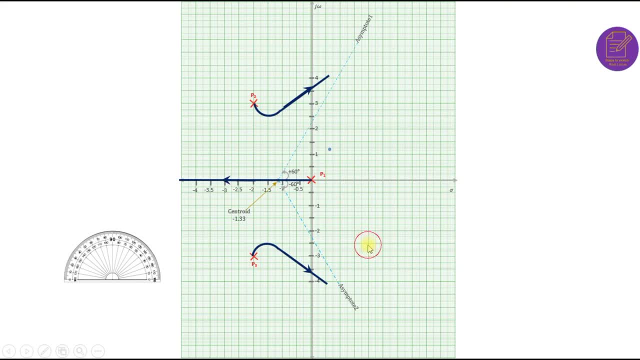 for the given system, please wait. are able to understand. okay. so, the able to understand. okay. so the able to understand, okay. so the direction wise, the location of the closed direction wise, the location of the closed direction wise, the location of the closed loopholes made available in this entire. 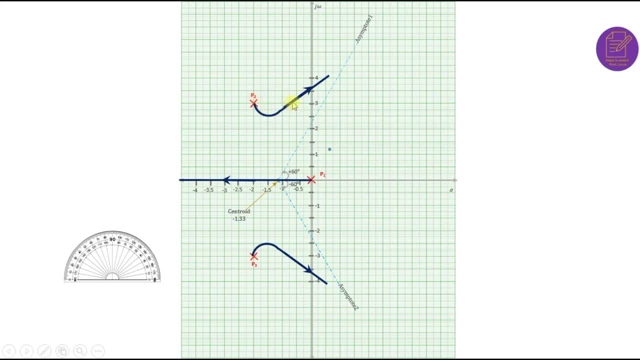 loopholes made available in this entire loopholes made available in this entire negative real axis or otherwise. there- negative real axis or otherwise there- negative real axis or otherwise, there may be a. there may be a locus like this may be a. there may be a locus like this: 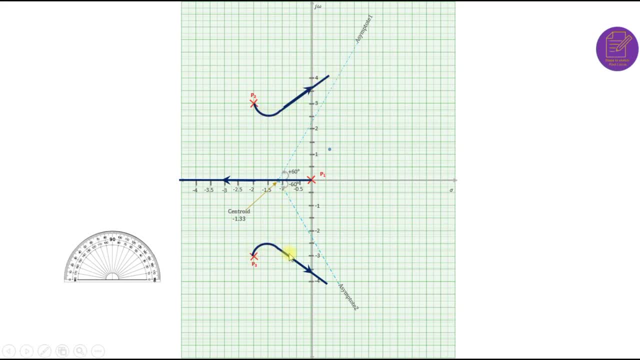 may be a. there may be a locus like this: in for second quadrant and also in in for second quadrant and also in in for second quadrant and also in third quarter and also there may be a third quarter and also there may be a third quarter and also there may be a what there may be a. 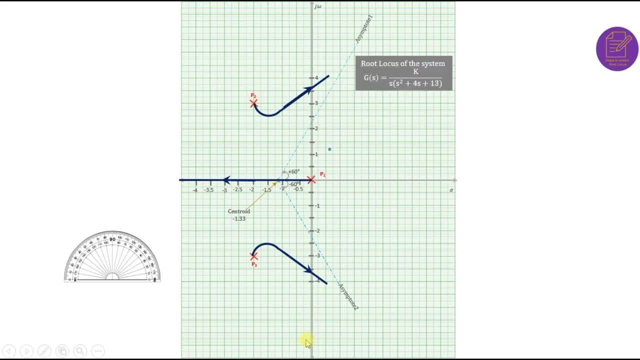 what there may be a what there may be a pole location like this: okay, so this is pole location like this. okay, so this is pole location like this: okay, so this is the entire root locus of the. given the entire root locus of the. given the entire root locus of the given system, k, divided by s into s square plus. 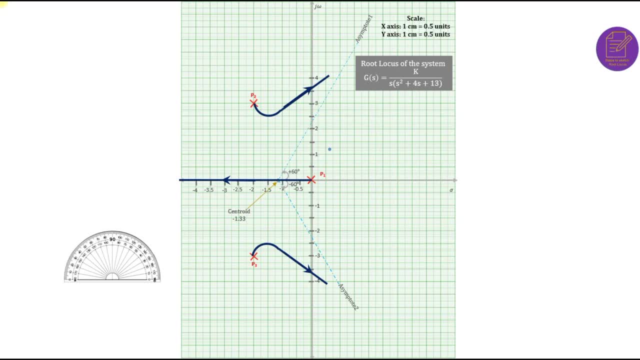 system k divided by s into s square, plus system k divided by s into s square, plus 4s plus 13, and 4s plus 13 and 4s plus 13. and we know that we only with the information. we know that we only with the information. 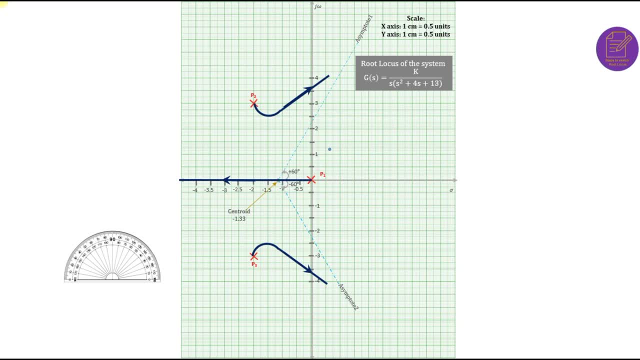 we know that we only with the information about open loop poles and zeros. we are about open loop poles and zeros. we are about open loop poles and zeros. we are calculated the locations of the closed. calculated the locations of the closed. calculated the locations of the closed loopholes. okay, in order to meet out the 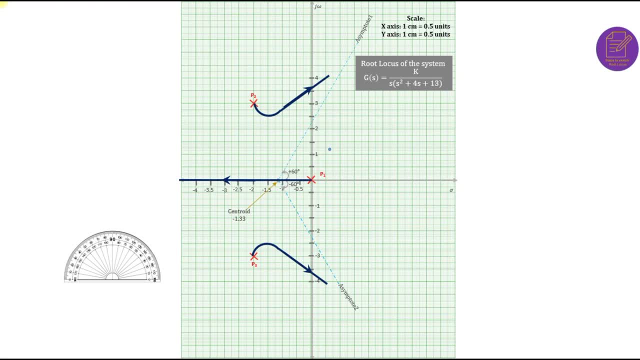 loopholes. okay in order to meet out the loopholes. okay, in order to meet out the. in order to the system should meet the. in order to the system should meet the. in order to the system should meet the stability. okay for the various values of stability. okay for the various values of. 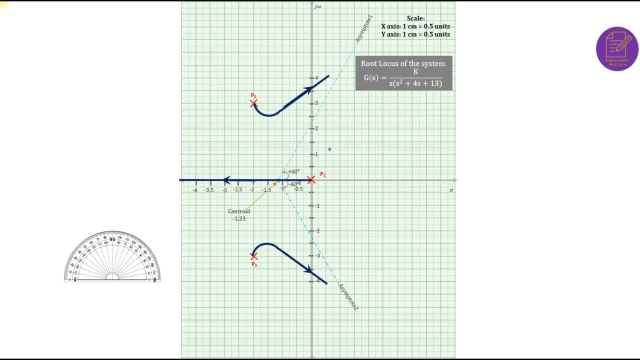 stability. okay, for the various values of k also. it is also possible to find out k also. it is also possible to find out k also. it is also possible to find out the locations of the closed loopholes: the locations of the closed loopholes, the locations of the closed loopholes. okay, so this is the simple procedure for. 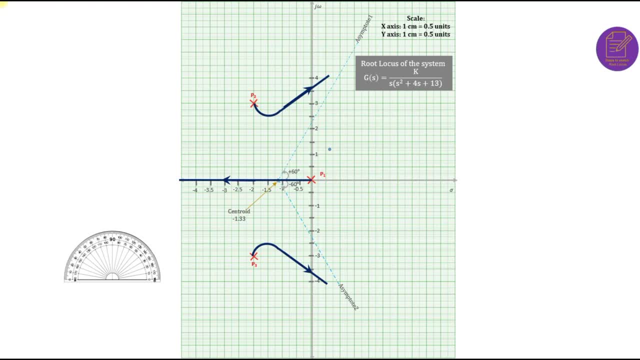 okay, so this is the simple procedure for okay. so this is the simple procedure for finding out the root locus of the given. finding out the root locus of the given. finding out the root locus of the given system. this is model one- okay, two, or system. this is model one, okay, two, or. 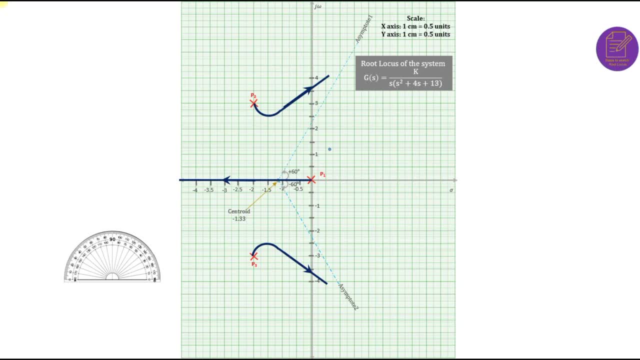 system. this is model one. okay, two or three models are there. kindly watch the three models. are there? kindly watch the three models. are there? kindly watch the next upcoming videos also where we will next upcoming videos, also where we will next upcoming videos also where we will solve different kind of root locus. 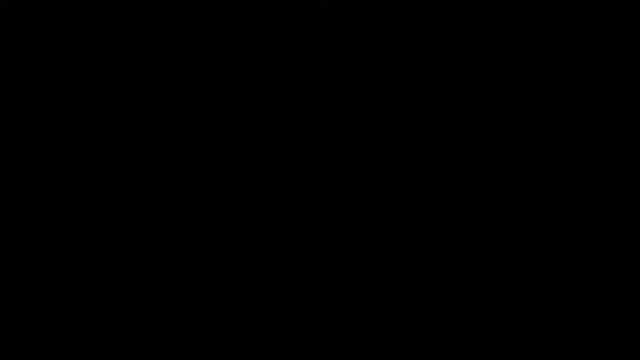 solve different kind of root locus. solve different kind of root locus problems. okay, thank you. 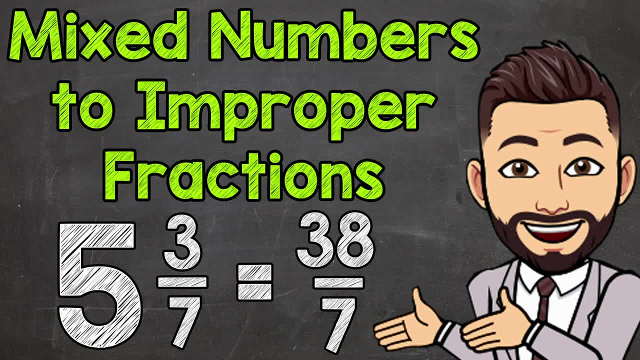 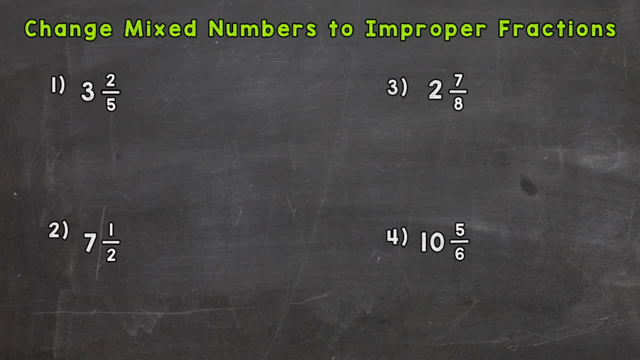 Welcome to Math with Mr J. In this video we're going to take a look at how to change mixed numbers to improper fractions And, as you can see, there are four problems, four mixed numbers on your screen there. We're going to change each of those to their equivalent improper fraction. So let's jump right in. 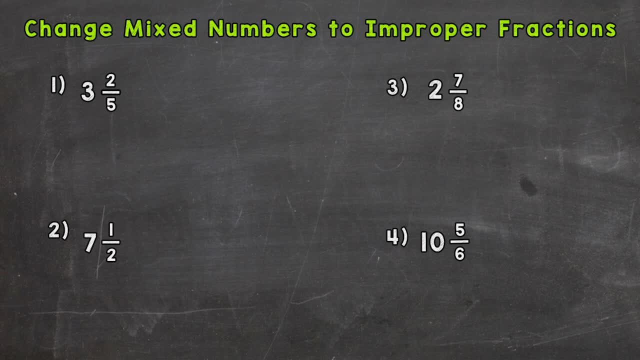 to number one And we have three and two fifths here for number one. So we're going to change that again to its improper fraction. So what we need to do, I call it the C method. We're going to start at the bottom here and we're going to come around. We're going to multiply the denominator.